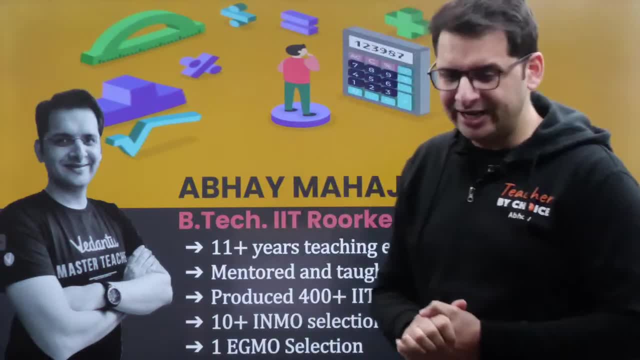 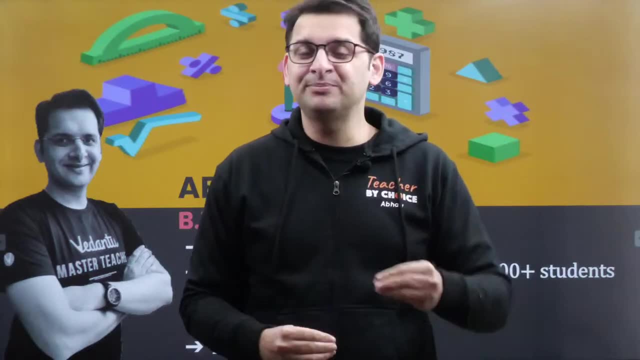 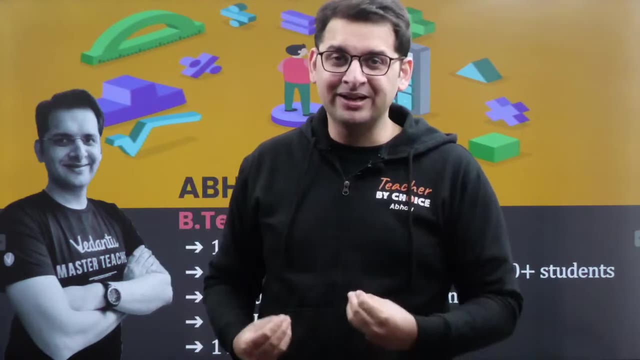 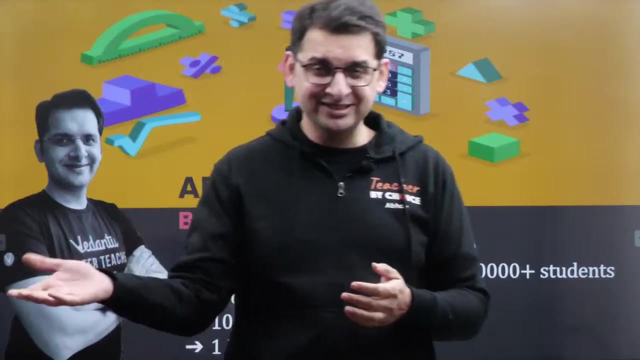 yes, IMOTC has been cancelled and so we can't do anything. this is something which is not there in our hands. we can only do preparation as per ourselves. we can only do good preparation. we can try to make it a little bit, which we are doing. we are doing it on YouTube, we are doing it on Vedantu platform, we are doing it in IEOQM camp, 7 day a week. engagement is already going on and marathon sessions are also being planned for INMO. so this is what we all can do. we can all work hard from now on. 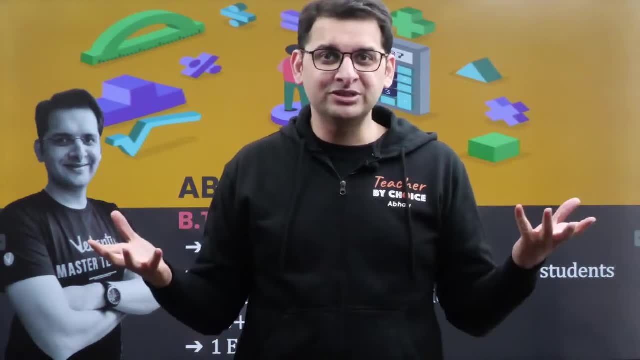 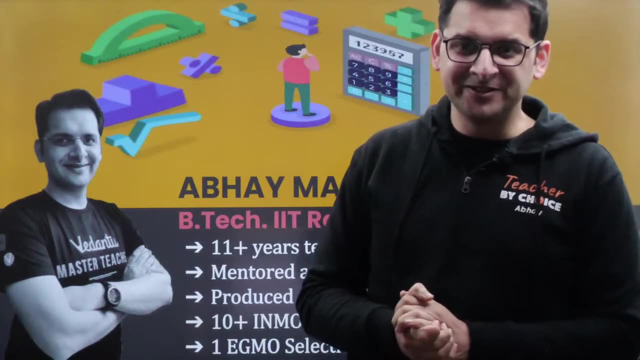 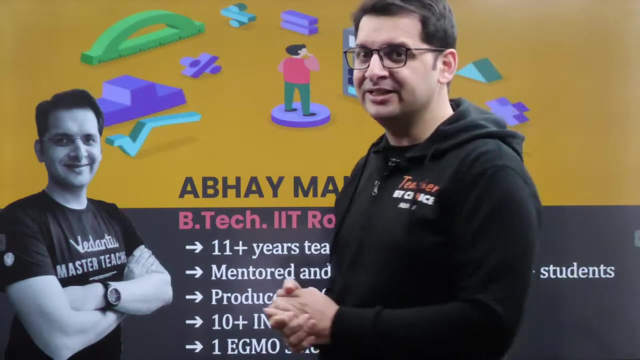 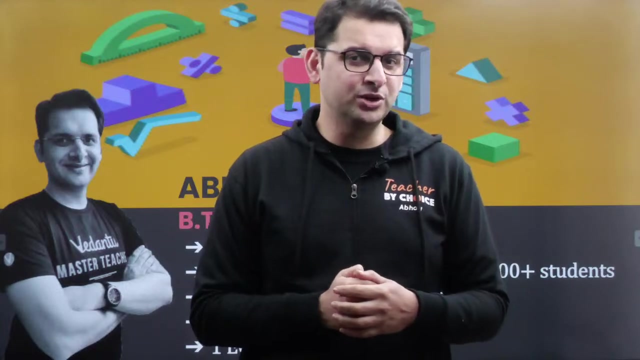 our side and that is what we are doing. so again, whatever is not in our hands, guys, there is no point in discussing it. yes, previous year kids will also be there. yeah, yeah, yeah, kids. so almost basically almost 400, 450, 500 copies will be checked, basically 30 regions if we assume India, which has been divided so in 30, 10 plus 2 plus 2, so all 420 copies will be given and 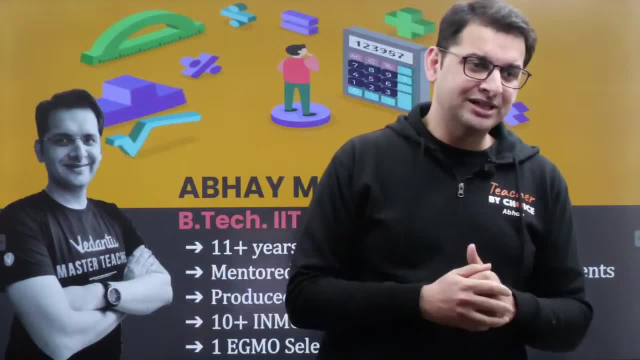 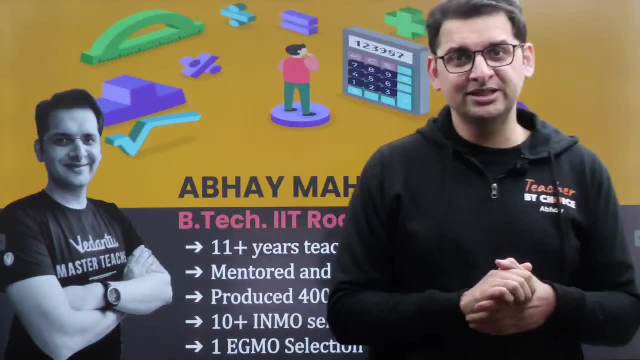 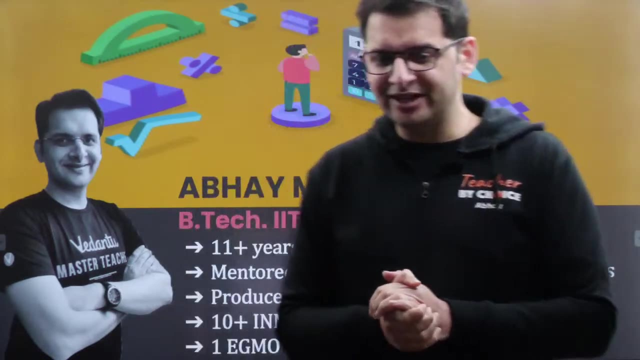 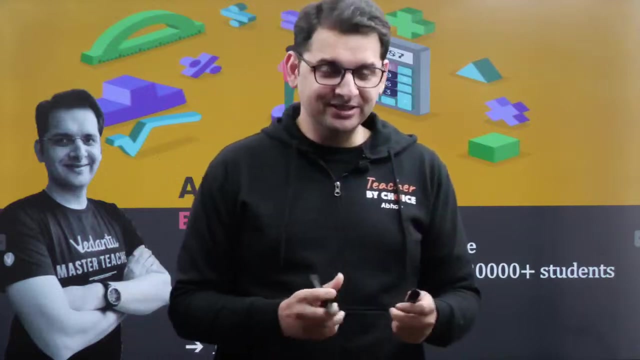 in 80,, 100, 20, previous year kids, which is again only their part B scores- will be checked irrespective of their part A scores. so almost 500, 520 copies will be checked. out of them, 6 kids will be slated. who will represent India directly? yes, yes, Pranjal is also giving guys. Pranjal is in 12th, so Pranjal is your competition. Pranjal is in 12th right now, so Pranjal will also be giving the exam. okay, so, of course, and we 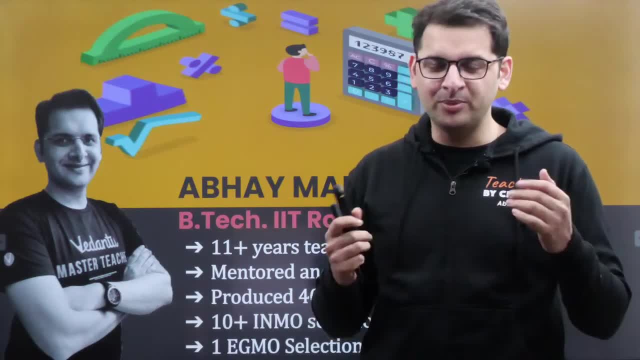 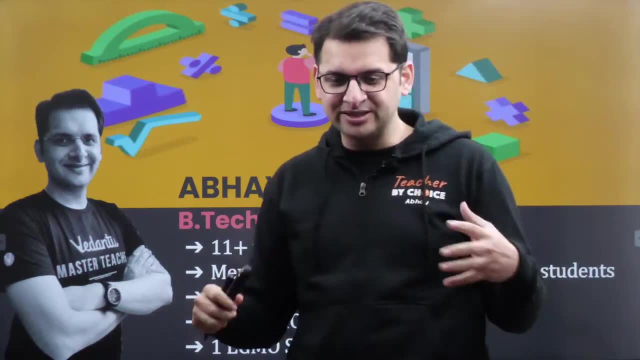 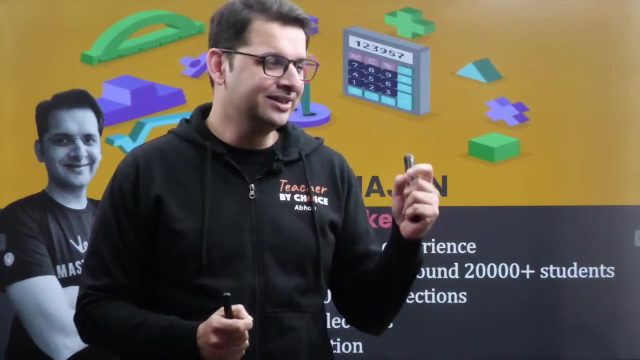 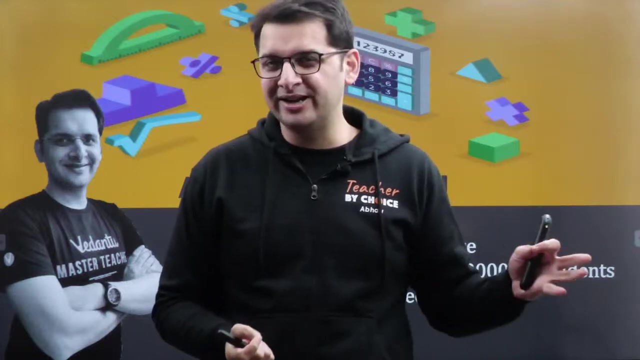 need Pranjal in our team. so again, Pranjal, just the way he has been performing for the last 2-3 years, bringing gold for the country. so again, I am very sure that this year the level which is going to happen with Pranjal and others in the team it is going to be super high and one of- maybe some of you can also join him in the team. just work hard, simple thing: 25 days, 20 days, 25 days, whatever is left- okay, almost 20 days are left. so work hard, really hard, and whatever things we need we are ready to give you. camp is already going on life. 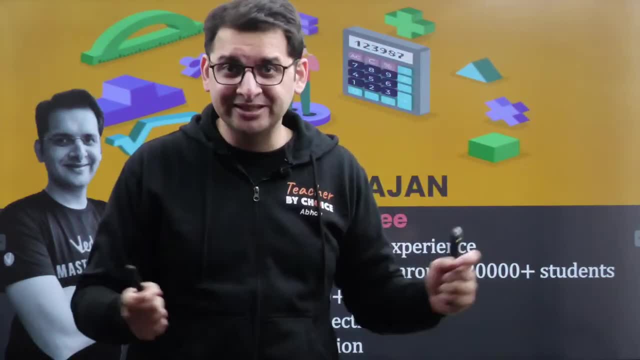 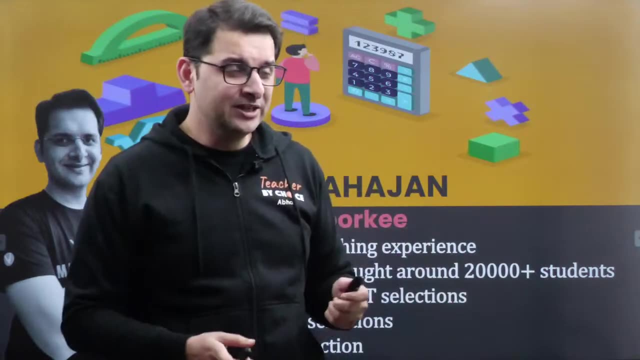 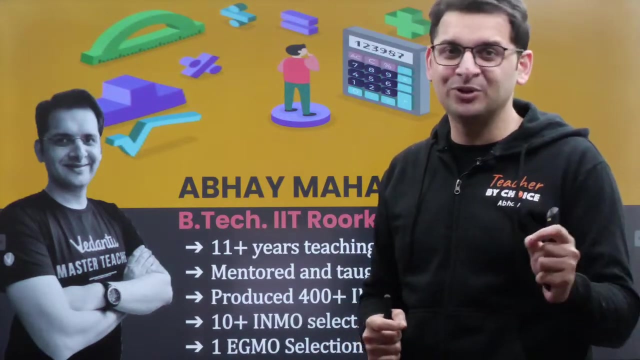 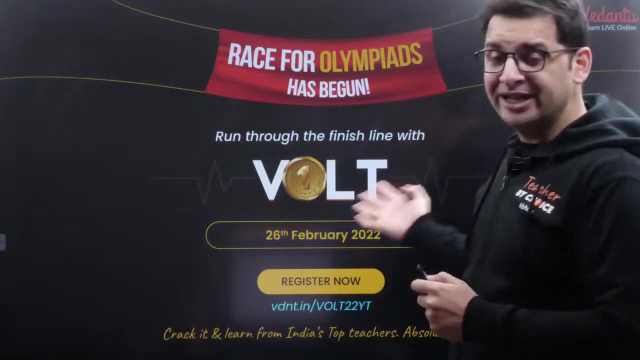 classes are going on on YouTube. life classes are going on on camp. you can also watch it in recorded form. books we have given to many children on Telegram. if you still need books, you can get in touch with us over Telegram. so whatever help can be done, we are ready to do it. just you read with passion. that is the only thing. got it, let's go, let's go. alright, guys, so start. so Wolt's exam, guys, is happening. so this is for the students who are in our batches: go, go, go, guys. 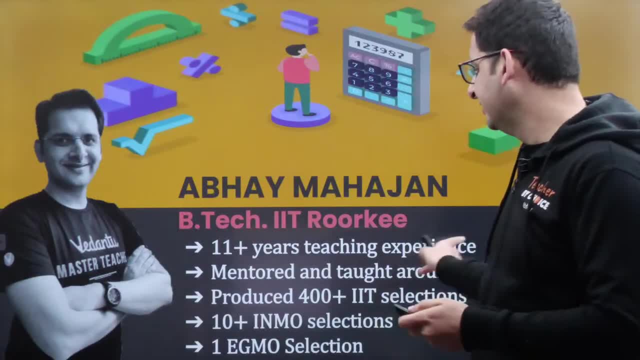 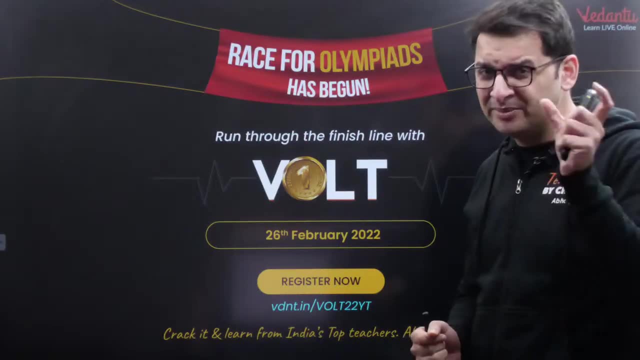 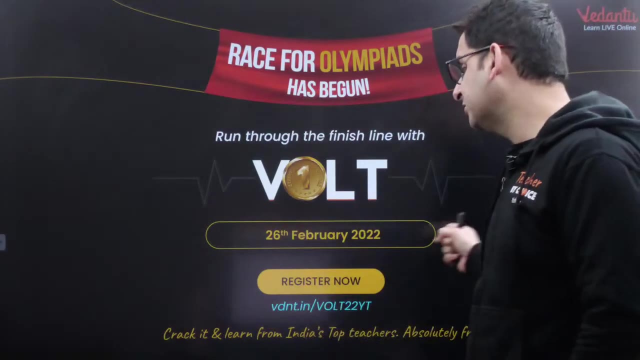 If you want to take admission for the first year, then you have to go to vdntincom register yourself. you will get a message from us, you will get a link. there will be a separate paper for maths courses. there will be a separate paper for junior science. there will be a separate paper. for SOF: there will be a separate paper. so this is something that you need to attempt. 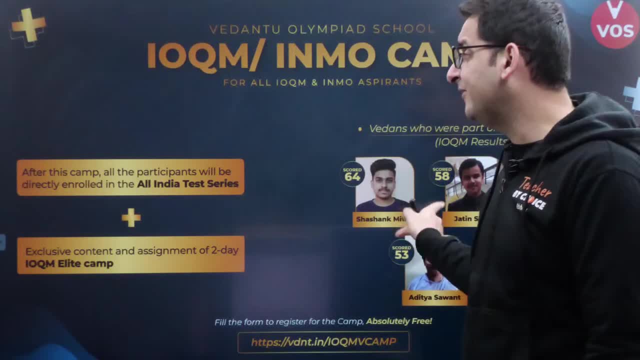 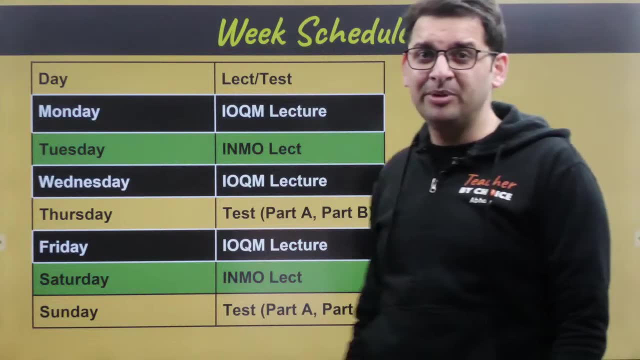 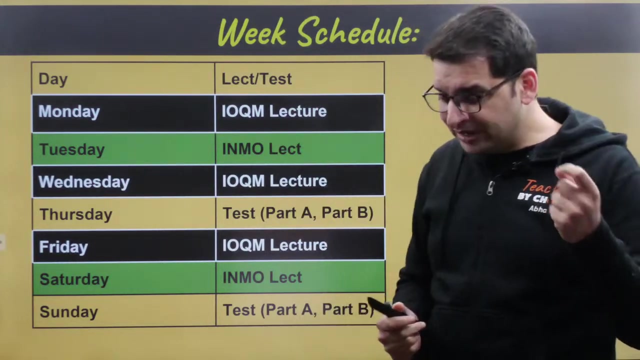 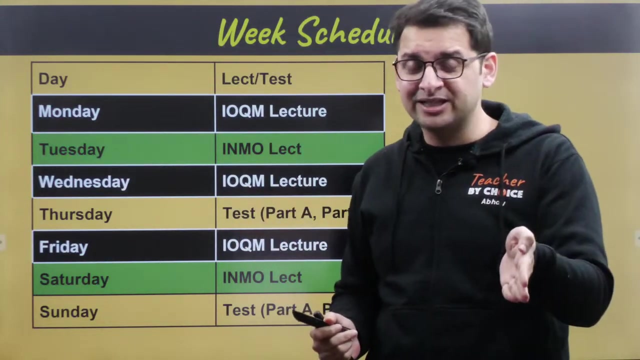 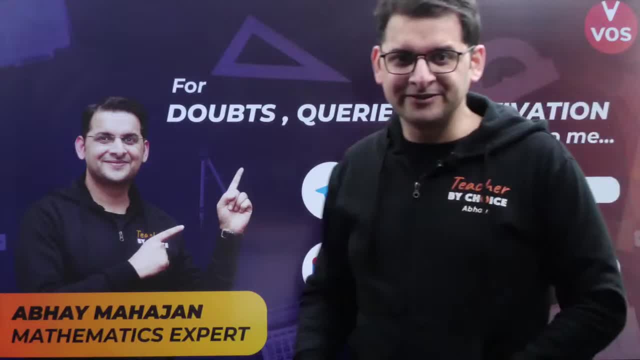 And in the last year you wrote INMO. or now all your tests are going on. we show the children in the live class that we are going to check the copies of these children or are doing it Super, super Amazing. So this is my Telegram: ع aged86Mahajan. you can get into touch with me over Telegram. 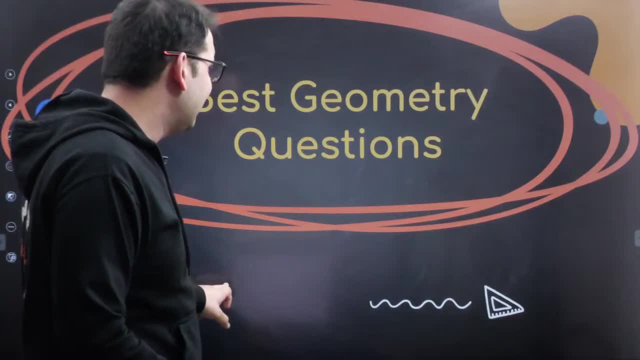 and now we will begin best: geometry questions, Although we have mentioned this name, but today we are going to discuss, but today we are going to discuss, but today the grade of the questions that we are going to discuss is for very, very cute kinds of questions. 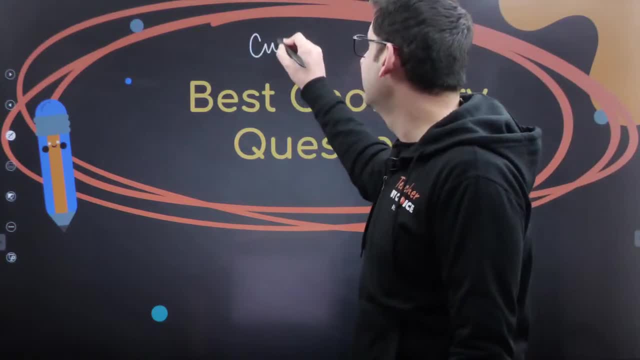 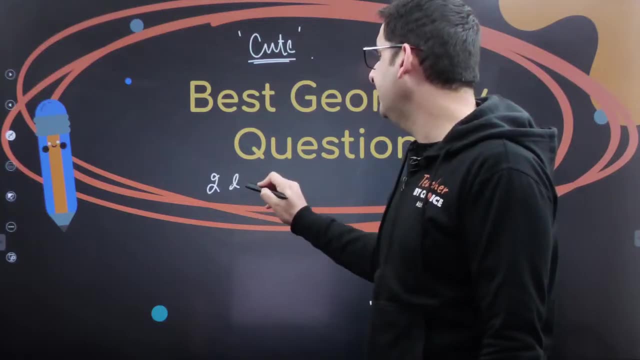 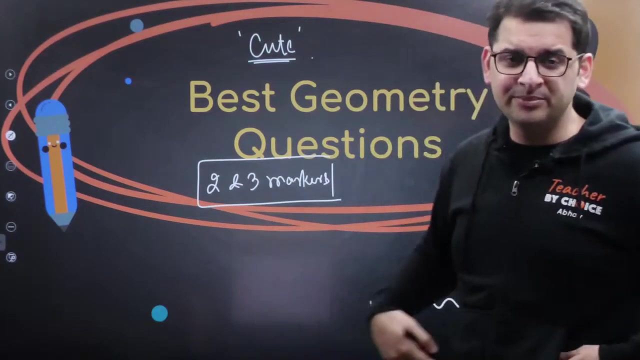 but today the grade of the questions that we are going to discuss is for very, very cute kinds of questions. So basically, majorly we will be discussing 2 and 3 marker questions. so 2 marker and 3 marker because the 5 number questions. 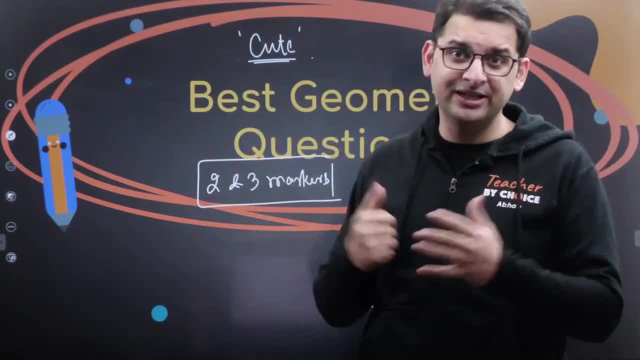 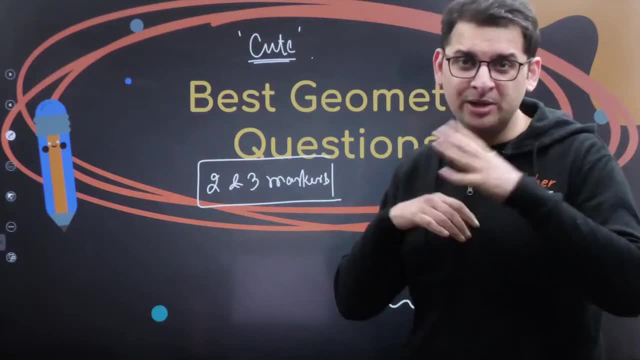 and inmo level content. we did a lot last week and a lot of kids were saying, sir, please bring some sessions for IOCUM. so again this week it is on the basis of IOCUM. so today's session is 2, 3 marker. number 3 session is 3 to 5 marker. 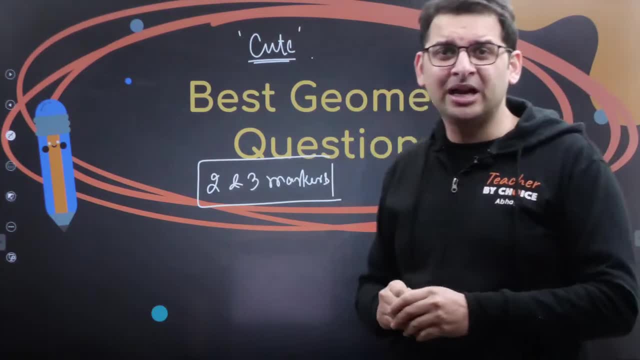 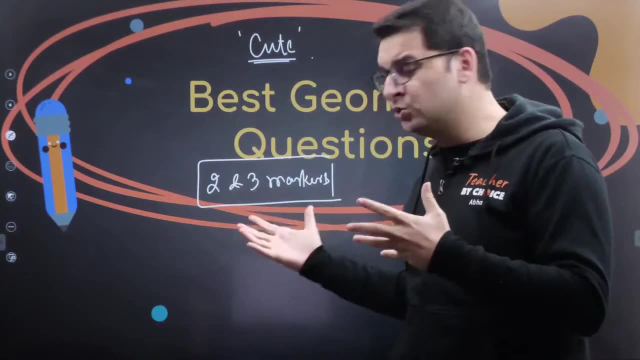 so it will depend. so we have done a lot of good questions already. geometry gems series is going on, in which we have done a lot of good 5 number questions. so again, its practice too. 2 number, 3 number questions, basic questions, practice. you should know how to see, you should know how to understand. 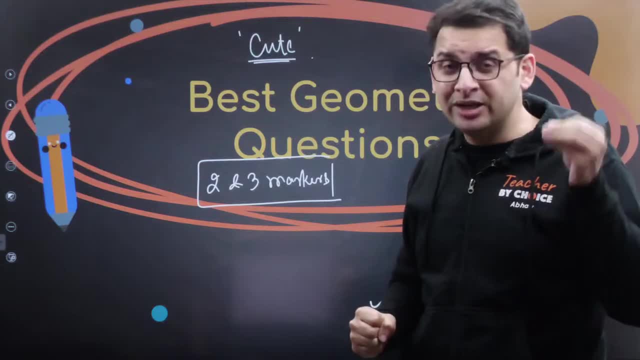 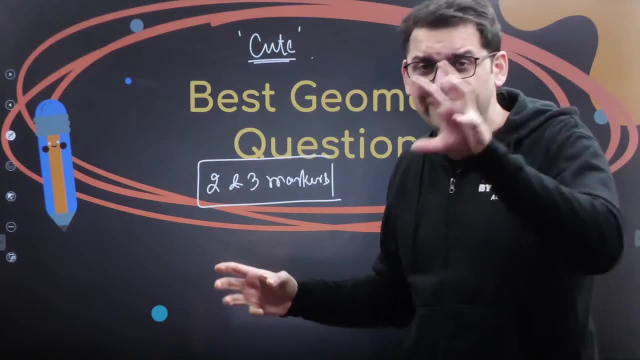 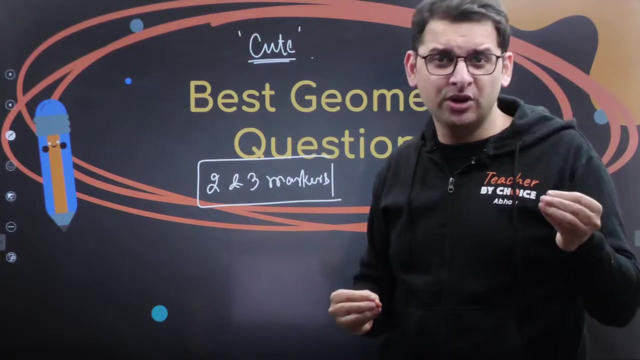 you should strike ideas which not only you know 2 number questions directly help, but 5 number questions also have small concepts which after taking out you have to use it and somewhere else you have to see it. so again, very basic concepts, very small concepts, you can do it. 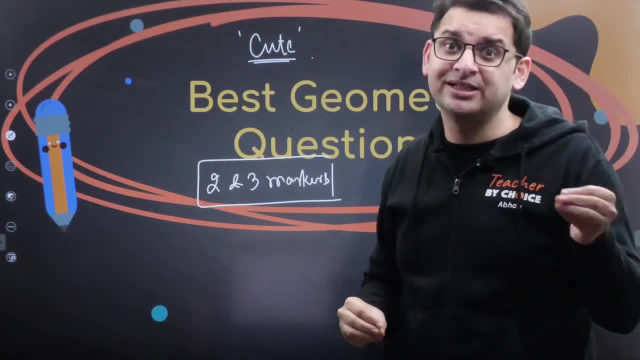 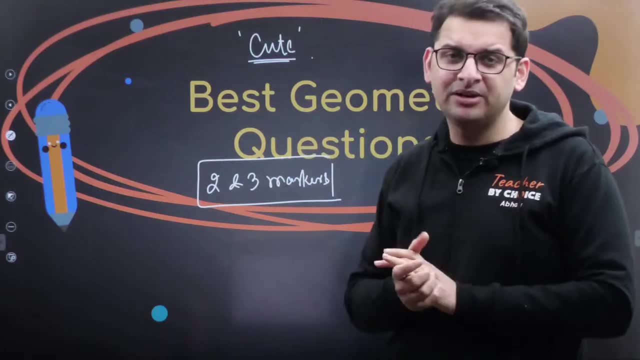 which should strike you as soon as you see it. so that kind of a session. it is going to be very quick session. 7-8 questions are going to be discussed. last 2 questions are very good. I will talk about 3 number questions. rest all are very simple. 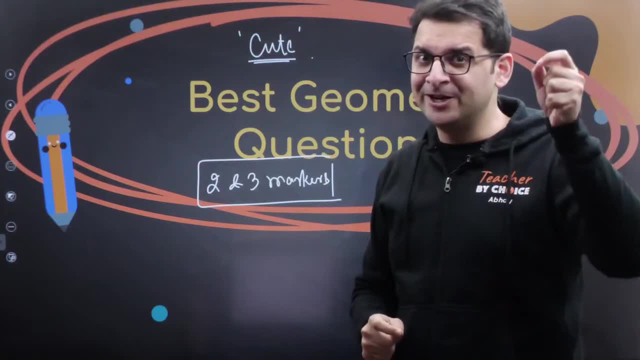 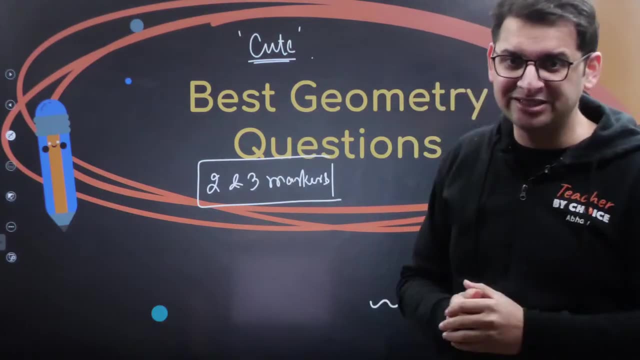 very basic questions and the expectation from you people is you should be able to write the answer on the chat box before I write the answer. as simple as that. if you are ready for this, give me a thumbs up on the chat box if you are ready for this. 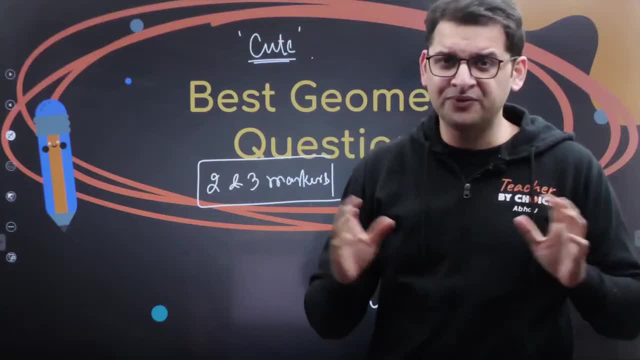 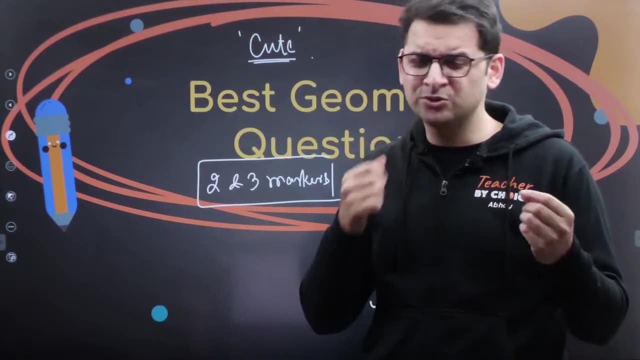 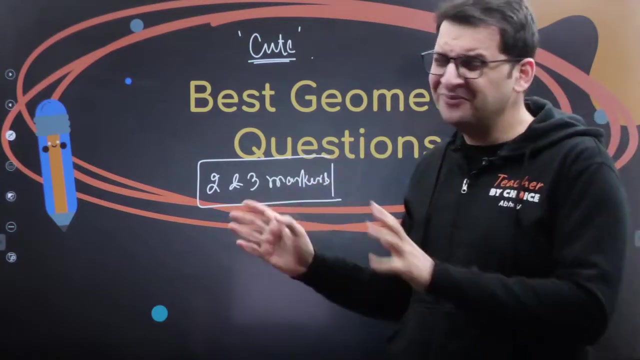 Arav your wish. if you think that you are confident, you don't need to attend this lecture live. you can see it later on your page and the questions: just see it later. ok, but today's session is going to be very simple. very mostly it is going to be 2 marker. 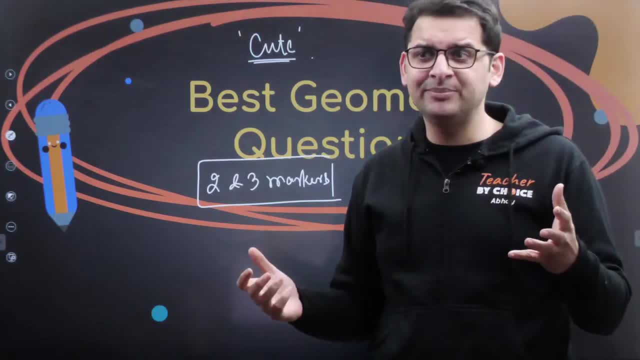 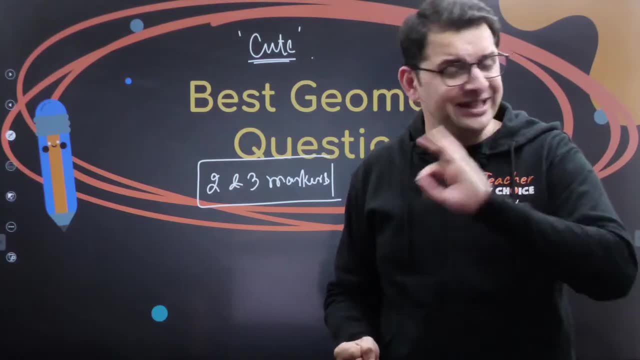 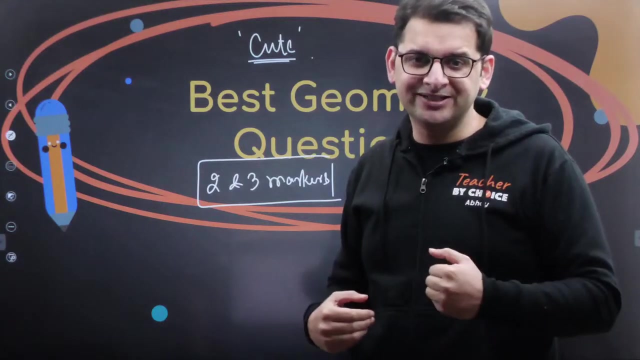 and very simple questions, very simple questions. all the questions are not made by me, all the questions are taken from a mathematics competition. ok, so it is that kind of session, but they are very simple questions and mostly questions are very quick, in one or two lines only. so that kind of session it is. 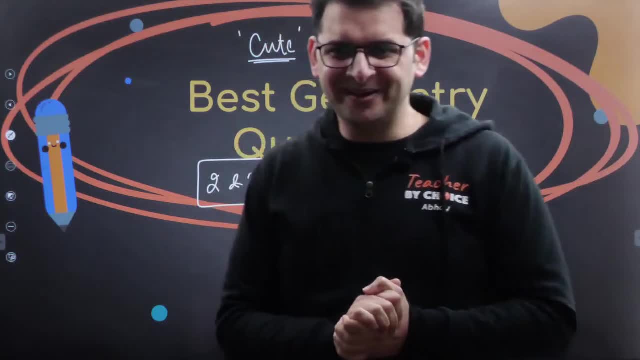 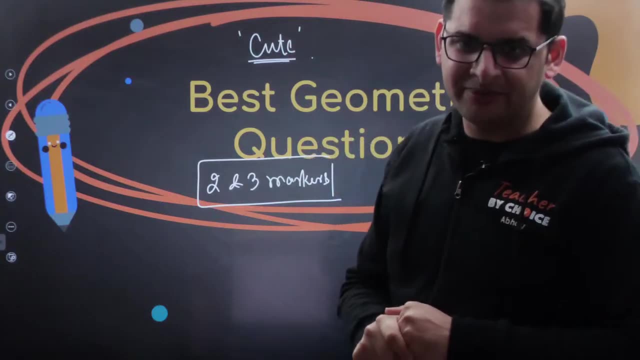 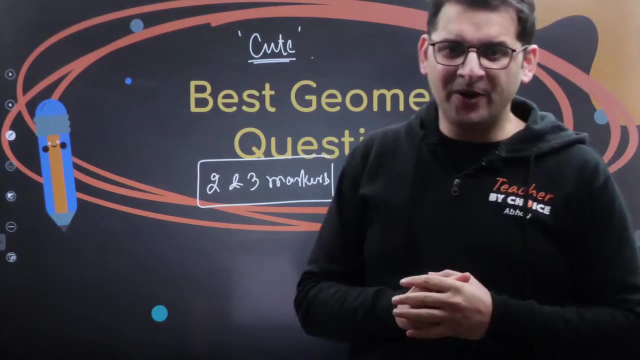 yes, yes, it is exactly a moral booster. amazing, amazing. ok, someone from Bangladesh is saying: I can't participate in world. ok, I will talk to my team about this, that why Bangladesh is not there. I will talk to my team about this, don't worry about it, all right? 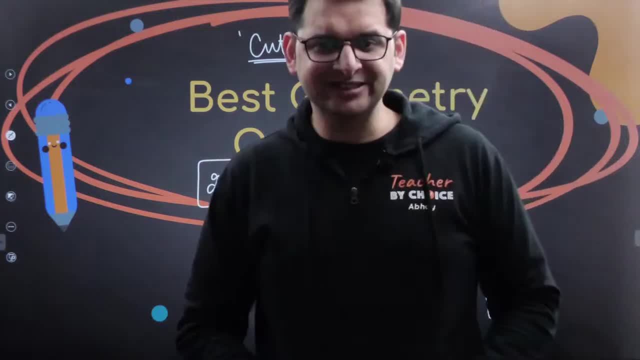 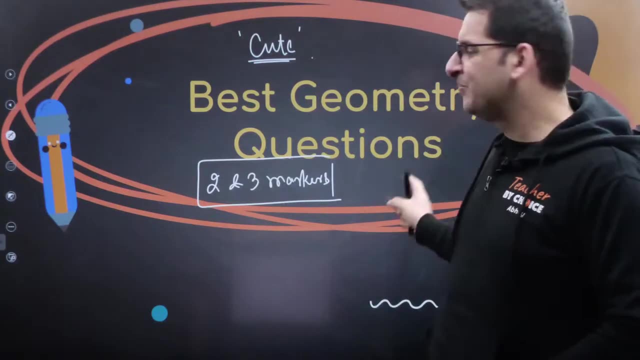 all right, so start guys. yes, yes, yes. 8th grader, 9th grader, 10th grader, 11th, 12th- all the graders can do this. questions all right? ok, all right, so let's start. let's start today's session. 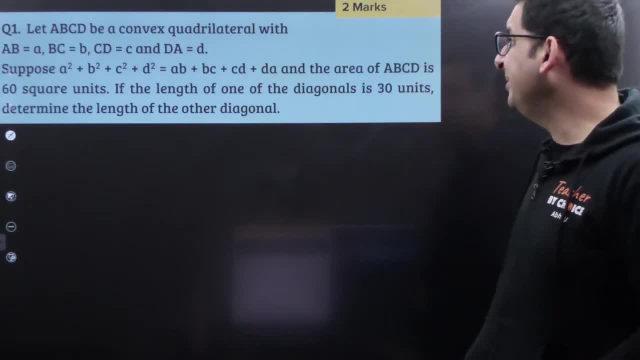 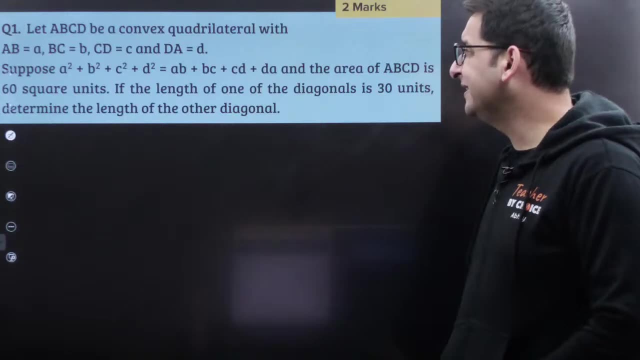 today's session. this is the first question. guys, let A, B, C, D be a convex quad with A: B is equal to A, B, C is equal to B, C, D is equal to C and D A is equal to D. suppose A square plus B square plus C square plus D square is. 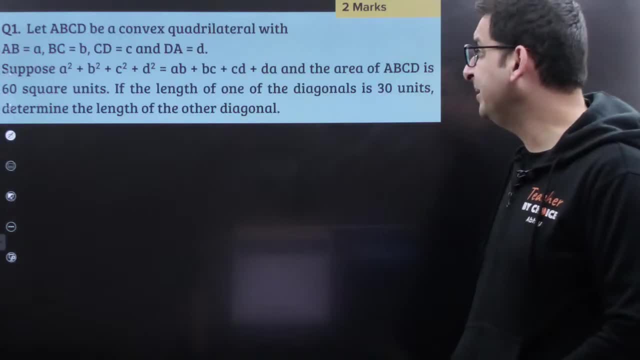 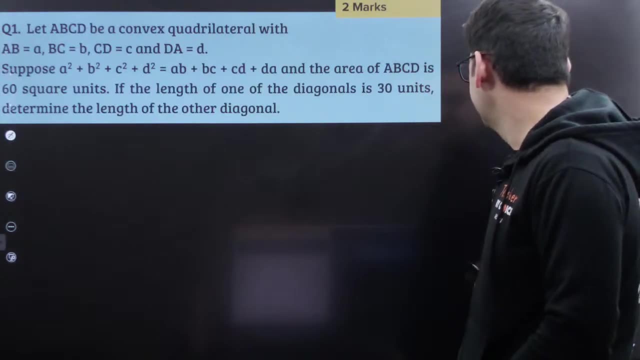 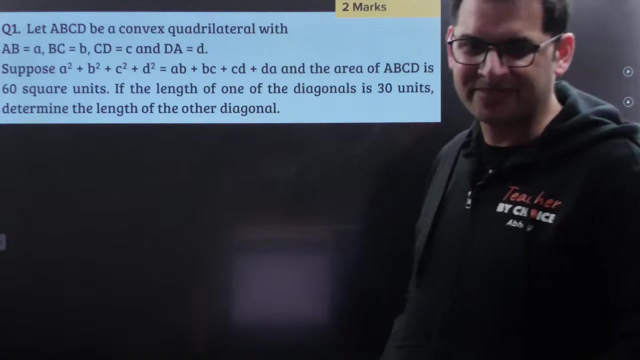 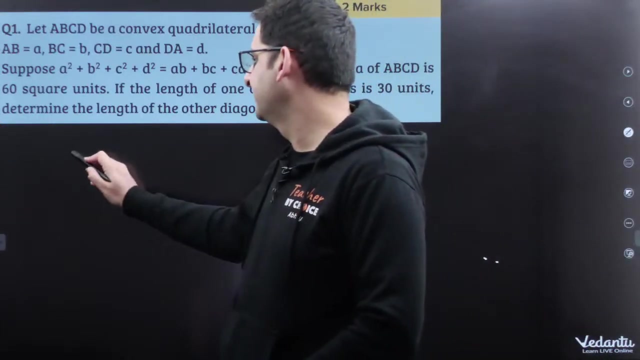 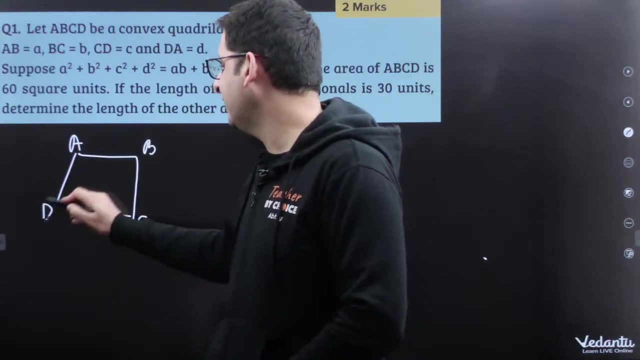 A, B plus B, C plus C, D plus D, A and area of A, B, C, D is 60 square units. length of one of the diagonals is 30 square units. determine the length of the other diagonal quickly guys, quickly, quickly, quickly quickly. A, B, C, D is a quad. 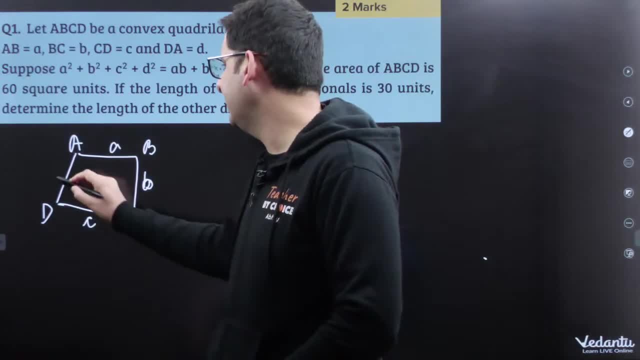 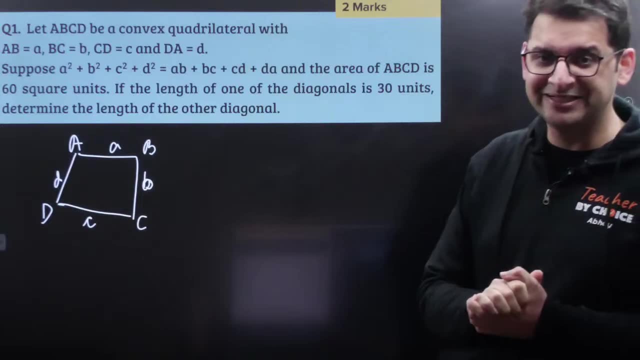 this is A, this is B, this is C and this is D. so A, B, C, D is a quadrilateral and this is given between the sides. A square plus B square plus C square plus D square is A, B plus B, C plus C, D plus D A. 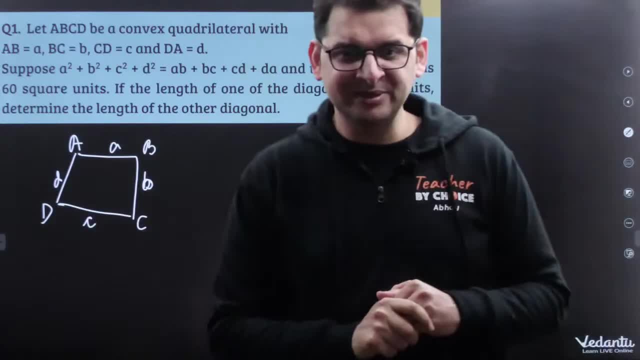 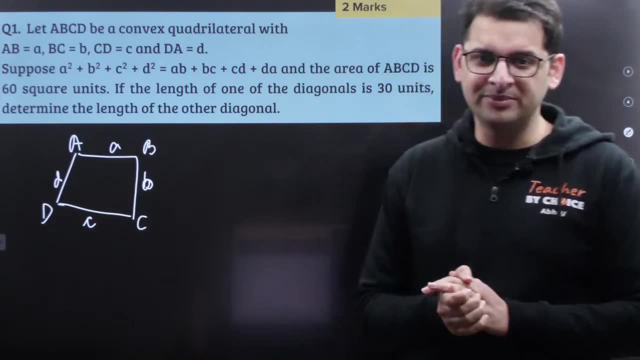 amazing. yes, yes, yes, guys, if 26 out of 41 have come, your copy will be checked, and it must have been done till now. you must have received a message, so please check your marks. you must have received a message on the mail. Tanmay is saying 4: 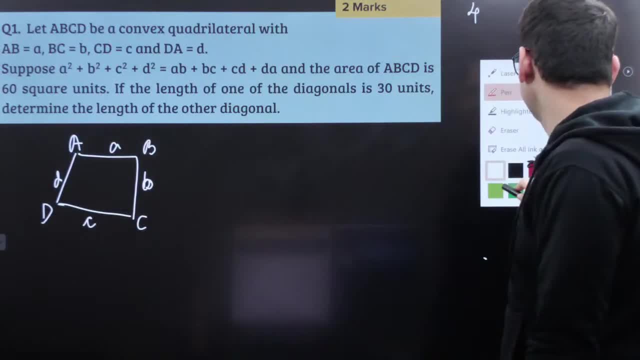 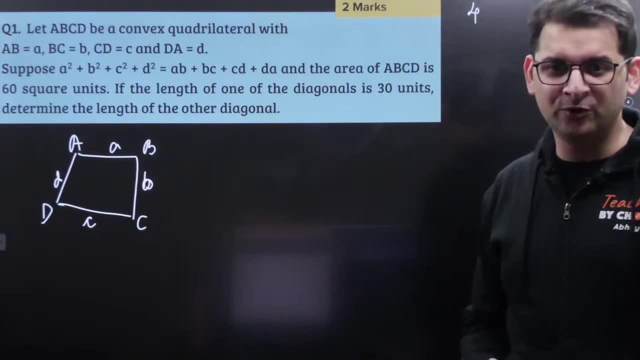 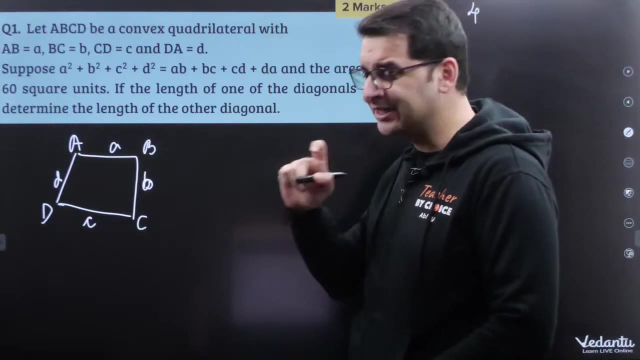 Tanmay is saying that, sir, 4 is the right answer. ok, these kind of questions are very simple. Shashwat is also saying 4. Shashwat is also saying 4, amazing, amazing, ok. so, guys, these kind of things are very simple. look, you have surely done this thing. 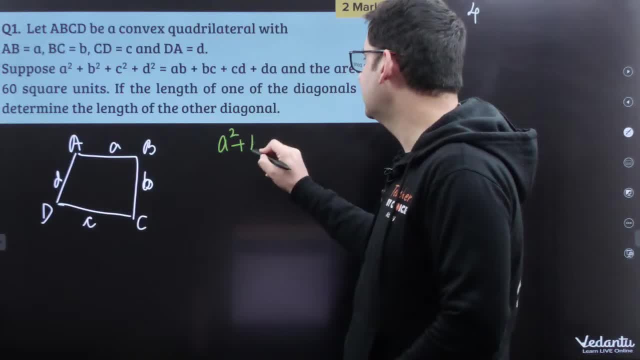 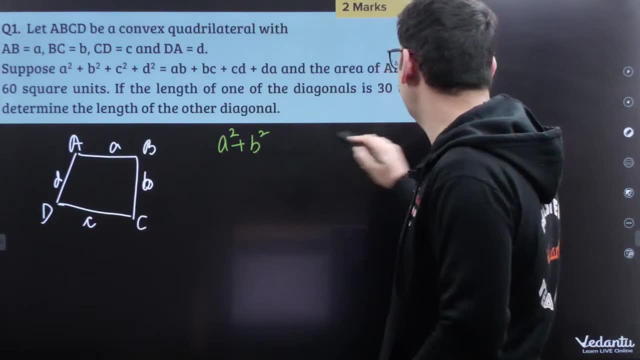 i am very sure about it, that you must have read this: A square plus B square is equal to A, B, A square plus B square. A square plus B square plus C square plus C square is equal to AB, is equal to a, b plus b, c plus c a. 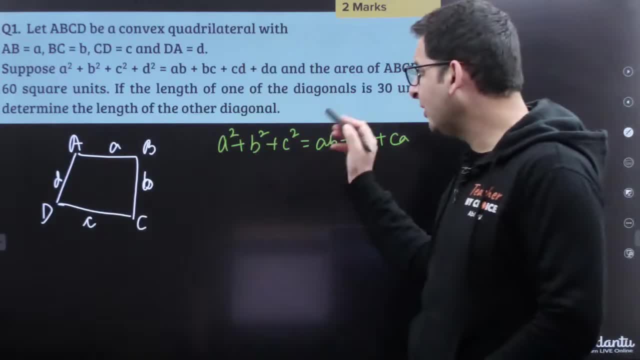 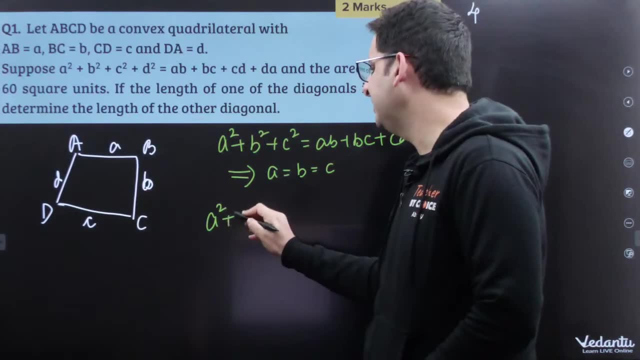 This is a very standard identity, Okay. So if this happens, then obviously what we say is: sir, a is equal to b, is equal to c, Because let's bring this here: a square plus b, square plus c, square minus a, b minus b, c minus c, a. 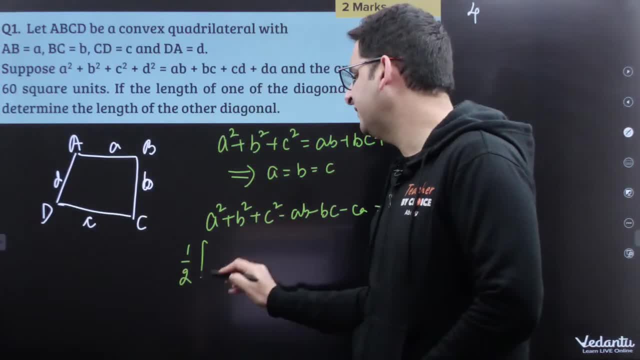 is equal to zero. Let's multiply this by 2.. Let's multiply this by 2.. Let's divide this by 2.. 2 a square plus 2 b square plus 2 c square minus 2 a b, Let's do a. 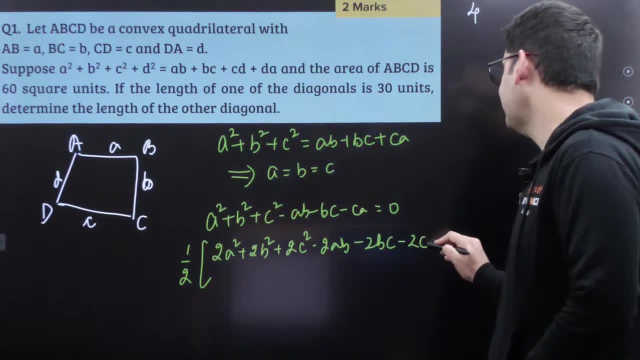 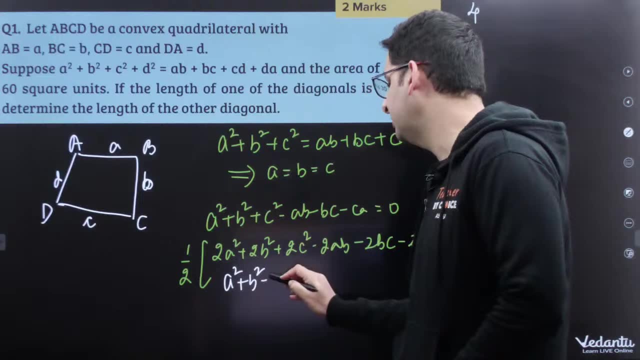 Let's do a Minus 2 b c minus 2 a c is equal to zero. And here what is done? now Let's split this: a square plus b. square minus 2 a b. b square plus c. square minus 2 b- c. 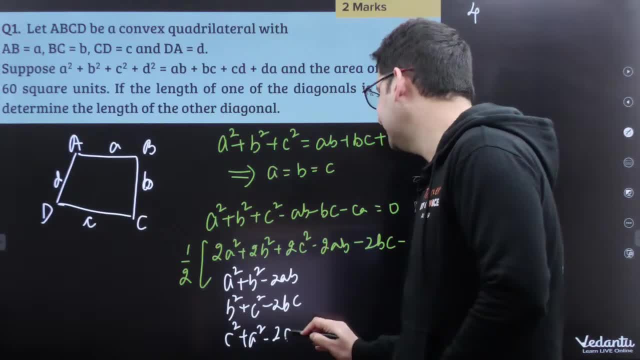 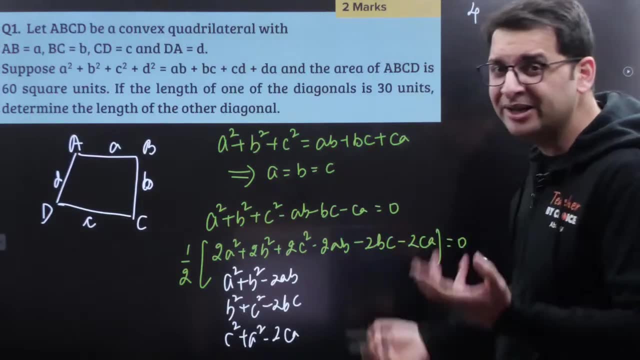 c square plus a square minus 2 c a. So this is a minus b whole square b minus c, whole square c. Exactly same thing. we will do in 4th one. Exactly same thing. So a square plus b square minus 2 a. c minus 2 a b. 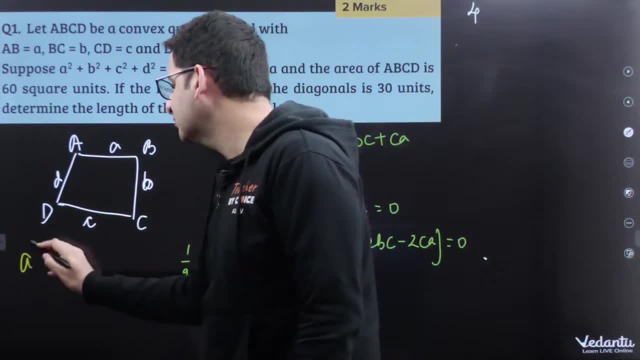 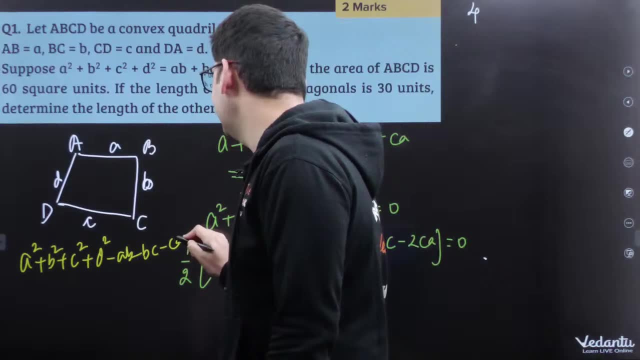 b square plus c square plus d square is equal to zero. So what is done now? a square plus b square plus c square plus d square minus a, b minus b, c minus c, a, c, d minus d, a is equal to zero. Multiply by 2 and divide by 2.. 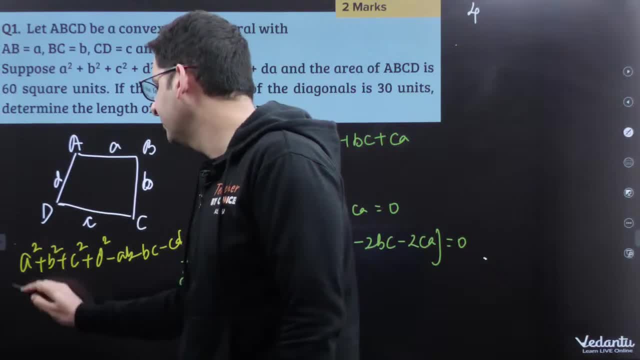 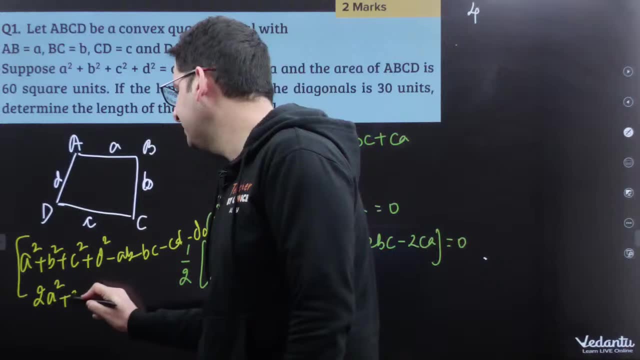 Multiply by 2 and divide by 2.. So multiply this whole by 2 and divide by 2.. So what will happen here? 2 a square plus 2 b square plus 2 c square plus 2 d square. 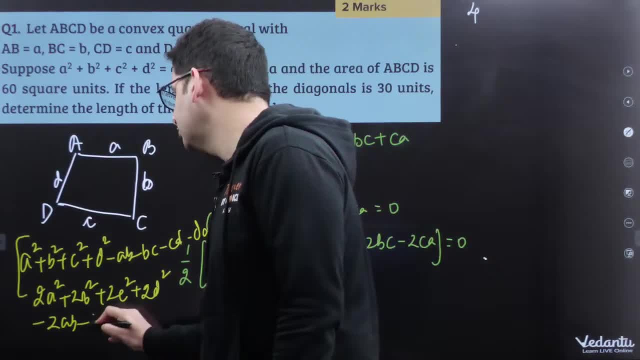 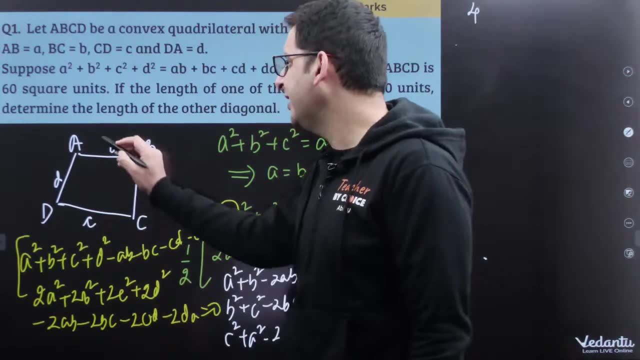 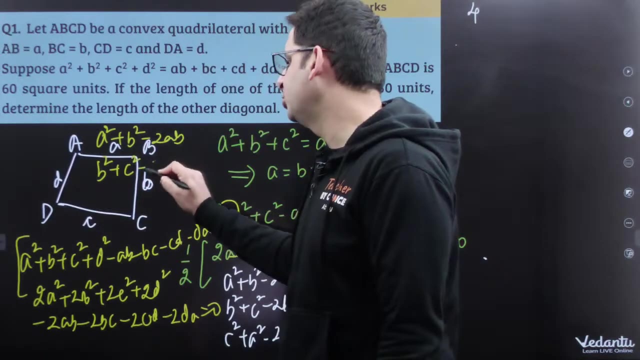 So what will happen here? minus 2 b c, minus 2 b c, minus 2 c d, minus 2 d a, This is zero. So now we have split A square plus b square minus 2 a b b square plus c square minus 2 b c. 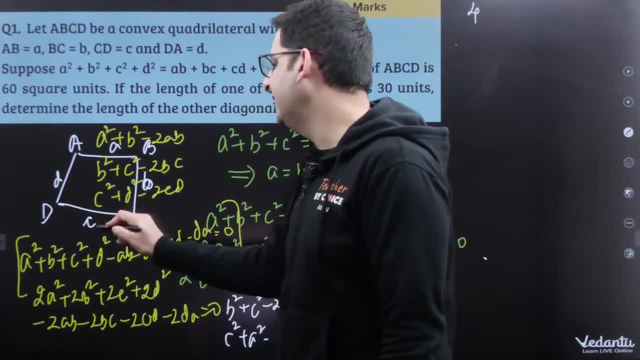 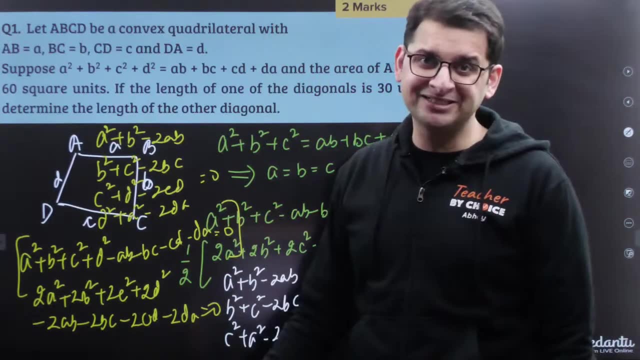 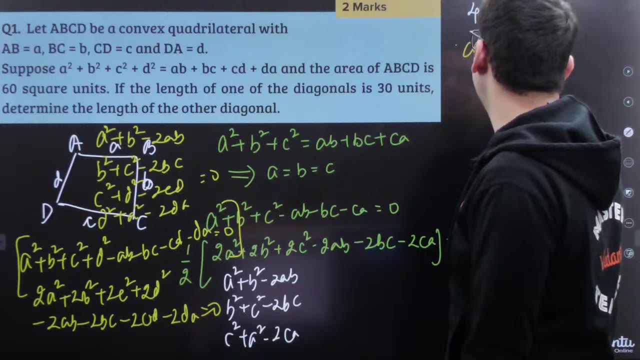 c square plus d. square minus 2 c, d and d square plus a. square minus 2 d, a is equal to zero. a minus b. square plus b minus c. square plus c minus a. square plus d, a is equal to zero. A is equal to B, is equal to C, is equal to D. This means this correlator is actually a rhombus. 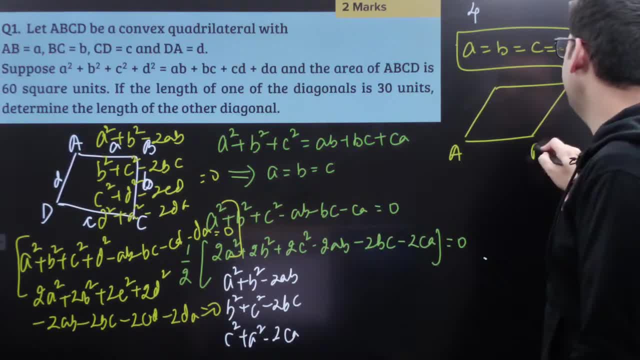 A, B, C, D. This is a rhombus. All of its sides are 4.. A diagonal is 30.. A diagonal is 30.. Area is 60. So half into D1, into D2, is 60.. 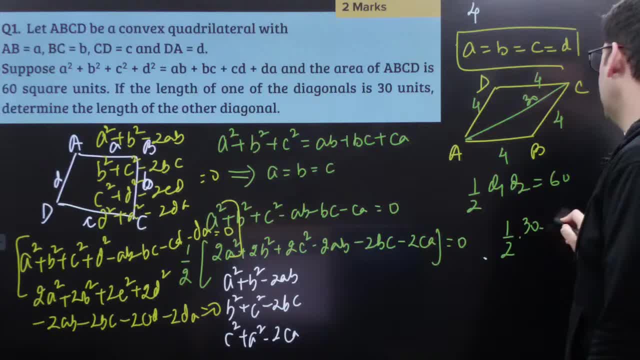 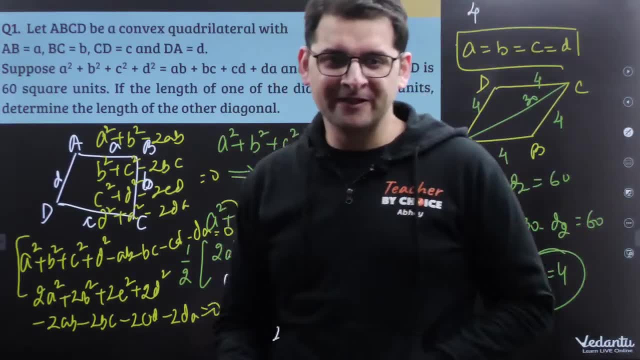 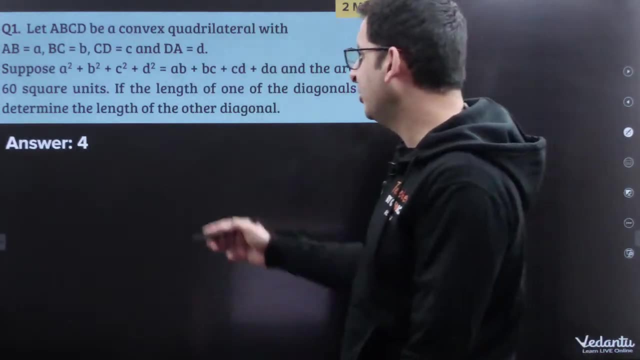 So half into 30 into D2 is 60. Giving us D2 is equal to 4.. 4 is the right answer. Is this clear everyone? Yes or no? Tell me quickly on the chart box: Kids see Two words are written on the chart box. 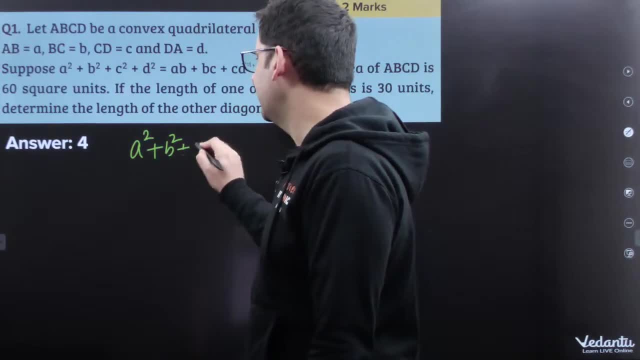 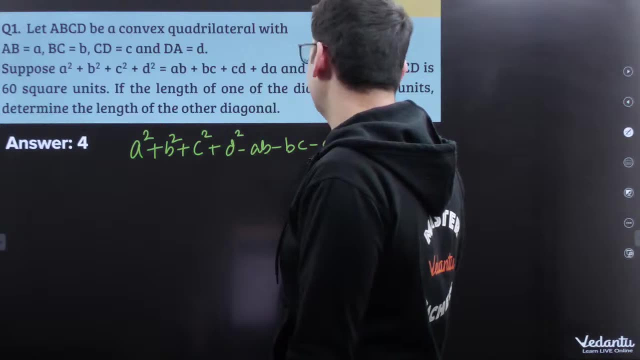 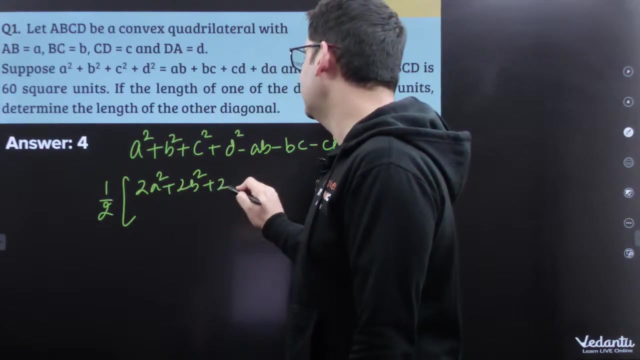 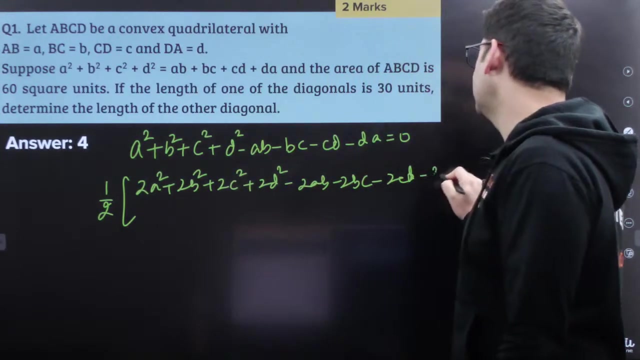 A square plus D square. minus A, B, minus B, C, minus C, D, minus D, A is equal to 0.. Do you agree? We have multiplied by 2 and divided by 2.. So 2 A square plus 2 B square plus 2 C square plus 2 D square, minus 2 A, B, minus 2 B, C, minus 2 C, D, minus 2 D, A is equal to 0.. 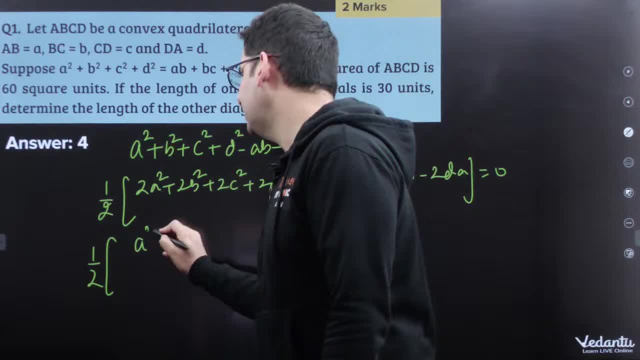 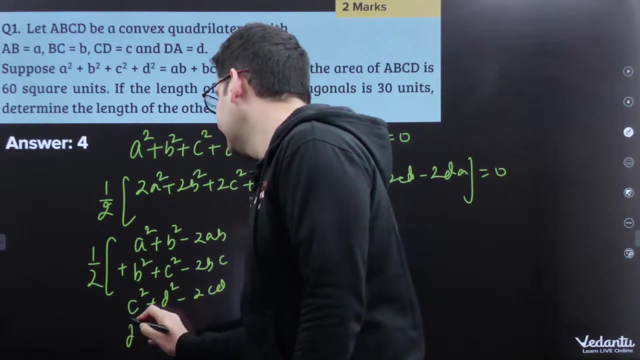 Half common. We have split this Half common. We have split this. Here we have A square plus B square minus 2 A. B is equal to 0.. plus B square plus C square minus 2 B. C plus C square plus D square minus 2 CD plus D square plus A square minus 2 D A. 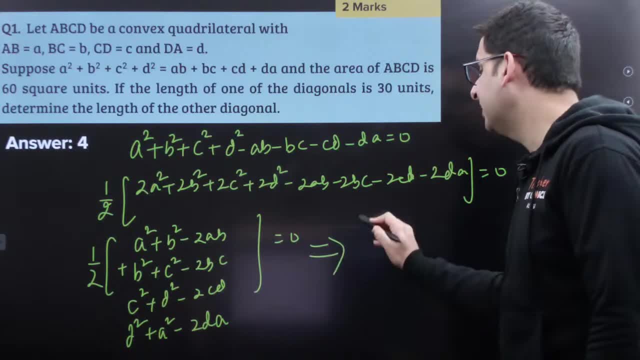 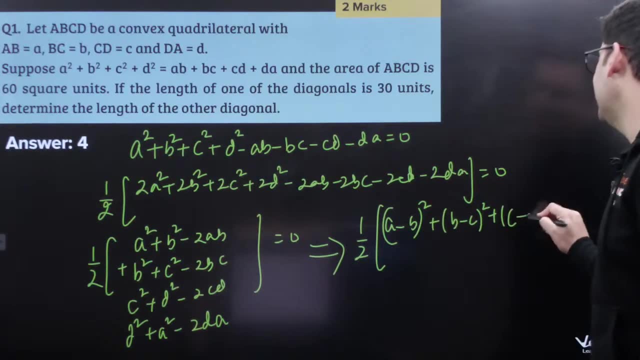 All of these have a sum of zero. This means, guys, half of A minus B whole square, B minus C whole square. C minus D whole square, whole square plus d minus a whole square. This value is zero, The sum of four non-negative numbers. 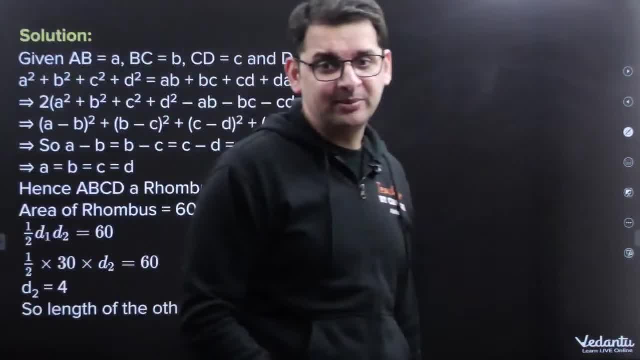 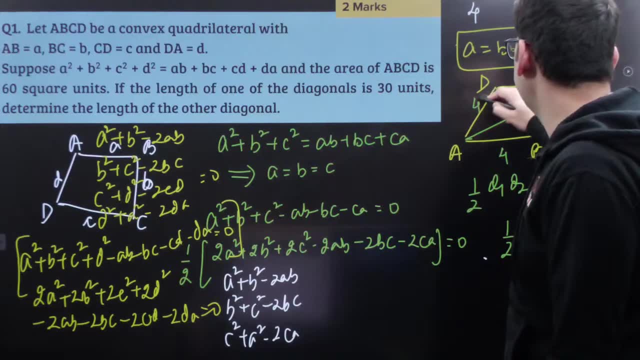 is zero. This means four of them are zero. So a and b and c and d are equal. I hope this is clear. Got it? Sorry, sorry, sorry, Yes, yes, yes, In fact this side is not four. I made a mistake. 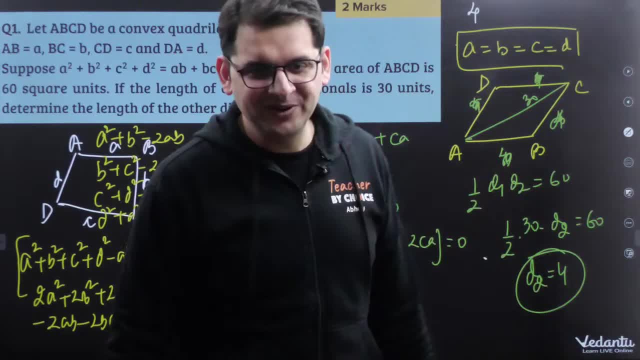 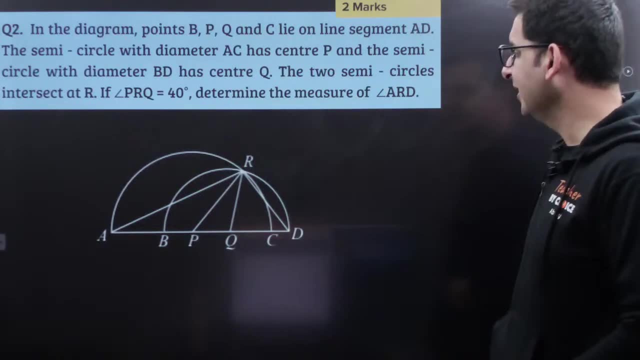 a and b and c and d are equal. It is not four. Okay, I got your point, Got it. Moving on to the next question, guys, which is this Very simple question: It is a very simple question, guys. It is a very simple question. Let's see. 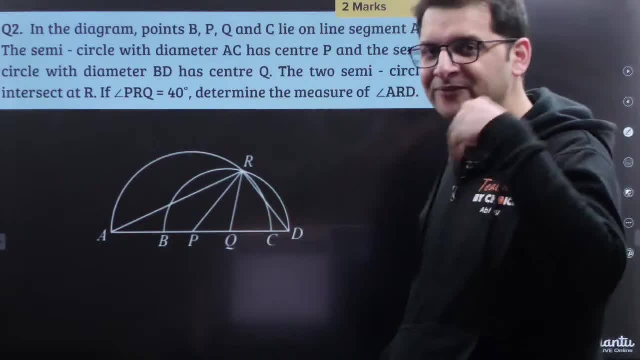 No, no, Bache Athar, you are right. By mistake, by mistake, it was in my emotions, It was in my emotions And I wrote four on the side. I told you. I have corrected it. It is not four, It is not four. 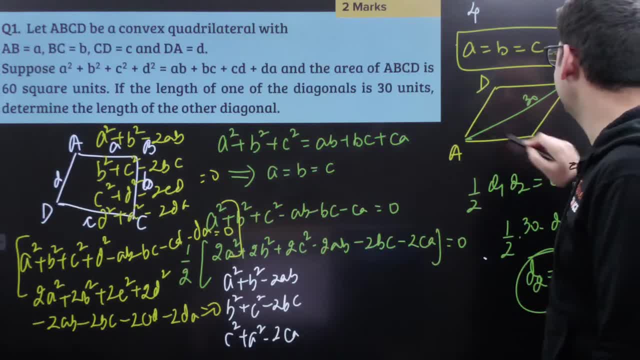 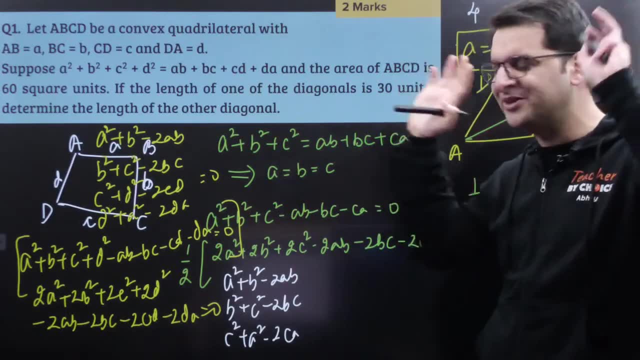 Let's remove it. Not four By mistake. I wrote it. I saw four all of a sudden. I actually remembered that it is four, So I don't know, I got confused, Forgive me. Moving on, Next question is this guys. 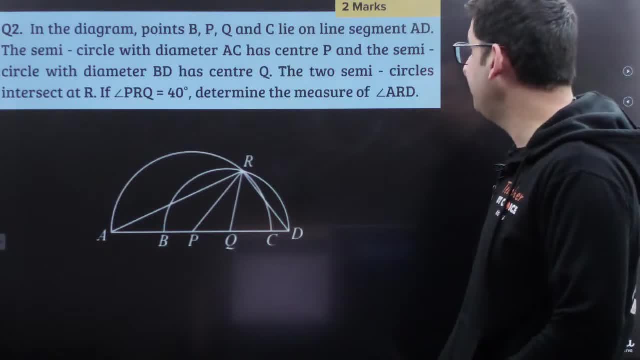 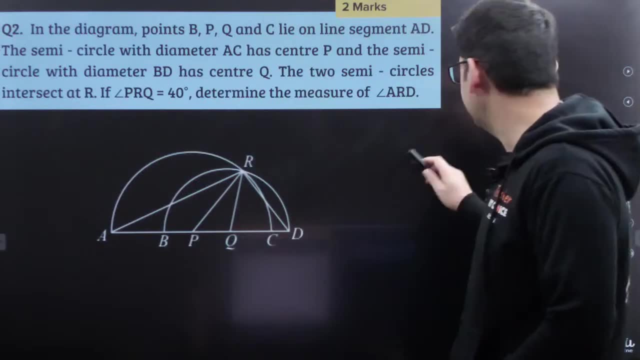 In the diagram, points B, P, Q, C, B, P, Q, C lie on line segment A D, The semicircle with A C as diameter. So let's make this Semicircle with A C as diameter. So again, this is the semicircle. 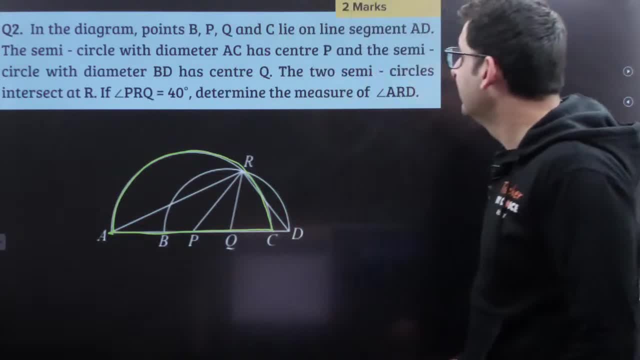 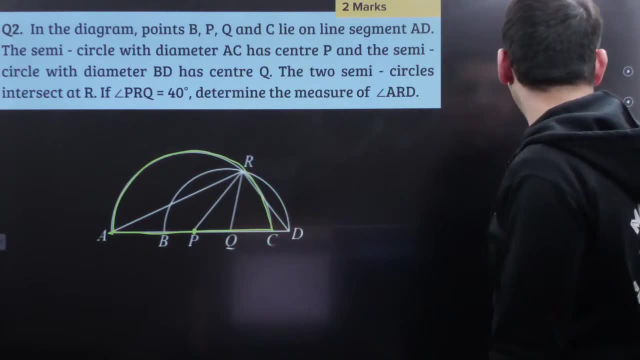 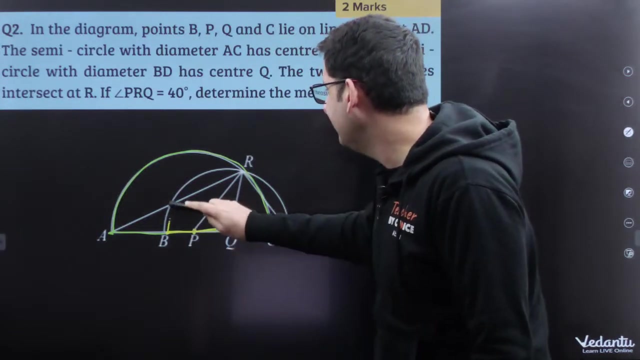 This is the semicircle. A C diameter. Done Has center P. Its center is P, Very good, Very good. And the semicircle with B D has diameter. There is one more semicircle. Its diameter is B D. This is the B D diameter. This is the semicircle. 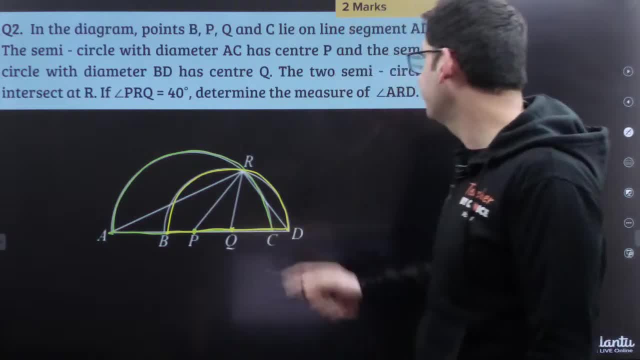 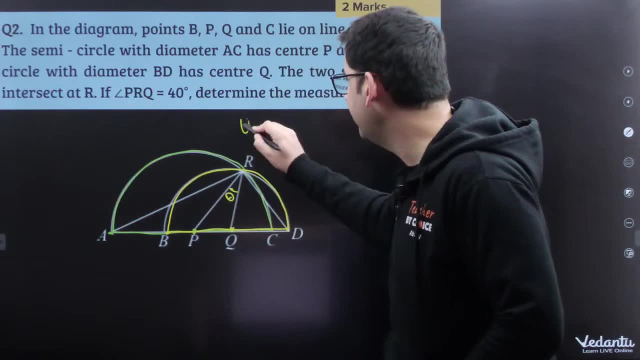 And its center is Q. The two semicircles intersected point are: If P, R, Q, This angle is theta, Theta is 40 degrees. Determine the measure of triangle A R D. Measure A R D. 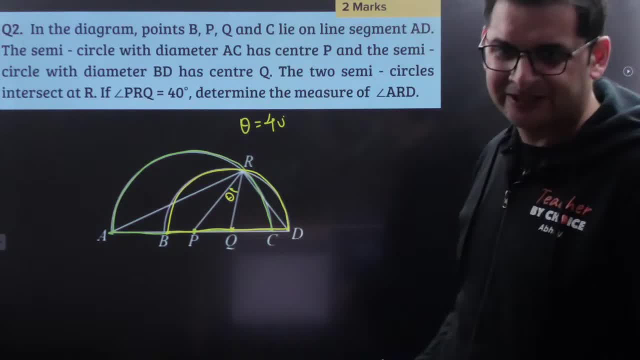 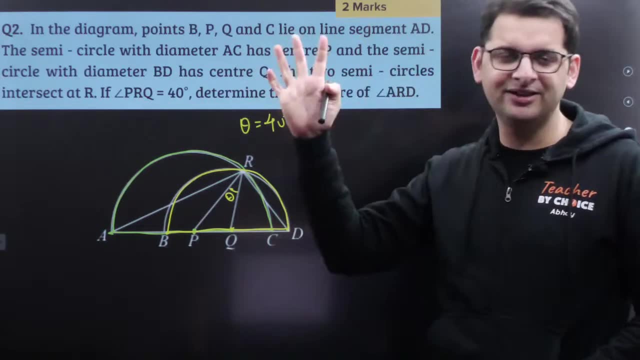 Fast guys, Fast, fast, Fast, fast. Yay, Adesh, Thank you. Thank you for correcting me. I didn't write a four by mistake. I didn't remember that answer by mistake, So I wrote four by mistake. It is not four. 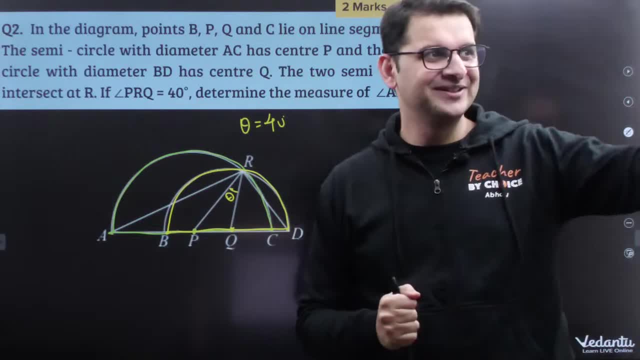 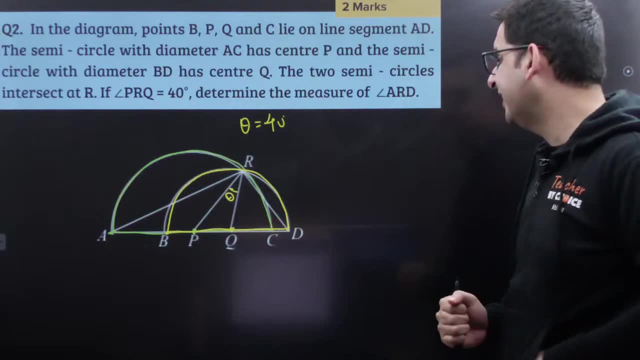 The only thing is: A is equal to B is equal to C is equal to D. Yes, Fast guys, Fast, fast, Fast fast. We have to find A R D Now. this kind of questions should be very quick. 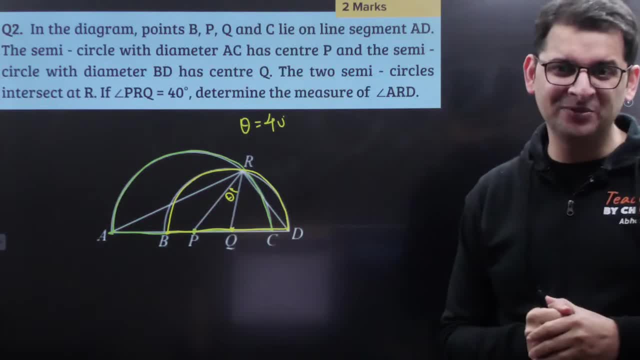 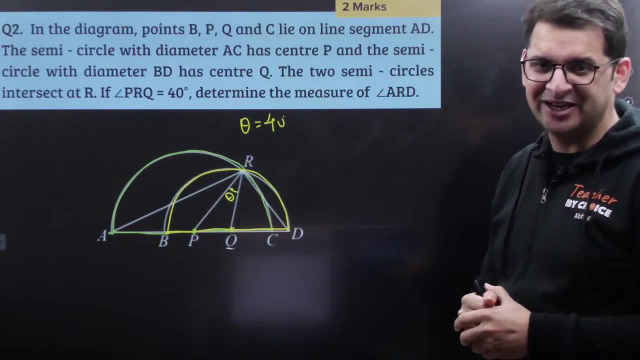 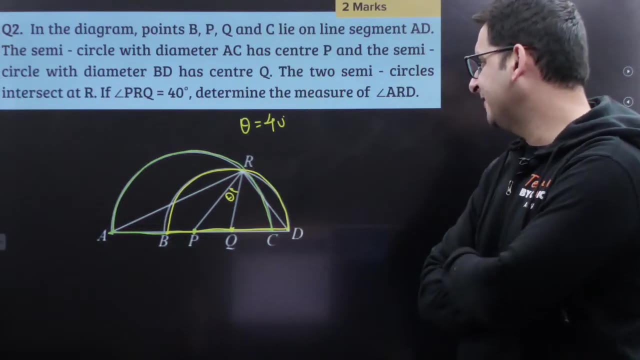 Should not take time. Should be very quick, guys. Should be very quick. Shashwat is saying 140.. Shashwat Singh 140. quickly, guys. what would be the right answer? what would be the right answer? tell me the right answer, P. 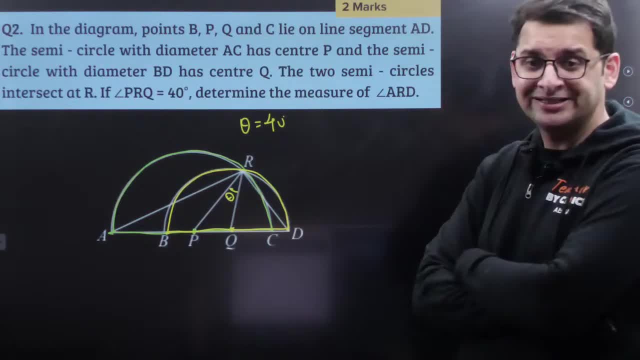 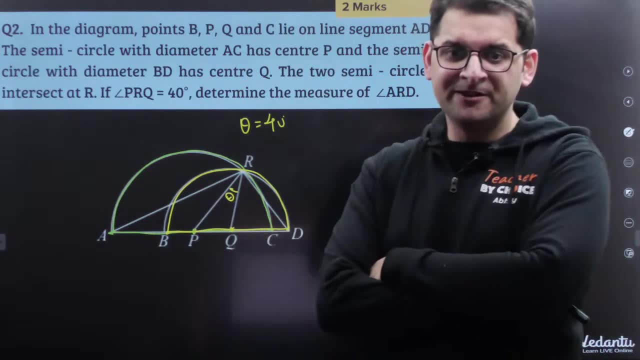 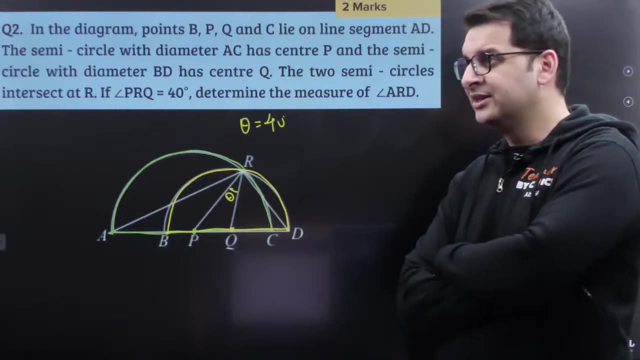 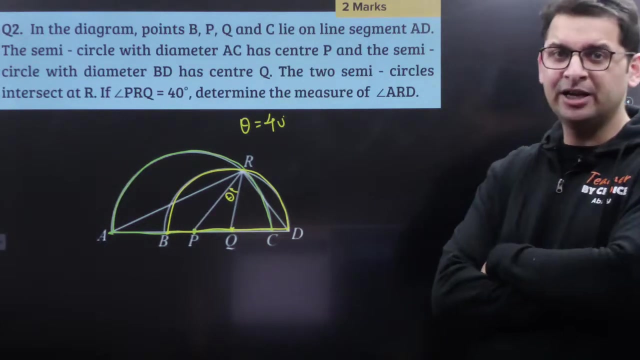 is the center of big semicircle. Q is the center of small semicircle. wonder solutions of life. please contact me over telegram after the session. we will check what problem is there. those who got more than 18 marks: we have corrected the copies of all those students. 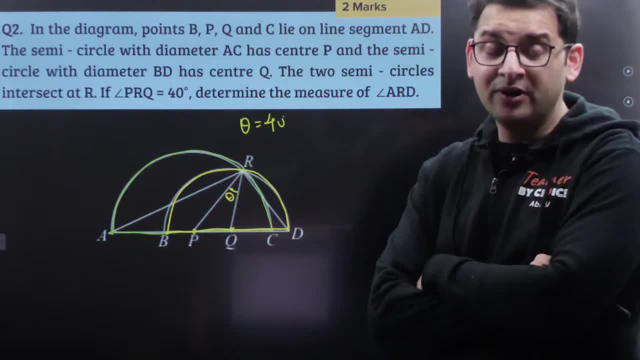 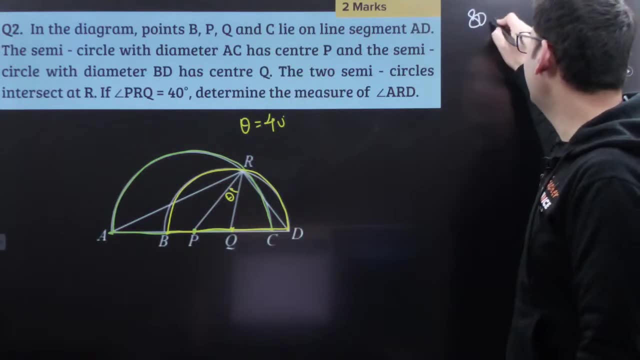 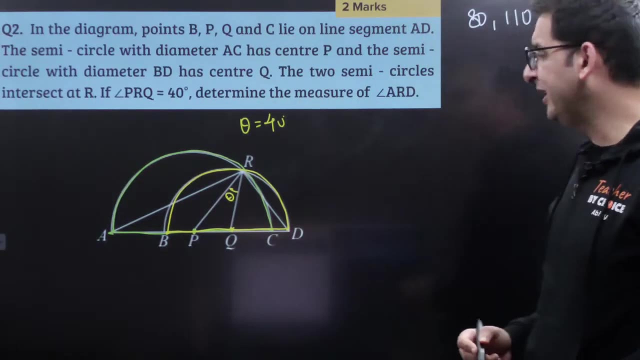 last Sunday test. Abhishek is saying 110. Tharav is saying 80, so two words have come: 80 and 110, 80 and 110. Rachit is saying 105, 105, 110, 80. how many? this is a simple question. 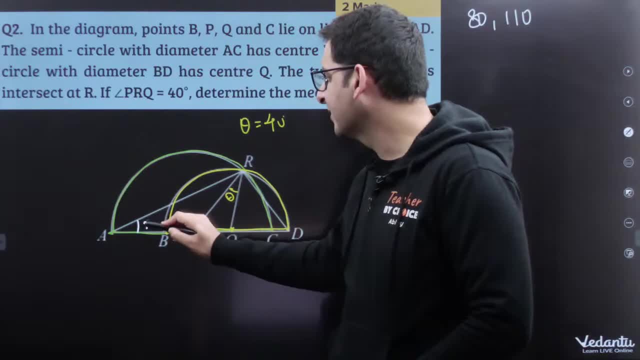 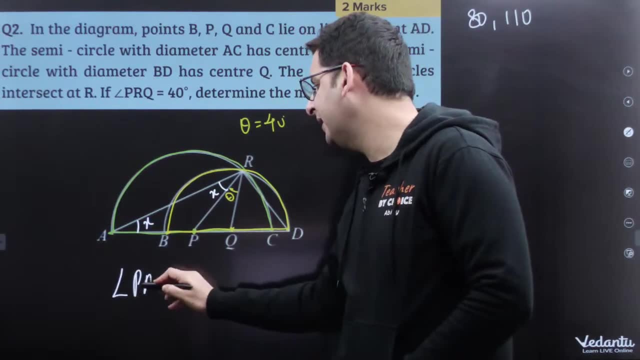 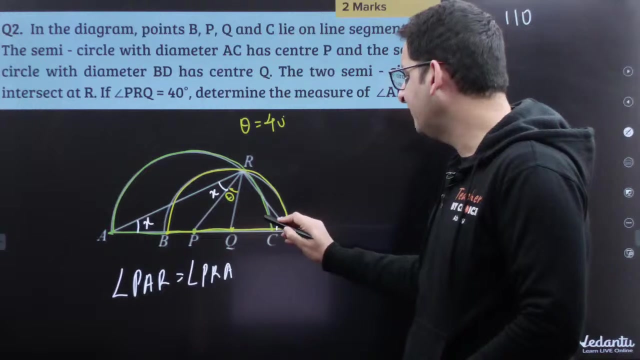 so Can I say: if this is an angle of x, this angle is going to be x. Can I say that? because par, these two are x. likewise, Q is center. if this is an angle of y, this angle is going to be y, because angle QdR. 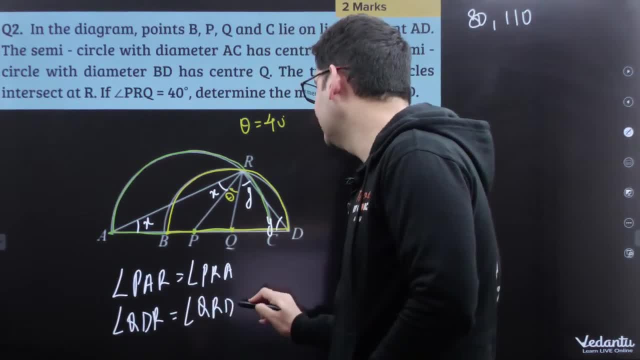 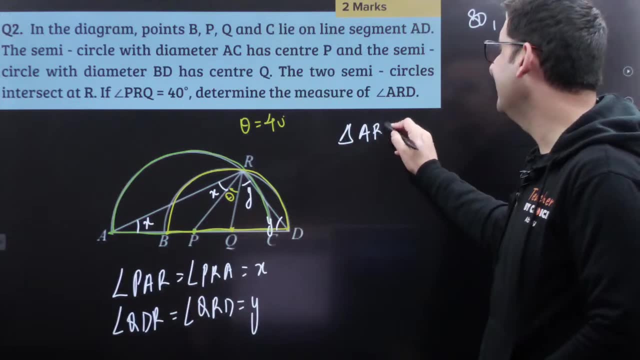 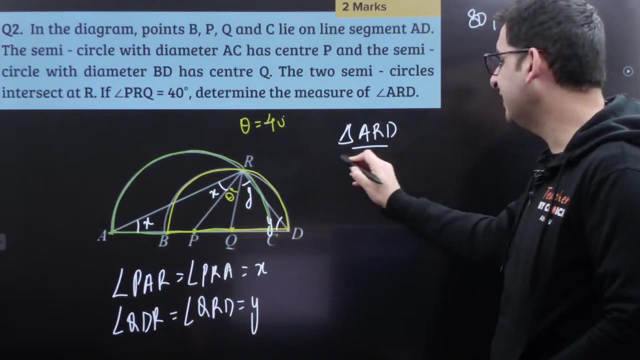 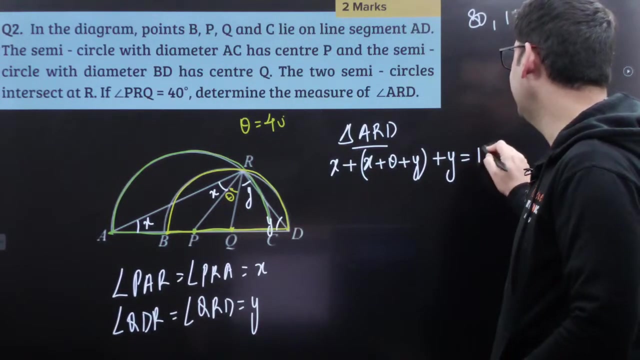 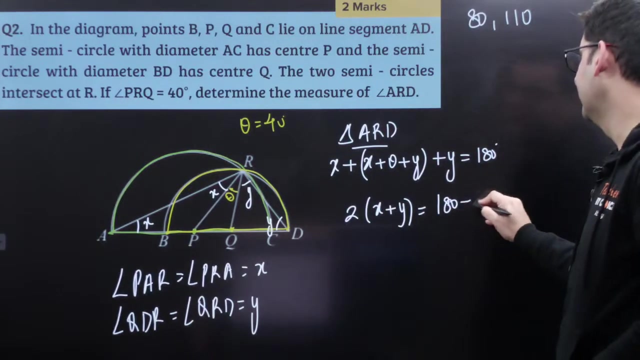 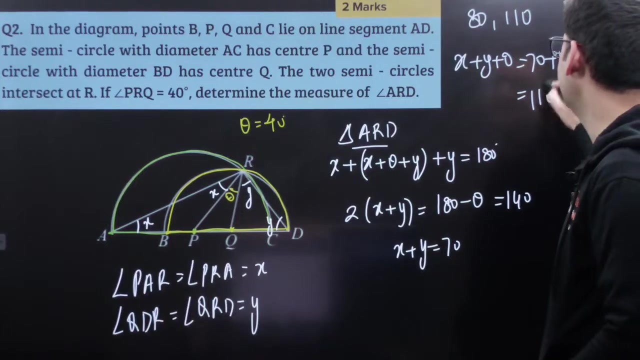 is equal to angle Qrd. these two are y. If we look at this triangle, x plus x plus theta plus y plus y is 180 degrees. So 2 times x plus y is equal to 180 minus theta. Theta is 40, this is 140, x plus y is 70, and we have to subtract x plus y plus theta, angle ARD. x plus y plus theta is 70 plus 40, giving us 110.. 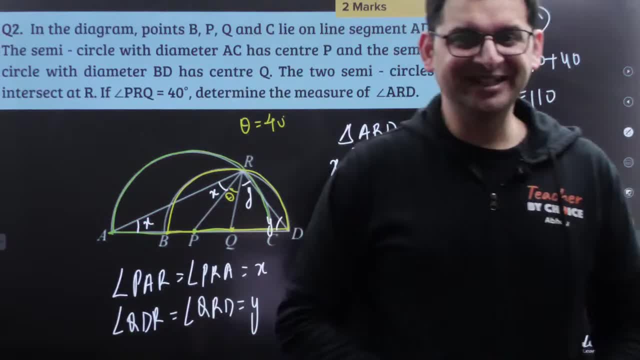 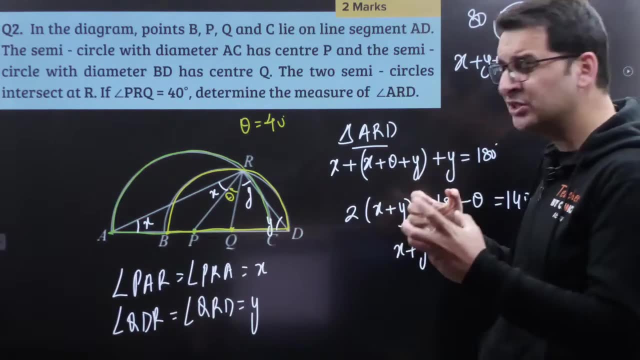 110 is the right answer. 110 is the right answer. Do you understand? So these type of simple questions, guys, simple questions. so there is confusion in this, because sometimes the diagram becomes very complicated and we get confused about what will happen. what will happen? 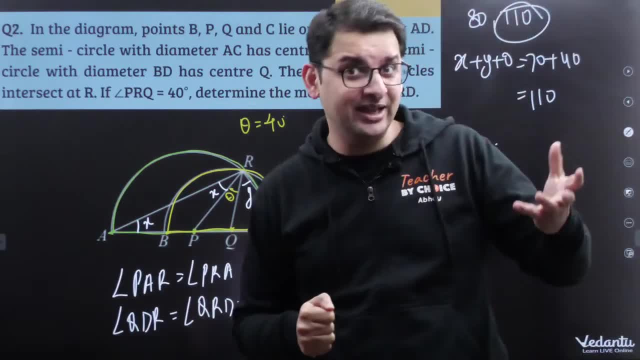 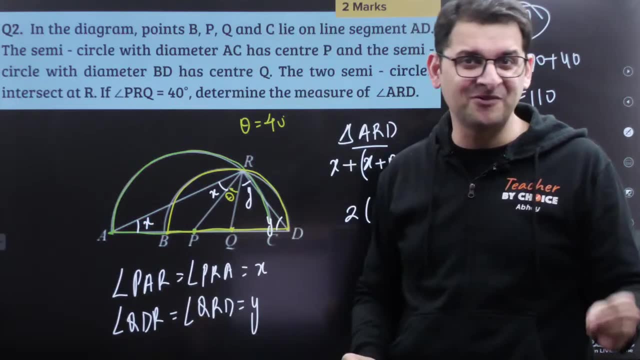 But the two questions, The four number questions that come in the geometry- can they come or will they come? they are very simple. so I just presence of mind logic, presence of mind practice. that is the only thing that you need to apply. 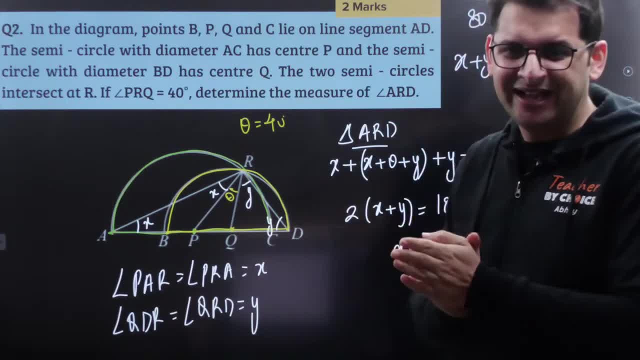 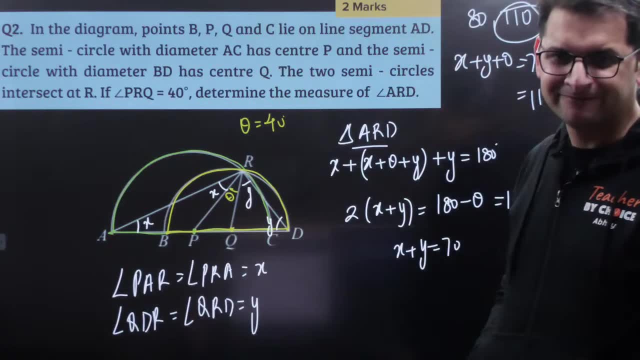 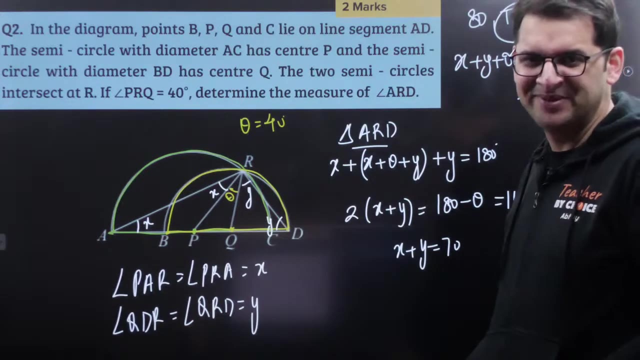 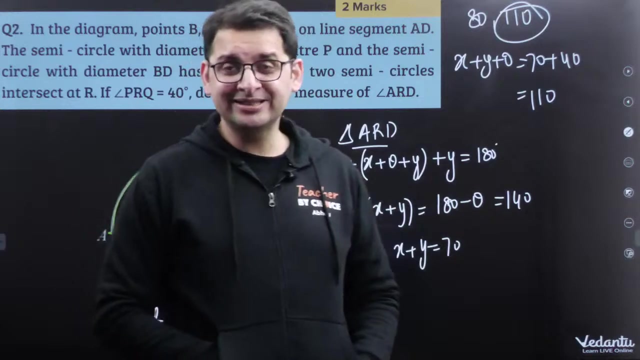 Got it, got it, got it. yes, Yes, Amazing, Amazing, Got it everyone? Did you all get this? Super, Super, Super, Amazing, Yes, yes, yes, we should not be judging. yes, Look, mistakes can happen with everyone, and you saw that I also made a mistake in the last question. 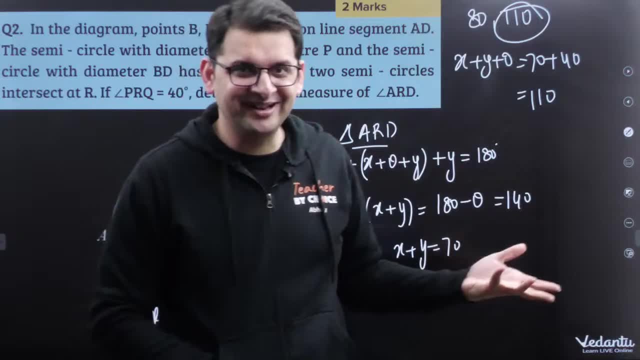 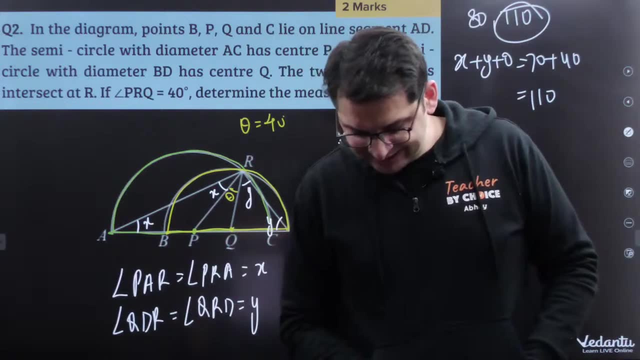 Okay. so if you start writing that sir Abhay, sir doesn't know, he doesn't know how to teach, then how will it work, man? Okay, so mistakes are the proof that we are humans. Mistakes are the proof that we are humans, not God, right? 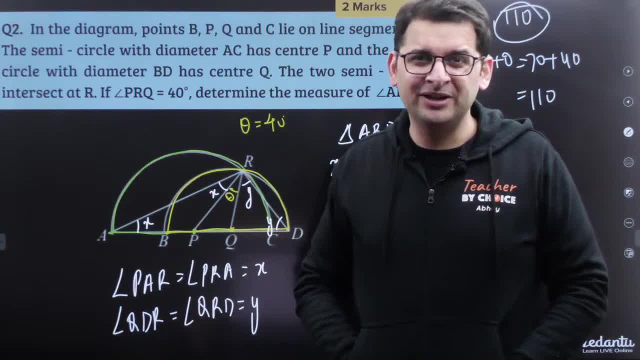 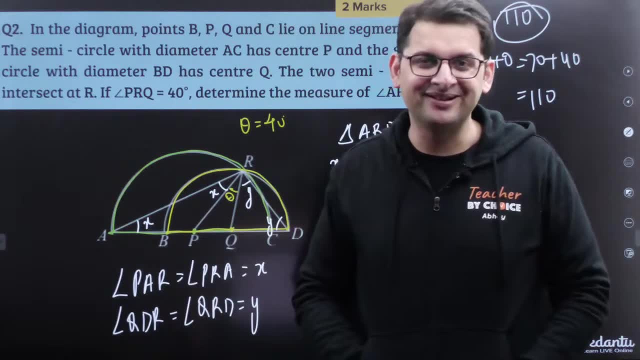 So, yes, So we should not be judging, because everyone will make mistakes. you will also make mistakes. everyone will do mistakes. okay, Virat Kohli has been making mistakes for the past year. he is not able to hit the century, okay, so so, but that doesn't mean Virat Kohli is a decent cricketer. he still is a top class cricketer. 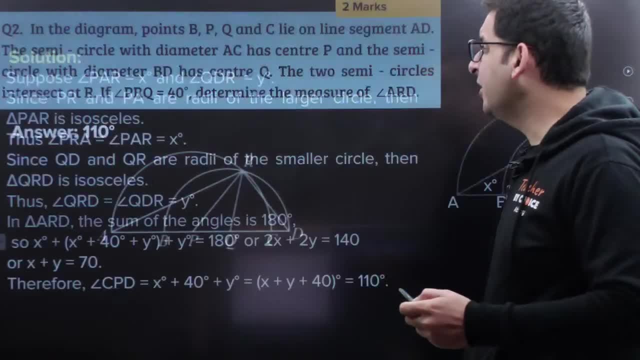 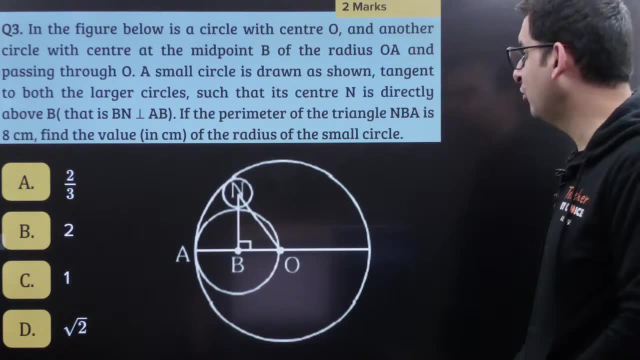 Yes, okay, okay, but I'll try to increase the time. Moving on next question is this: Okay, guys, now this question, everyone has to ask. this question everyone has to ask. I'll give you time. I'll give you time at least three minutes. 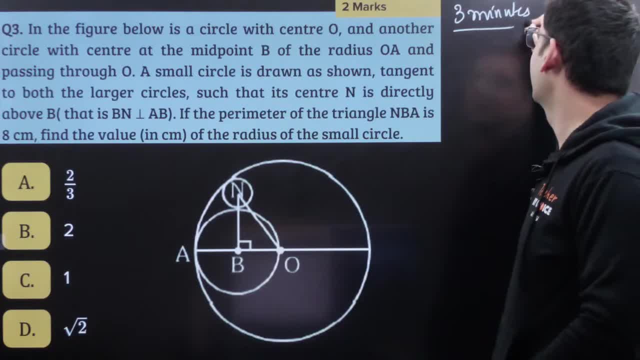 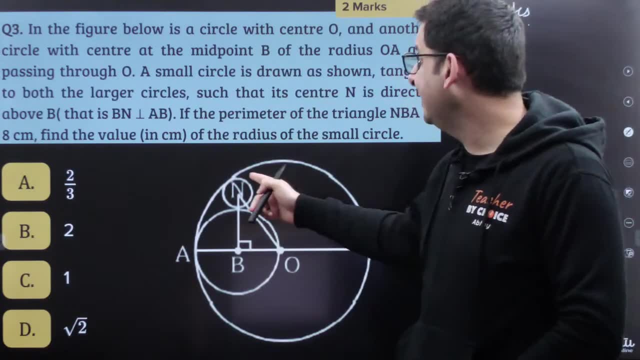 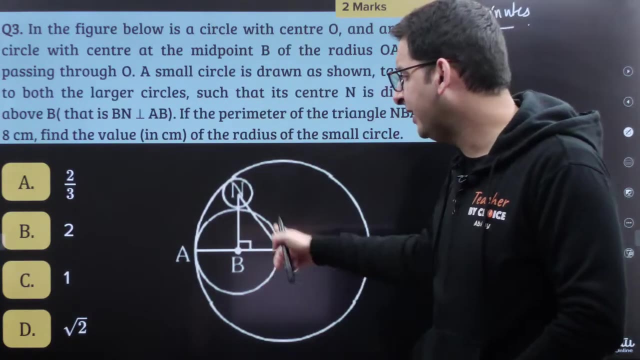 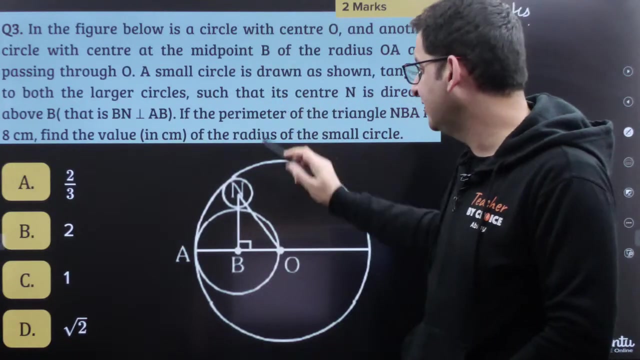 In the figure below is a circle with center O and another circle with the center at midpoint of the radius OA and passing through O. okay, So OA is one radius and it's midpoint is B. another circle is drawn. a small circle is drawn as shown. this is a small circle. it is drawn tangent to both the larger circles. this circle is touching this and this larger circle as well. 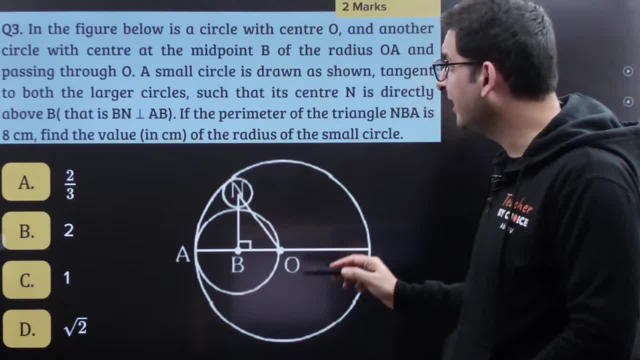 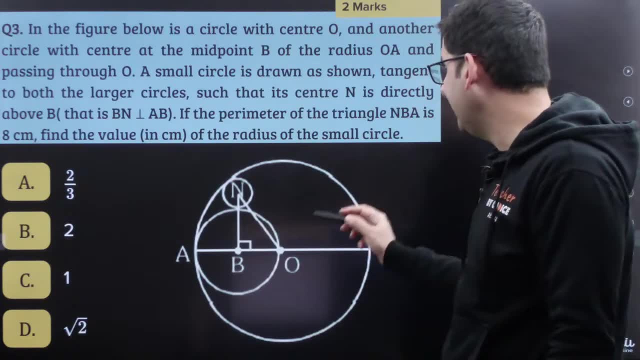 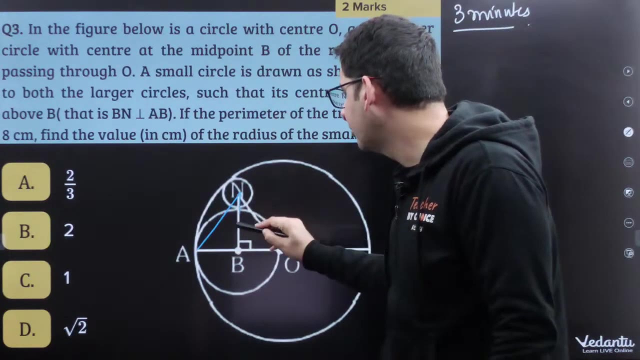 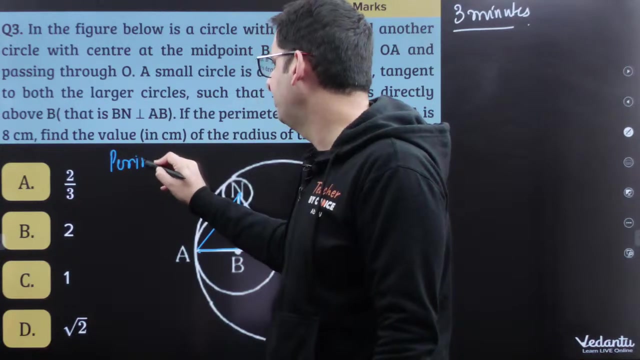 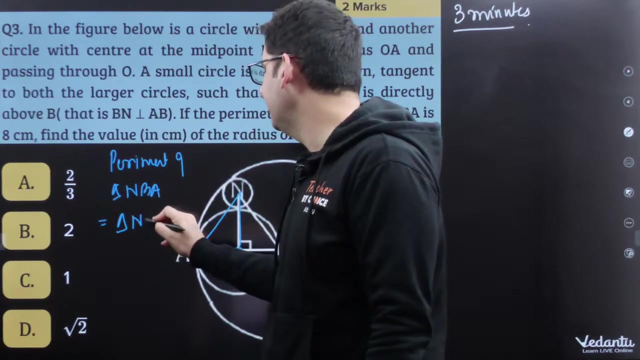 Okay, Okay, Okay, Okay, Okay, Okay, Okay. its center n is directly above B, which means Bn is perpendicular to AB. If we draw the perimeter of the triangle NBA, its perimeter is 8. And it is known to me that the perimeter of the triangle NBA is the same as the perimeter of the triangle NBO, by symmetry. 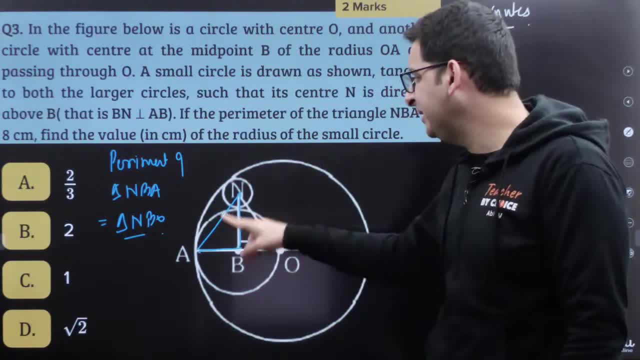 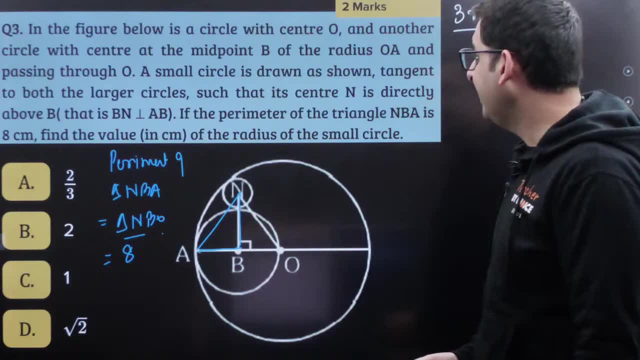 Because the circle is just above. the perimeter of NBA and NBO is the same and both their perimeter is 8 cm. Find the value of radius of smaller circle. we have to find the radius of smaller circle. Let's say small circle radius is smaller. 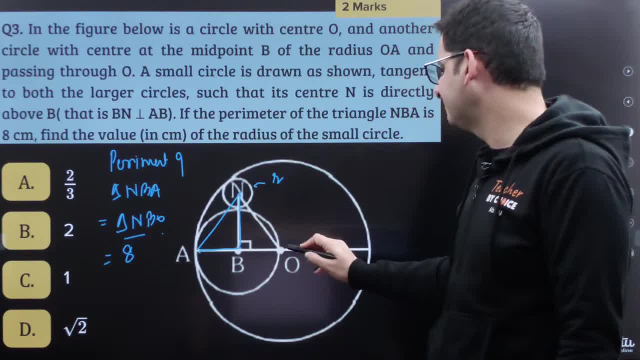 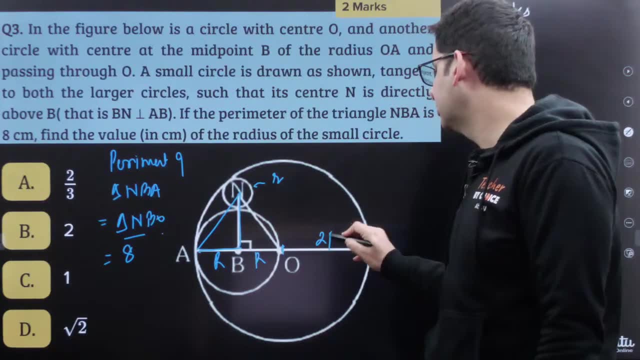 Find the value of radius of bigger circle is 7.. Find radius of smaller circle: radius is 10.. Find radius of bigger circle: radius is 10.. radius, capital R. Let's assume this is capital R. This is capital R. This is 2R, So the largest. 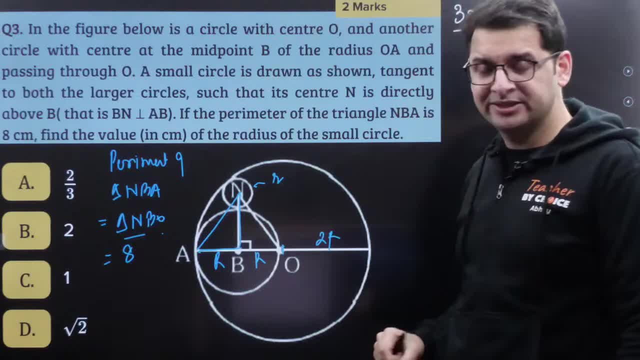 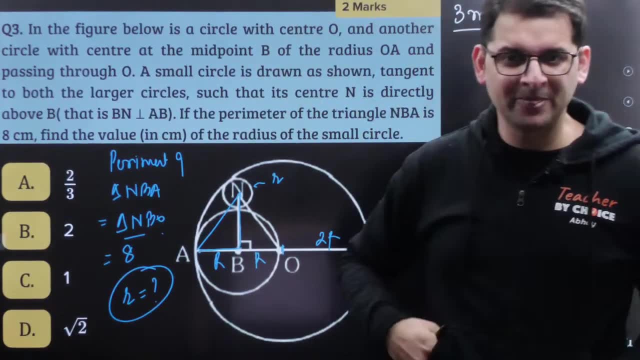 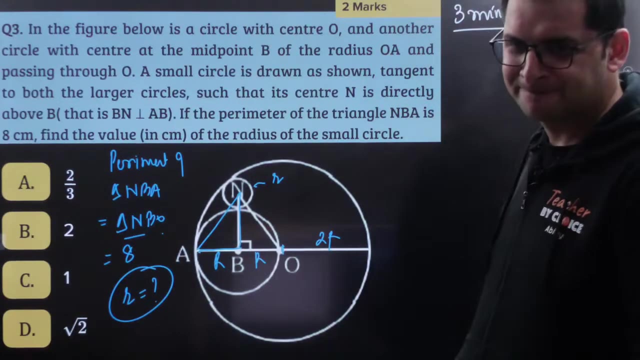 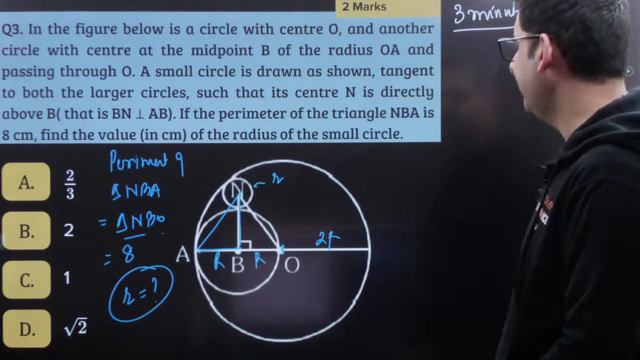 circle radius is 4R. The radius of the middle circle is capital R. The radius of the smaller circle is small R And we have to find small r. The ask is: we need to find small r? We need to find small r? What is going to be the right answer? The value of small r will. 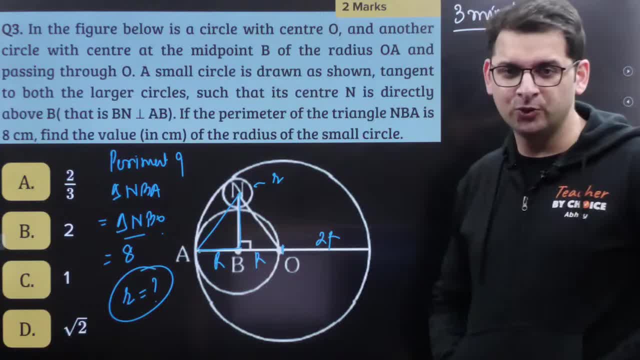 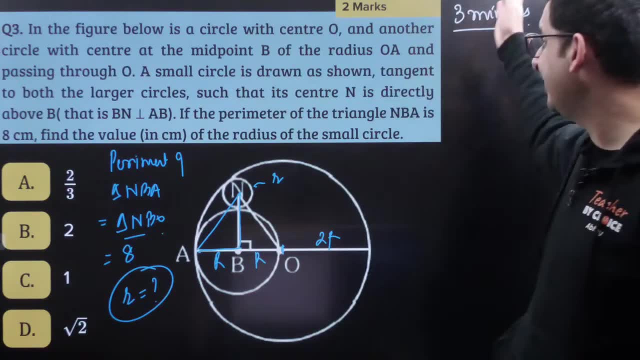 be 2 by 3.. It will be 2.. It will be 1.. It will be root 2.. Which one will be the answer? What will be the right answer? I will give you a time sign. It is written as 3 minutes It. 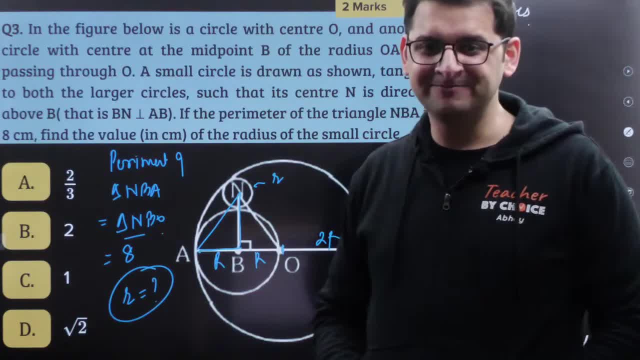 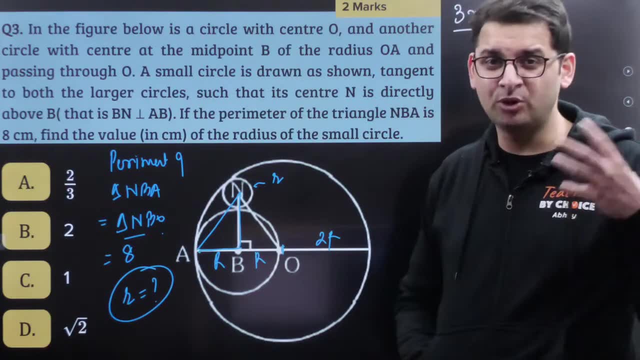 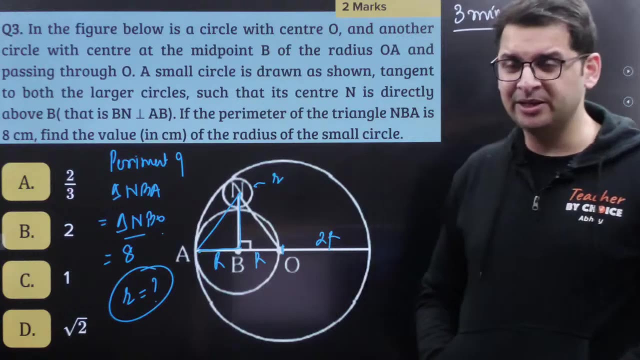 has been almost 1 or 1.5 minutes. Tell me quickly KVPY. I think we should get a notice of KVPY very soon because the cases have dipped down a lot And I think the first priority will always be the Olympiads, because the Olympiads- 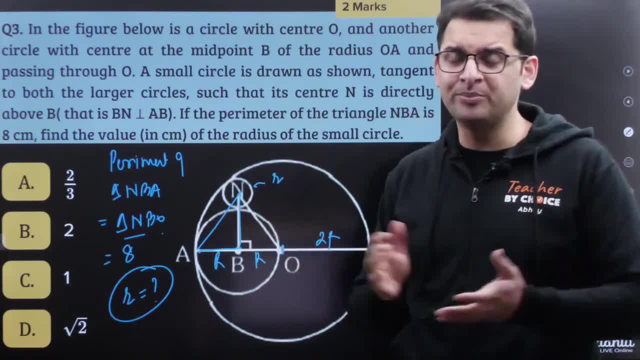 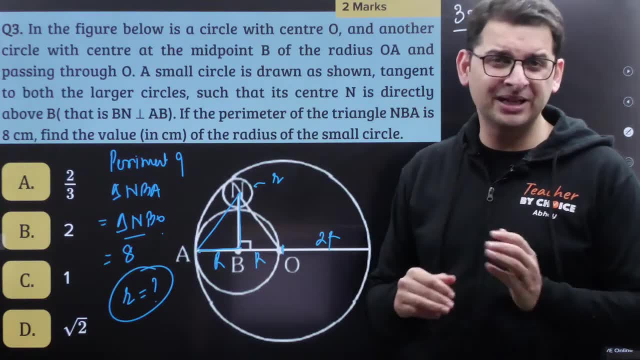 are in a way attached to international competitions And India has to select teams. KVPY is an internal examination, So I think even if it happens after the boards, it will not make much difference because ultimately they have to select some students and give them a scholarship. 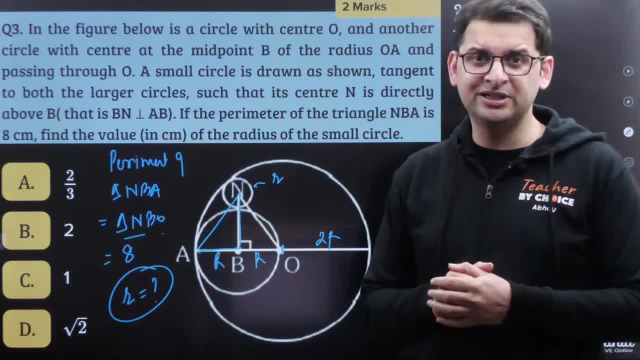 So I think even if it happens after the boards, it will not make much difference because ultimately they have to select some students and give them a scholarship, Although it is different that the prestigious institutes like IIC, their admissions are also on the basis of KVPY. 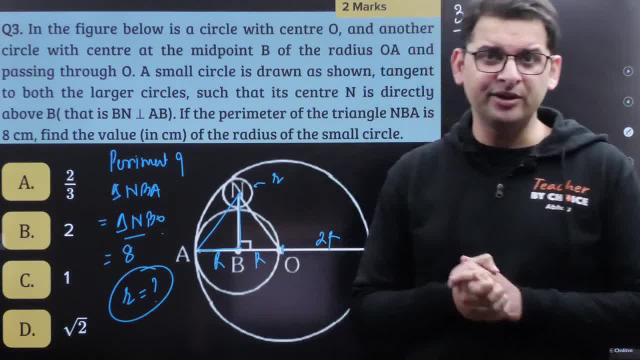 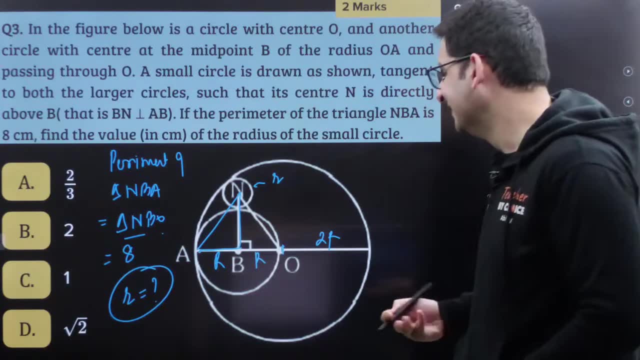 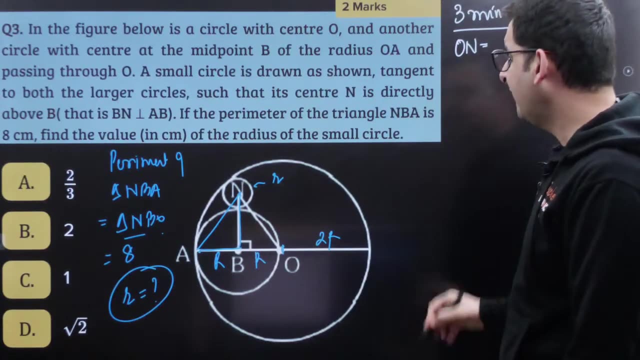 So, again, I think that its date will also come soon, but the priority would always be Olympiads. Alright, So a lot of people are saying 2 by 3.. Amazing guys, Amazing, So guys. yes, exactly As Alfa wrote. Alfa said that, sir, the value of O is going to be 2r minus r, Do you all? 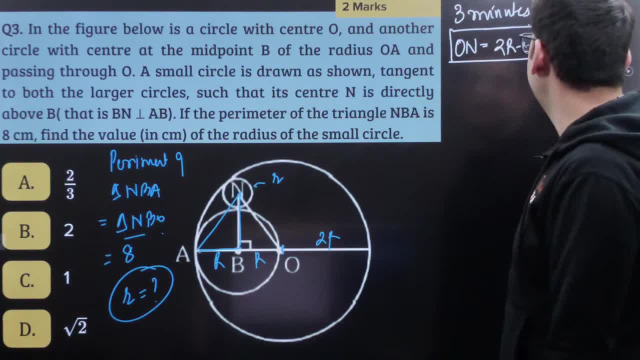 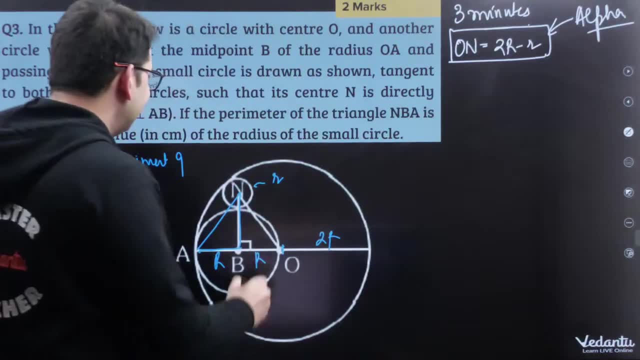 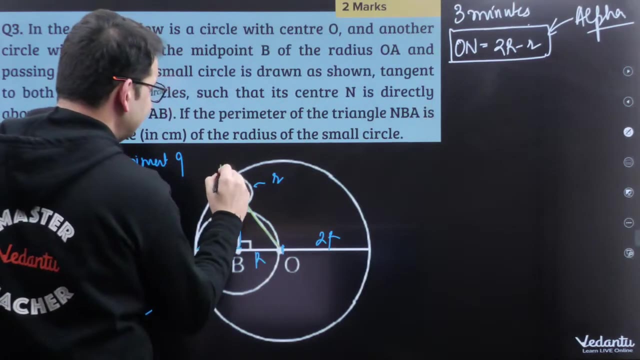 agree with Alfa. Do you all agree with Alfa? So Alfa has said that. the value of O, because if I extend it from here to here, let's say this is p and this is going to be small r, So 2r minus small. 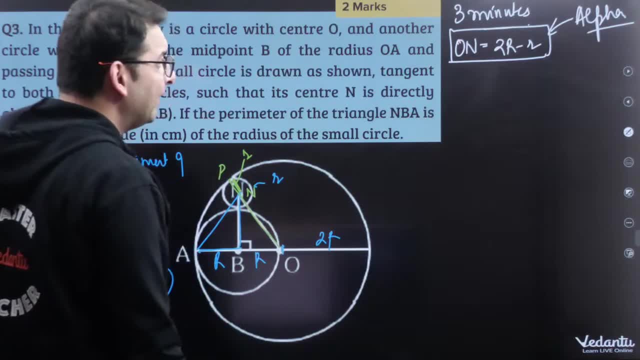 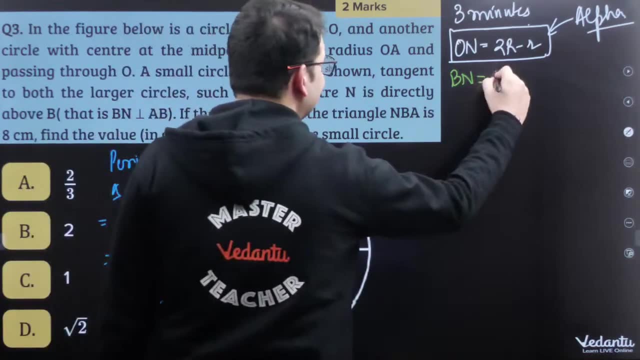 r. this is going to be O. O is going to be 2r minus small r. So this is clear, Alright. So the value of Bn: the value of Bn is going to be capital R plus small r and the value 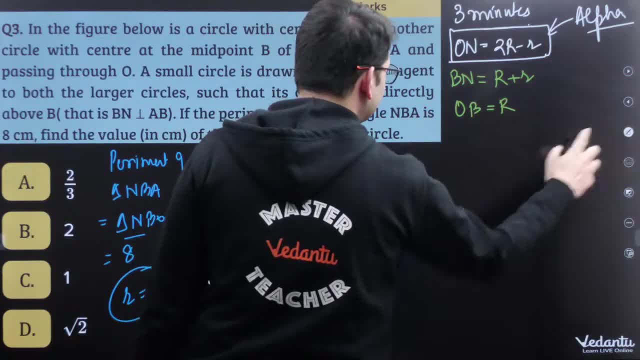 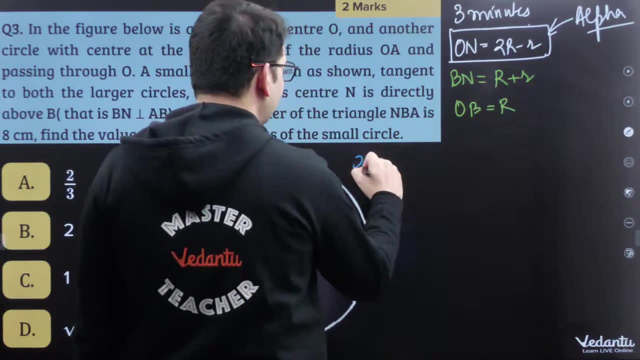 of Ob is going to be r, So can I apply Pythagoras here? Can I apply Pythagoras here? So if we apply Pythagoras here, Pythagoras, so clearly 2r minus r whole square is equal to r plus. 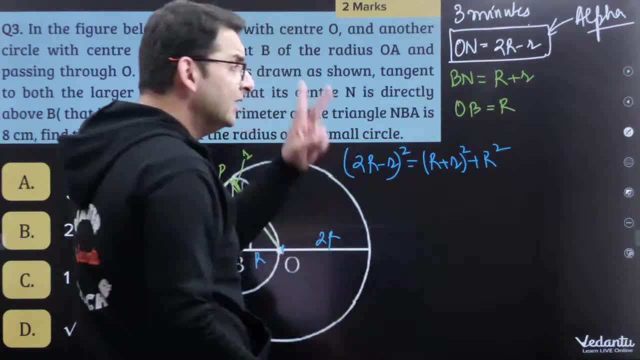 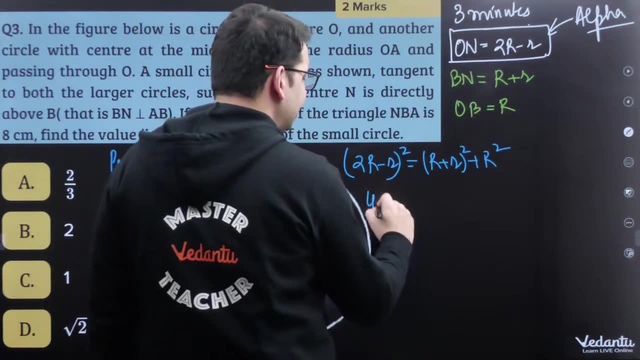 r whole square plus r square. This is the condition. There are two variables: capital R and small r. We need two equations. So there is one equation. it will come from the other parameter. So the work is sorted: 4r square plus r square minus 4r. capital R is equal to r square plus. 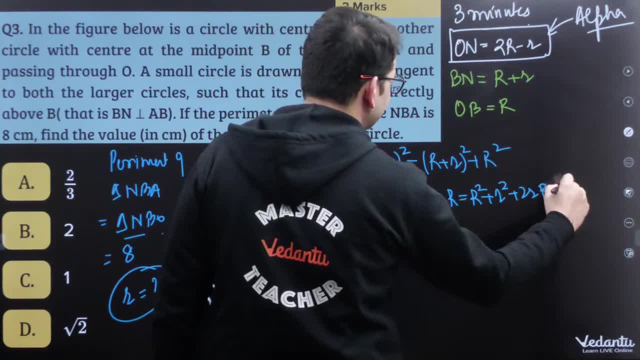 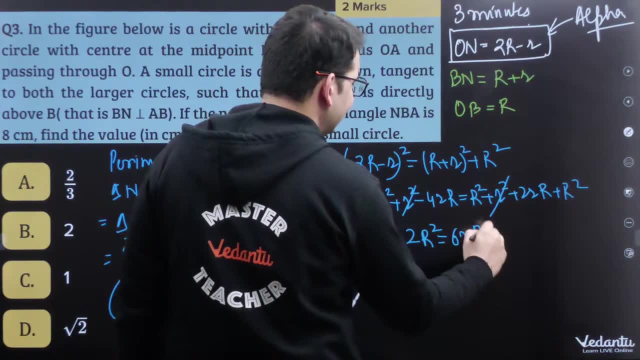 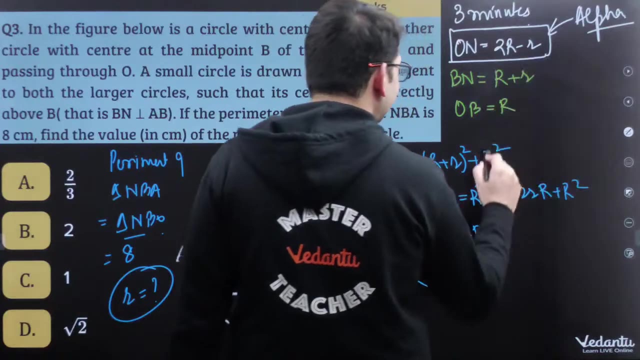 r square plus 2r. capital R plus r square. This is cancelled. 2r square is equal to 6rr. This is cancelled. So here capital R becomes equal to 3r. Sorted Capital R, 3r And this: 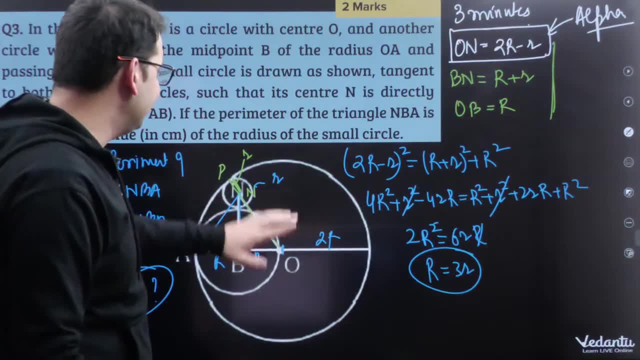 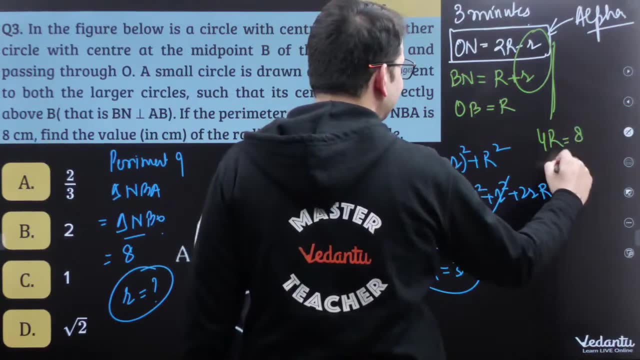 perimeter, its perimeter, the perimeter of nba and nbo is the same, So if we add it, then this is cancelled. So 2r 4r. So 4r is equal to 8, capital R is equal to 2.. As we 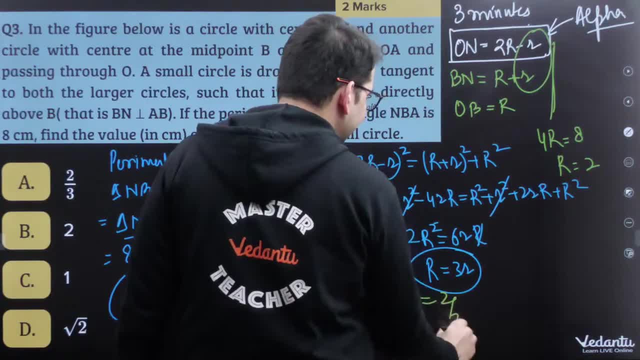 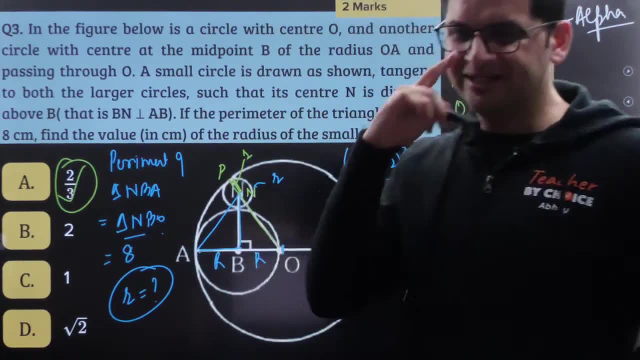 kept capital R 2, then the value of small r is 2 by 3.. That is the right answer. 2 by 3 is the right answer. I hope this is clear. Got it everyone. Did you all get this Got? 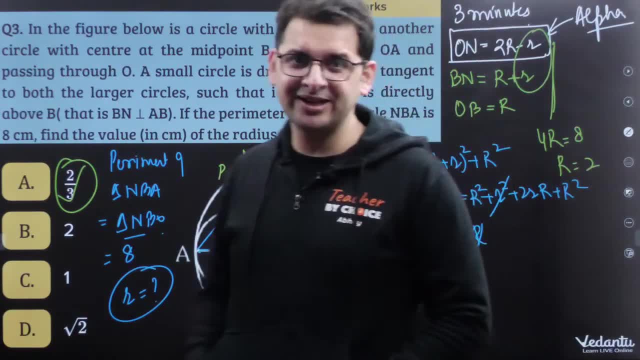 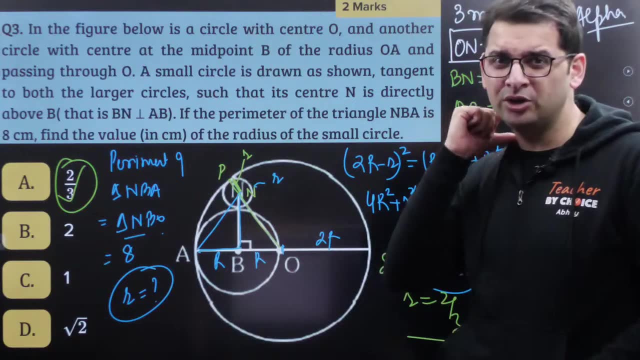 it everyone. Yes, yes, yes, Yes. kids, you have practiced so much that you have such questions. Now you will only get one marker. okay, And these are heavy, the same kind of questions. If you have seen, then the questions of two markers are very simple. If we talk about 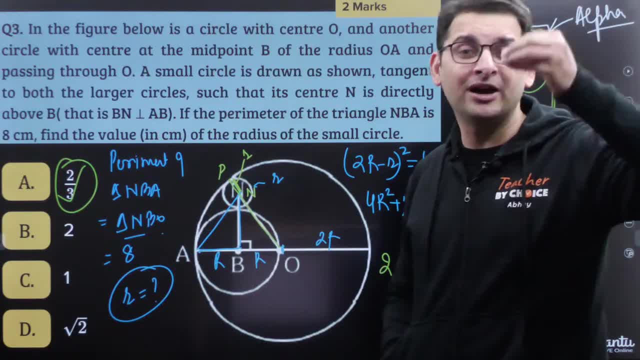 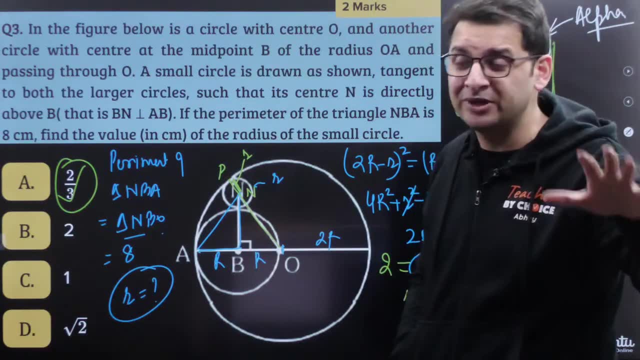 IOCUM. then the more you practice, the more you will move forward. the more you will practice, the more you will see things, the more things will start looking easy. For example, today you are finding the question of two numbers difficult, If you practice. 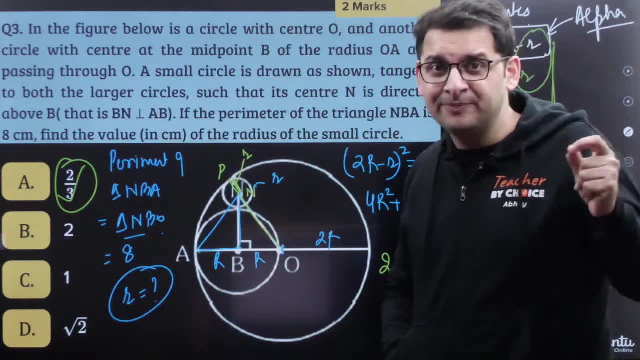 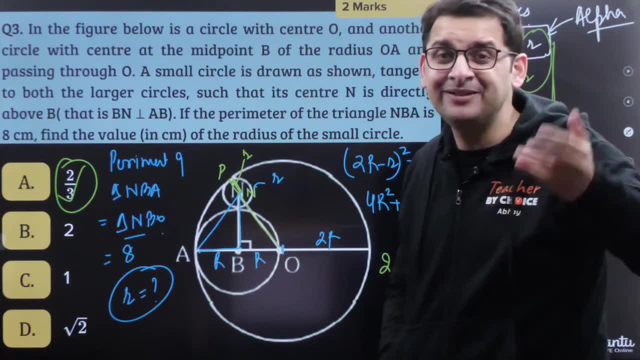 Maths for three months, practice Maths Olympiads. then the same three-number question will be easy for you. You will find it of two numbers, you will find it of two numbers, you will find it of one number, and so on. So in this way, if you are saying that, sir, 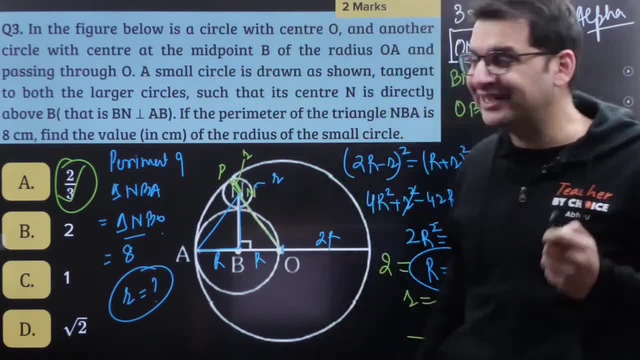 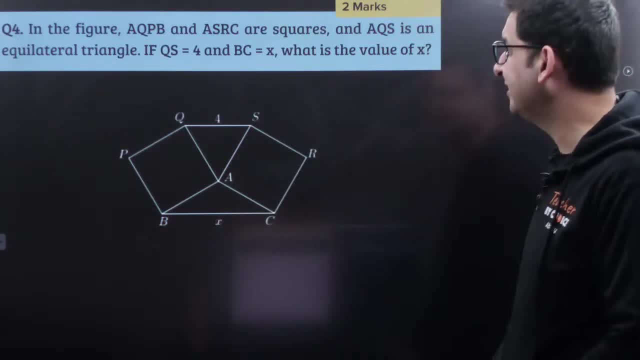 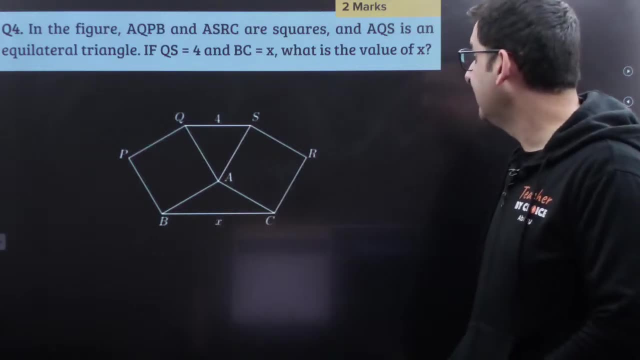 these questions are easy, then again, it means that you have got up as simple as that. Moving on, next question is this? Next question is this? Very simple question, guys. In the figure, AQPB and ASRC are squares and AQS is an equilateral triangle. So AQS is an. 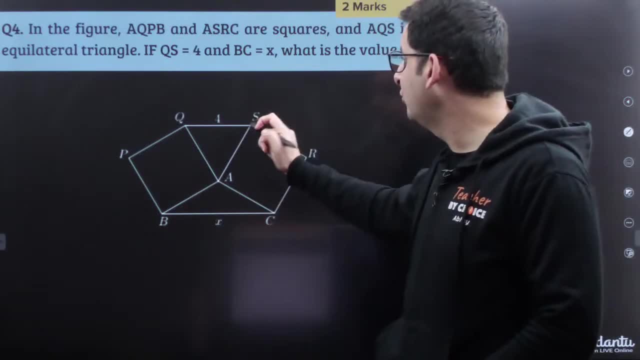 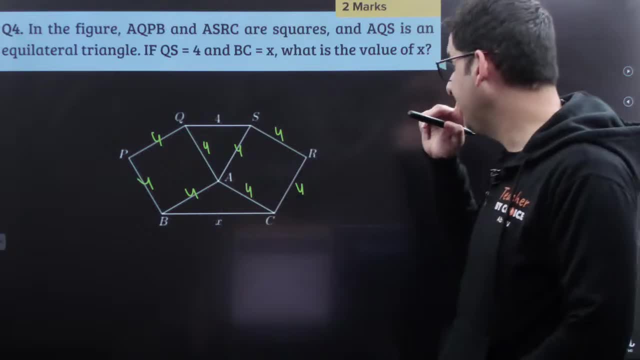 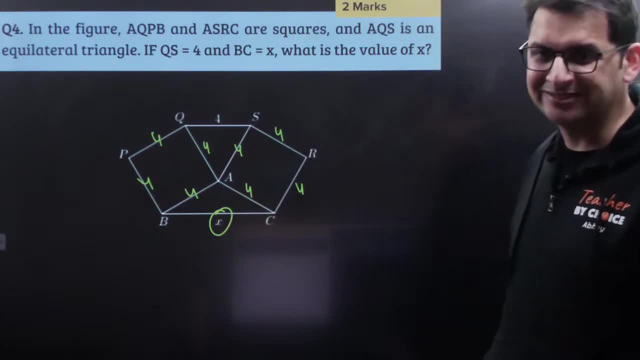 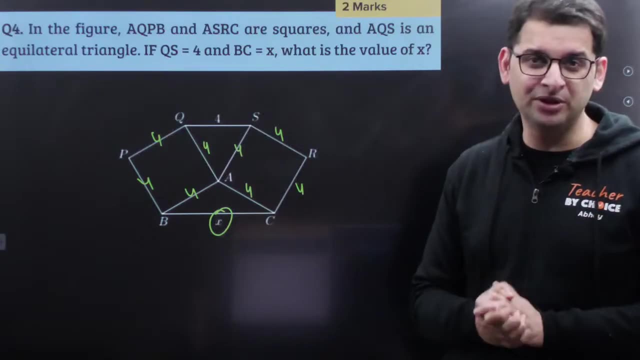 What is the value of X? Quickly, guys, I am not going to give much time in this. This is a very simple question. All the two markers are actually one marker questions, very simple questions, And you have practiced a lot, so you guys should get half the time. 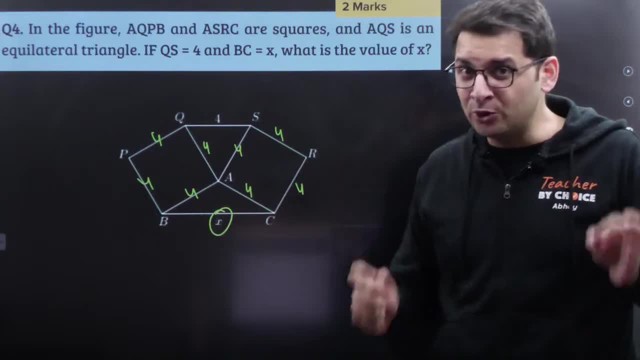 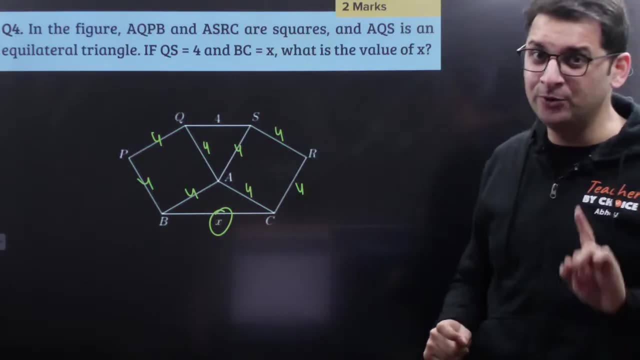 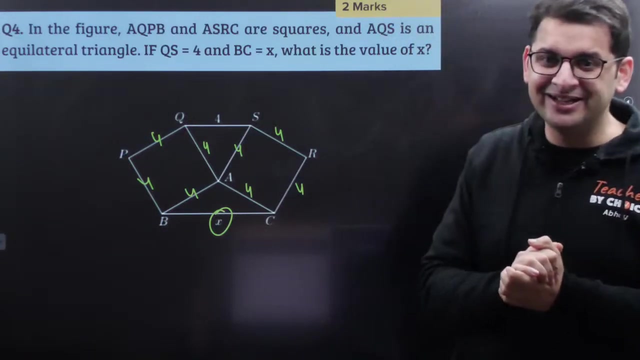 as much as the rest of the people who are following our lectures, the kids who were in the exams of the Vedanta school in general batches in the camp. They recently reached a higher level. You guys should get least time than them. This is the kind of speed that I want all between us. Amazing, sendai, amazing. 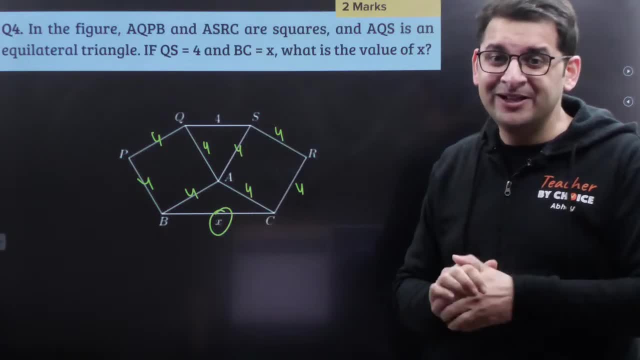 amazing, Arav. This type of speed is what I need. I am speaking to you and you have insulted there. I am very sure that he absolutely will do it. It has been a pleasure hearing about it at the time of the interview And today he's doing aEPEк. 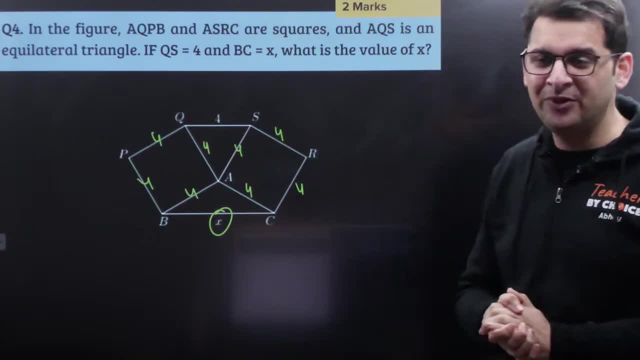 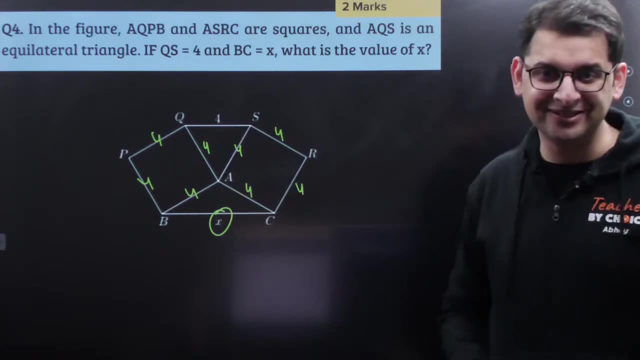 I am very sure that you have done a calculation just now. Yes, Navya. today I have a lecture on INMO at 6.30 pm. We are going to discuss functional equations with numbers of INMO. We are going to discuss very amazing questions. 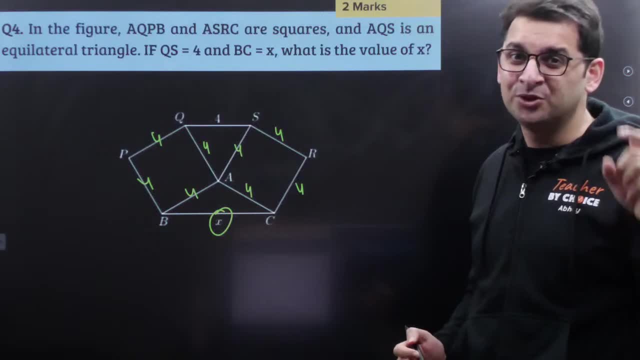 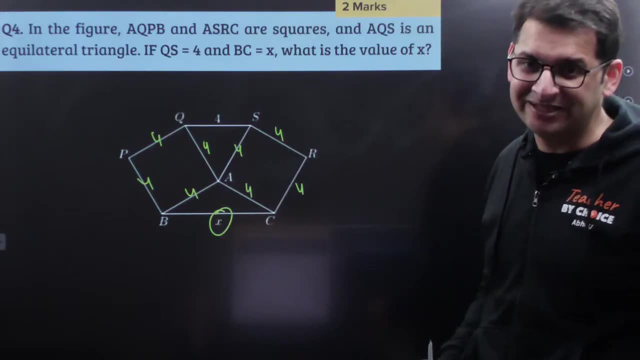 Amazing. this is the kind of speed which I want. So the speed of two number questions is the same. If you have practiced, you have confidence. this is the same speed. It should not take more time. As simple as that. 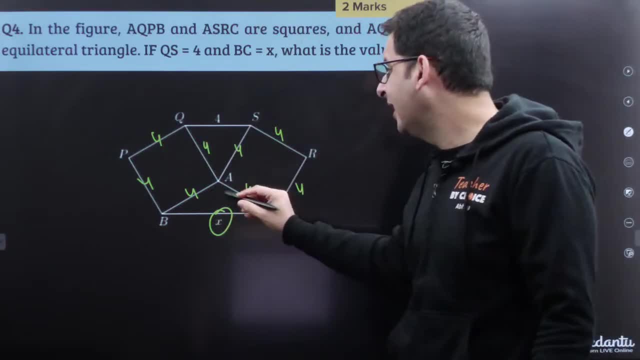 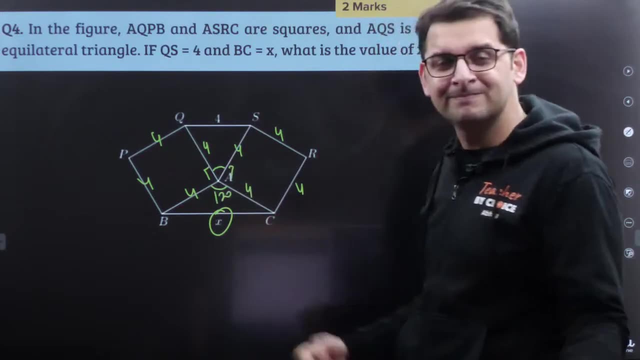 Cosine rule. as simple as that. You know these two numbers. If this angle is taken, then the question is over. So this is 60.. This is 90.. This is 90.. So this will be 120.. 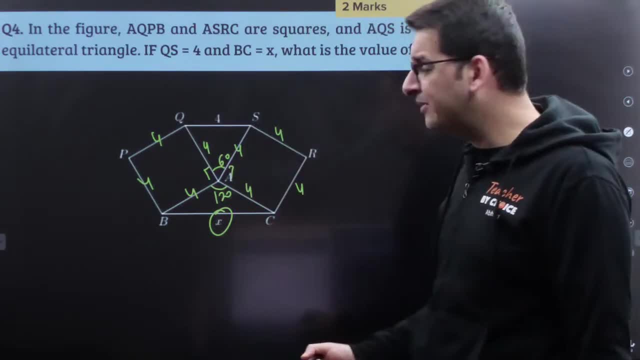 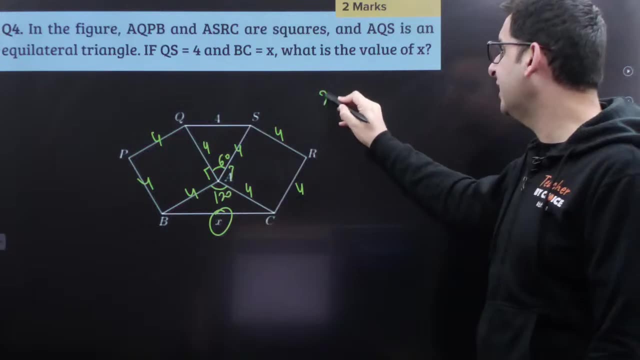 60.. This is 90.. This is 90. So total is 360.. So 90 and 90 is 180.. 180 is left 60 and 120.. So cos 120.. So what is the value of x square? 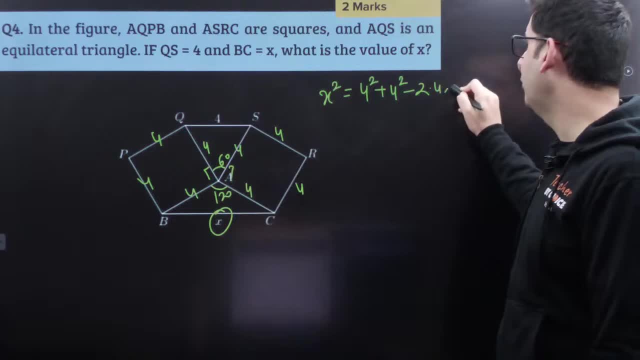 4 square plus 4 square minus 2 into 4, into 4, into cos 120 degrees. Is the question done: 4 square plus 4 square Cos 120 is minus half. Cos 120 is minus half, So plus 4 square. 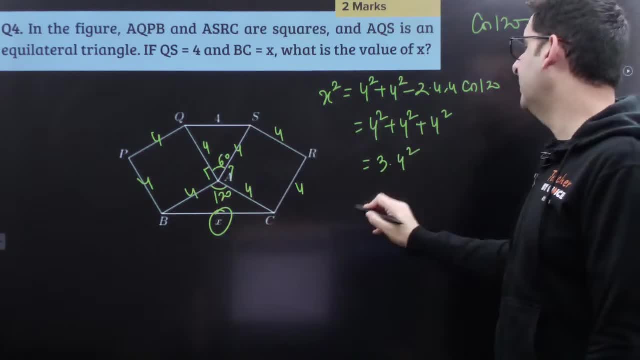 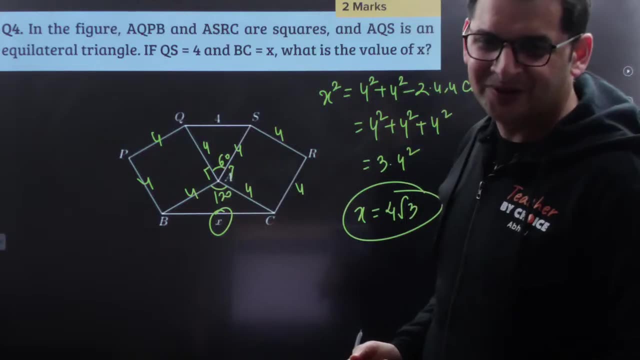 So 3 into 4 square. So what will be the value of x 4 root 3.. That is the right answer. As simple as that. Got it, Got it, Got it, Yes, Superb. I hope this is clear. 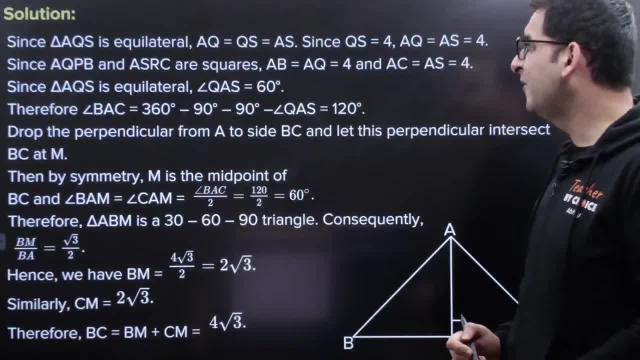 Moving on Next question is this Quickly? So I had already told you guys in the starting of the lecture: Today's question is going to be very cute, Super cute, Because I know that in the last week I have taught you a lot on the Inmo level. 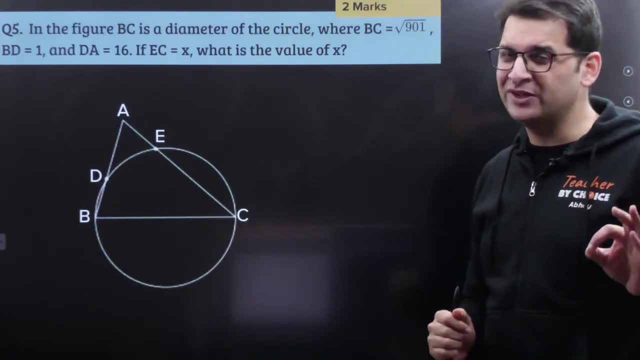 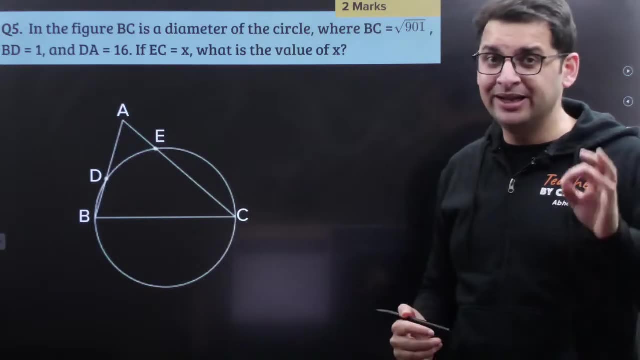 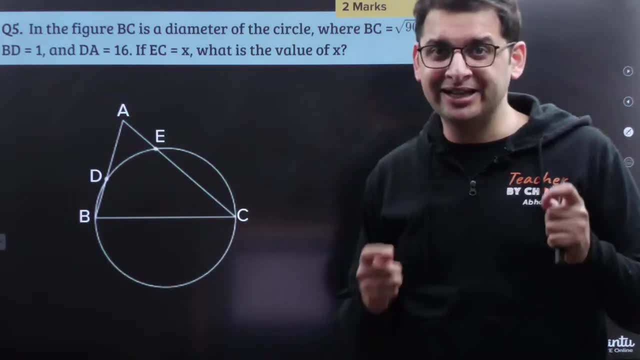 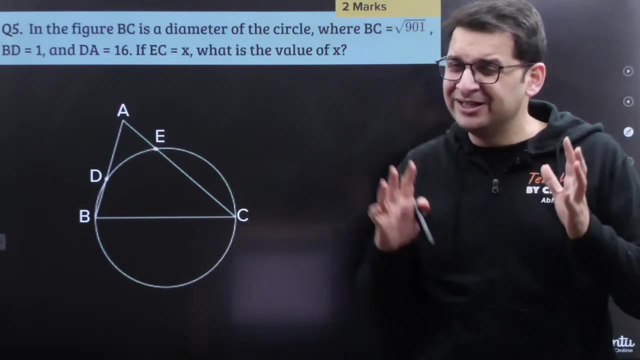 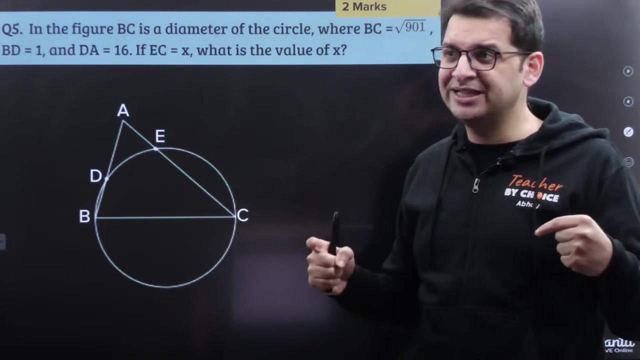 So a lot of people said and came to my telegram and said: bring some simple sessions forward on IUQM, because ultimately our target is to go for the certificate And this is our first attempt. So we decided that in this week we will be doing a lot of sessions on IUQM- only on basis. 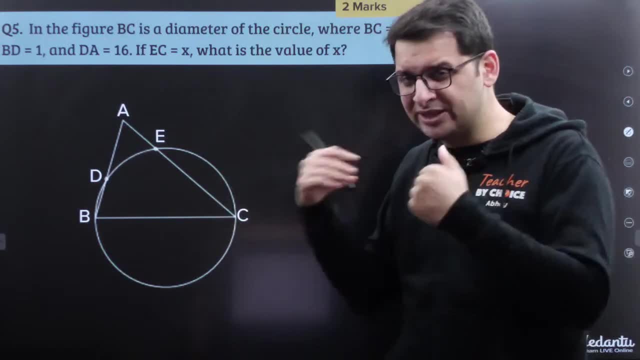 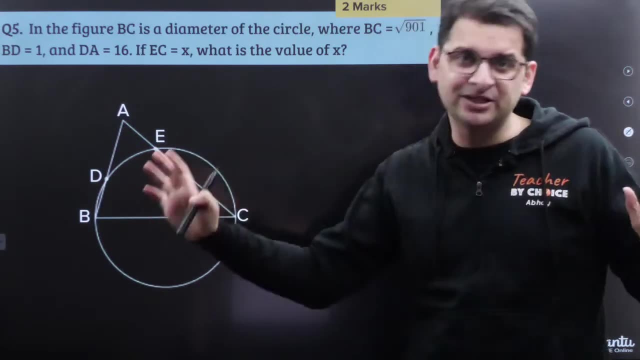 of IUQM. Today's session is mainly 2-marker, 3-marker May be in tomorrow's session there will be а lot 2-marker then if we have 3-marker, or So again. but IOCUM level sessions are going to be held this week. 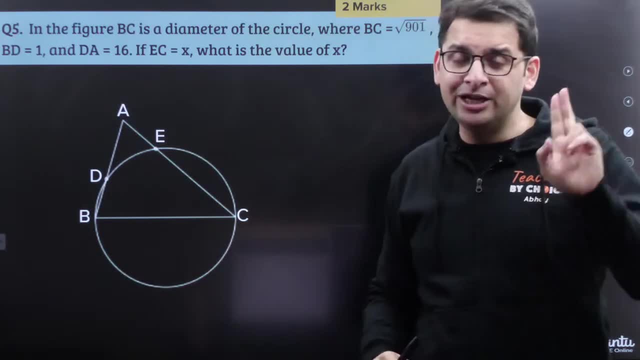 Along with that, what is there for the INMO people? There is a camp for the INMO people And secondly, IOCUM question of the day. Every day, a question is going to come, as I had promised, And we are still standing on that promise. 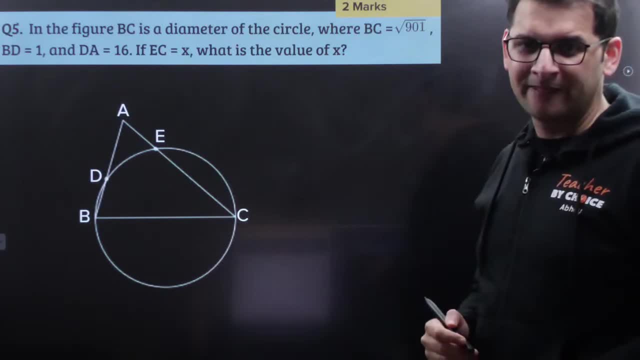 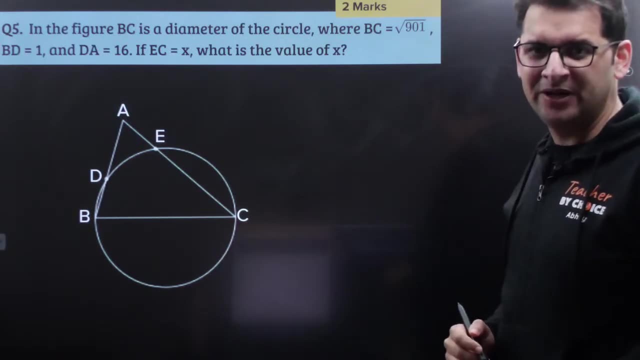 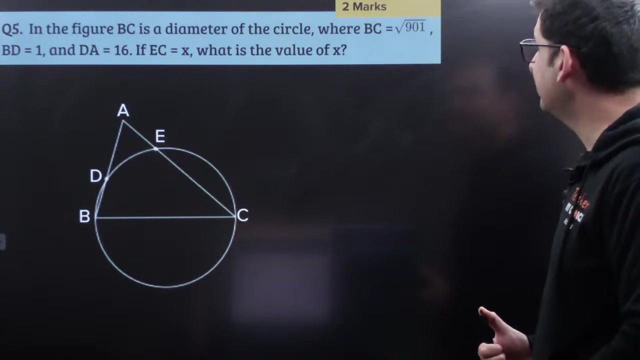 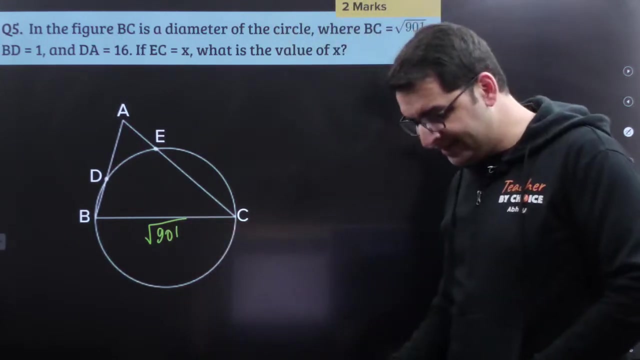 Got it. Come on, Come on, guys, Quickly, Quickly, Quickly. So in the figure, BC is the diameter of the circle where BC is root of 901.. So BC is root of 901.. BD is 1.. 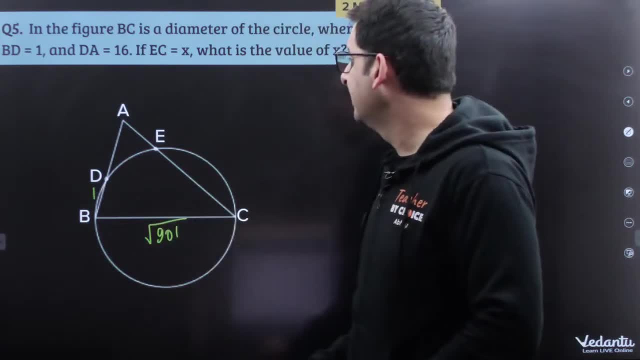 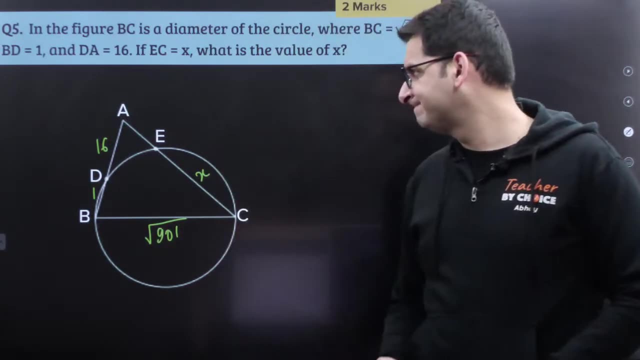 BD is 1.. So BD's value is 1.. DA's value is 16.. EC's value is X. What is the value of X? Someone is saying, sir, join B and E. You can join B and E. 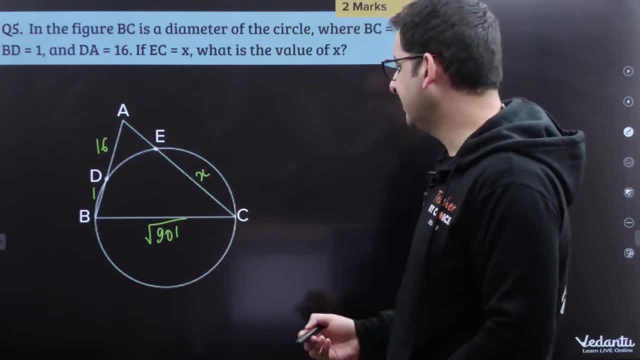 What is better than that? Join CD. I will give you a hint: Join CD. It is much better Because 901 is 1 here, So two sides were already known. So joining CD will be a little better. It will be a little better. 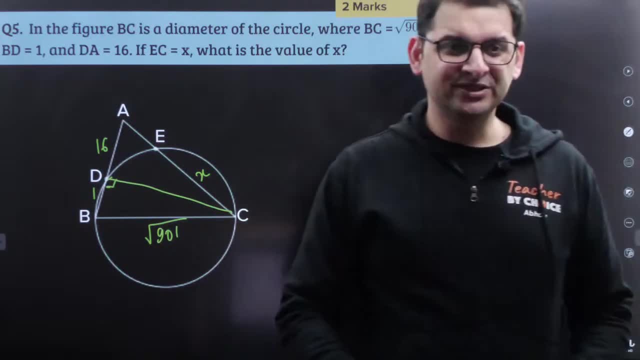 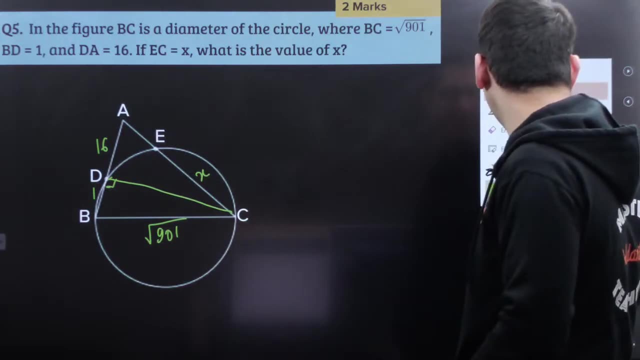 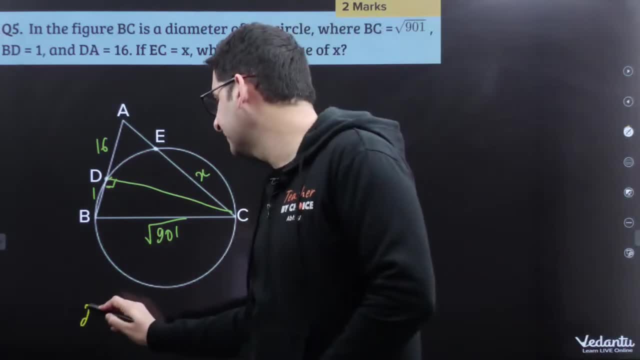 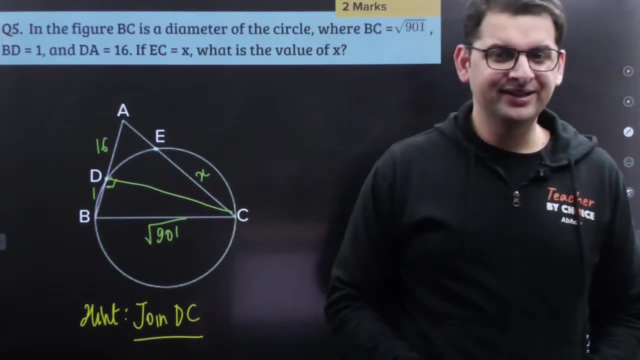 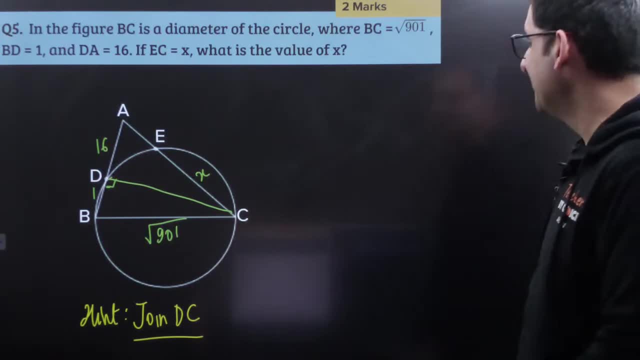 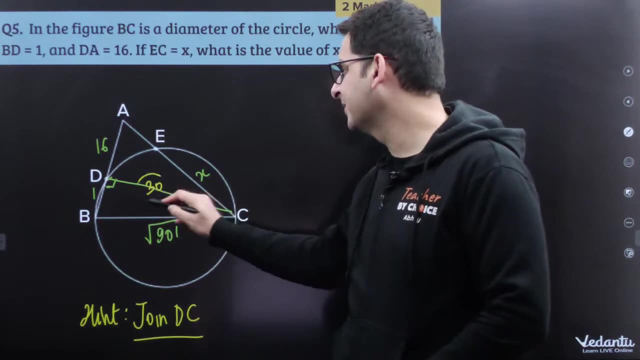 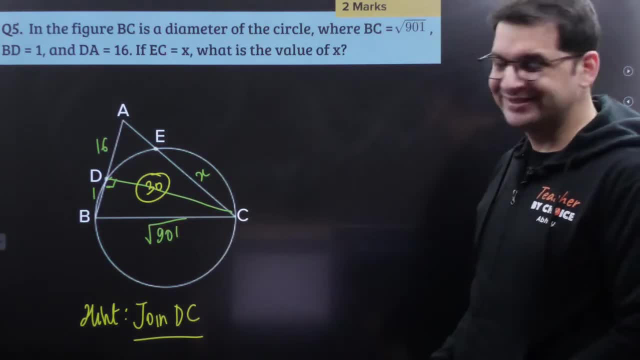 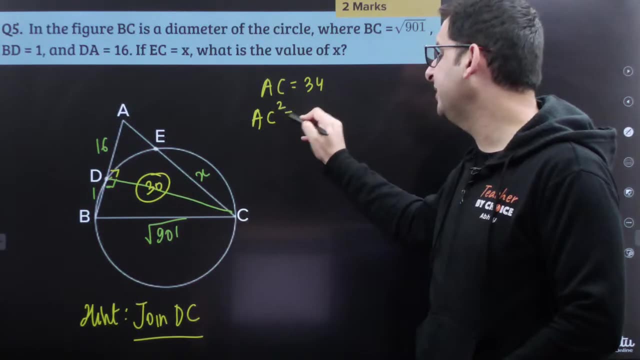 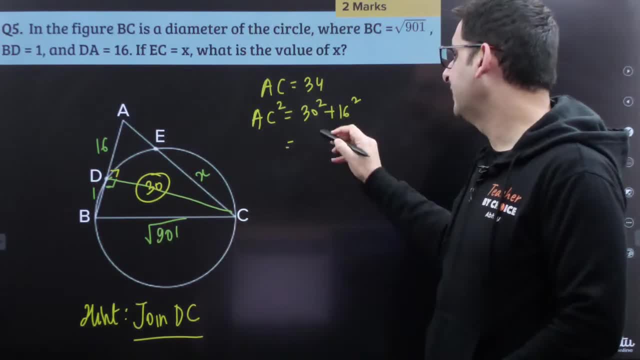 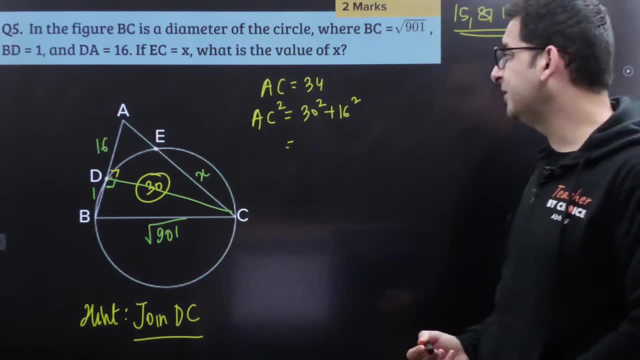 Join B and E. Join B and E, Join B and E. So this is a Pythagorean triplet of 15, 8, 17.. Pythagorean triplet of 15, 8, 17.. So 15 into 2, 8 into 2.. 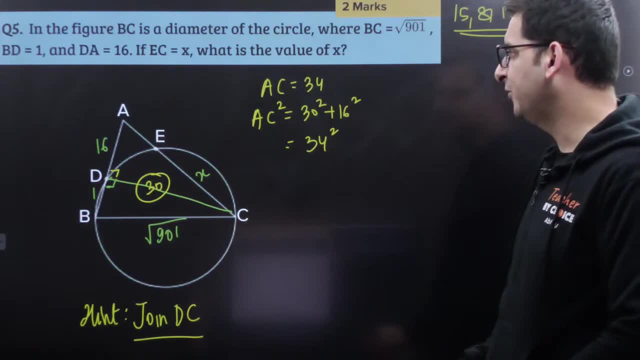 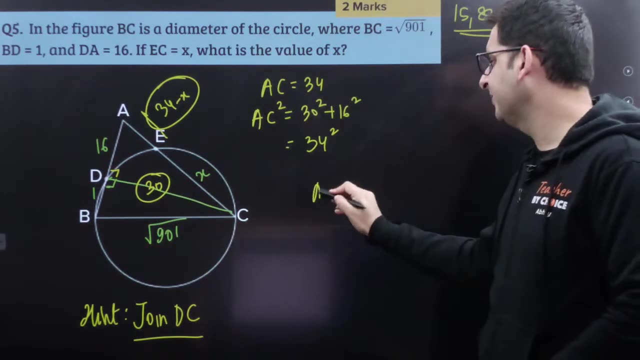 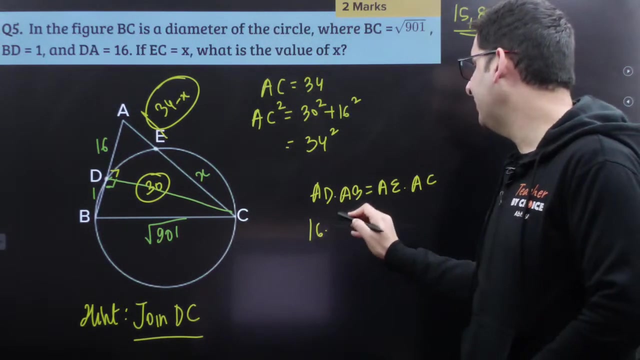 So it will give a square of 34.. So AC is 34.. If it is 34, then it will be 34 minus X. So can I say AD into AB is equal to AE into AC. So AD is 16,, AB is 17 is equal to AB is 34 minus X into AC is 34.. 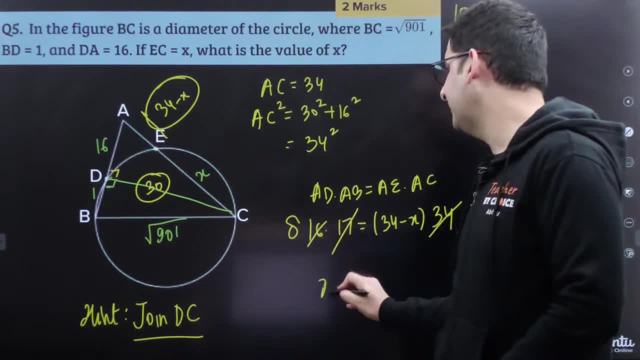 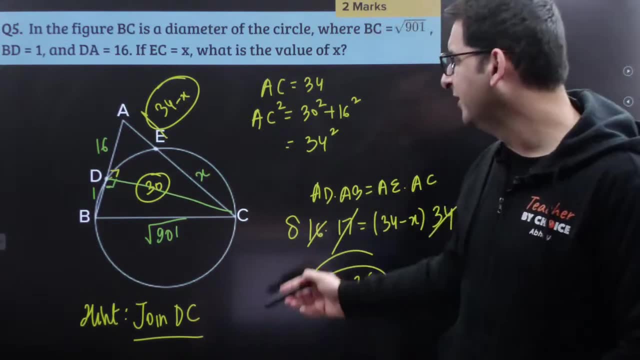 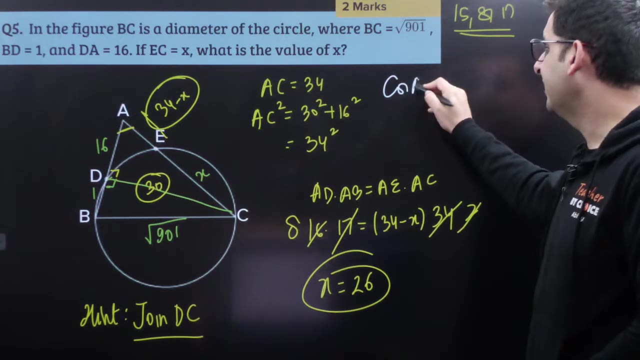 This will be the value of 2,, 8, X. 26 is the right answer. 26 is the right answer. Can we do COS as well? So a kid is saying: sir, apply COS A twice. So COS A is 16 square plus 17.. 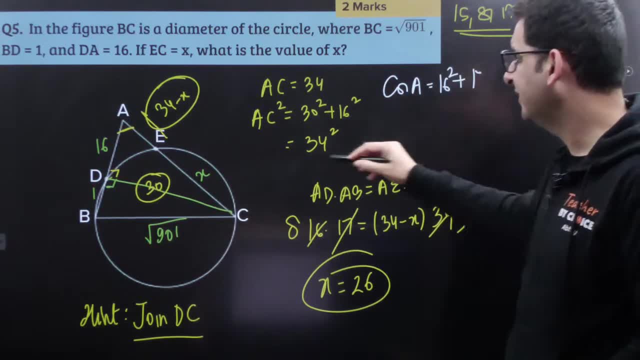 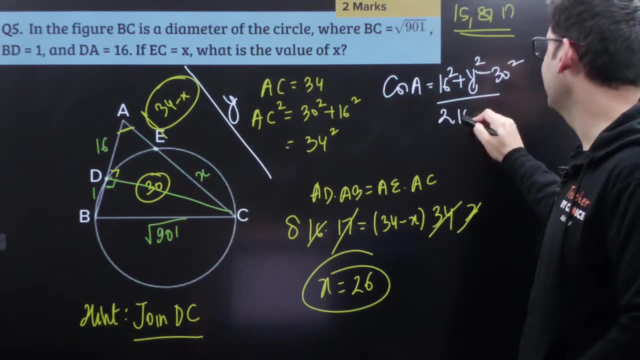 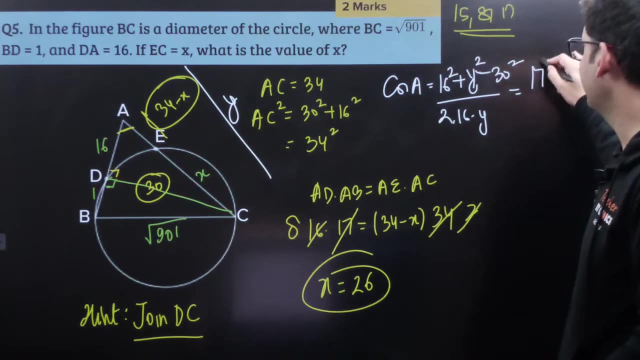 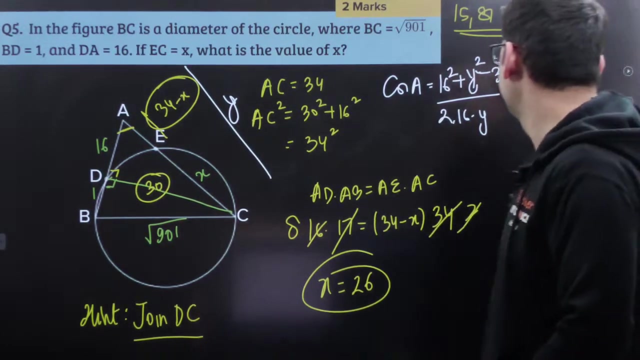 17 square 16 square plus. consider this whole as Y, Y square minus 30, square upon 2 into 16, into Y, And apply COS A in the bigger triangle. Apply COS A in the bigger triangle as well. So 17 square plus Y square minus 901 upon 2 into 17, into Y. 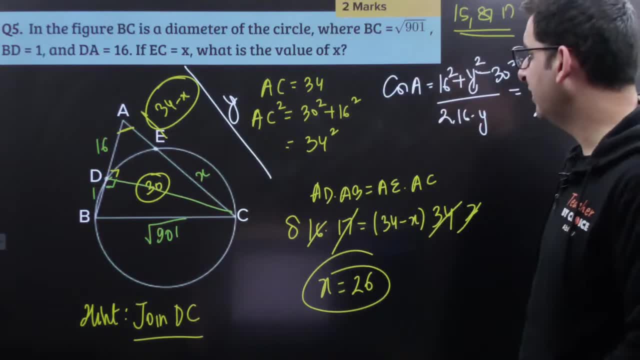 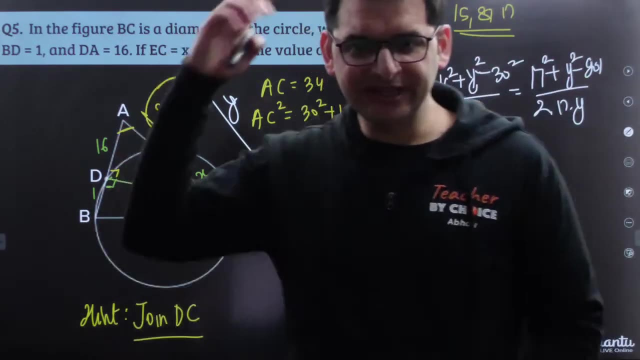 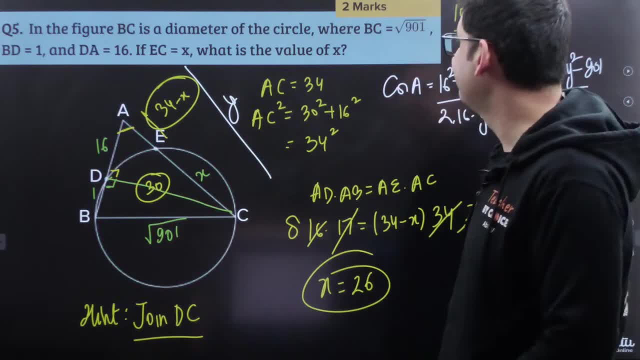 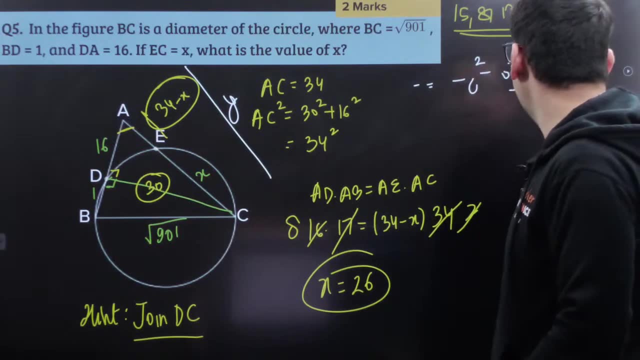 Super, Super. I hope this is clear. Instead of BC diameter, it will be 90 degrees here. Got it, Come on. Moving on to the next question: Very simple, simple question. The last two questions, the three number ones, are very good. 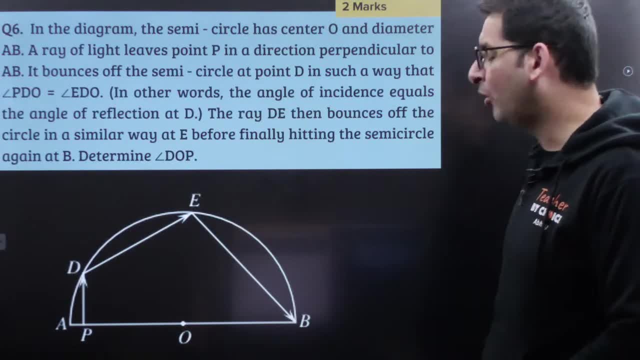 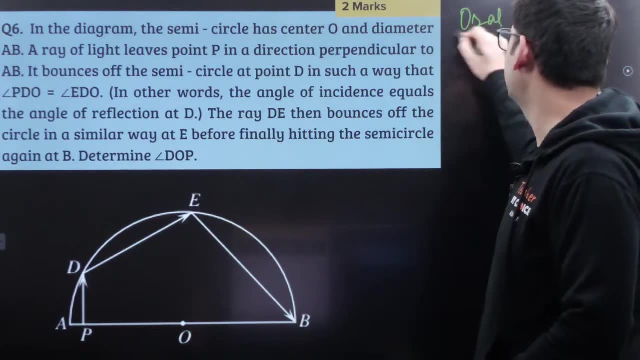 Very simple question. Now we move on to the next one. toes Quickly, we move on. The very simple question is: this should be oral. this should be oral. It should not be even there. It should not be even there. 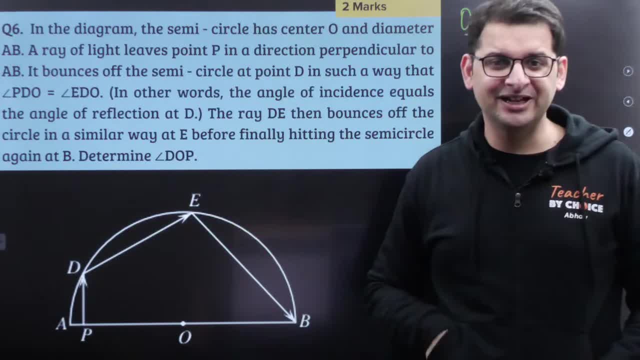 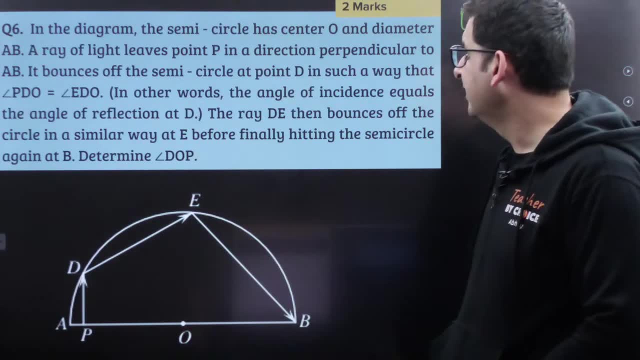 This is the last question of tomorrow. after that two to three number questions are coming Quickly guys, Quickly Quickly. So in the diagram of a semicircle has the center O, The center O of a semicircle, Diameter A and B? 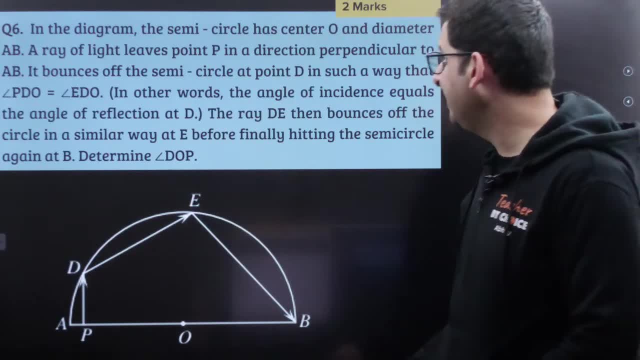 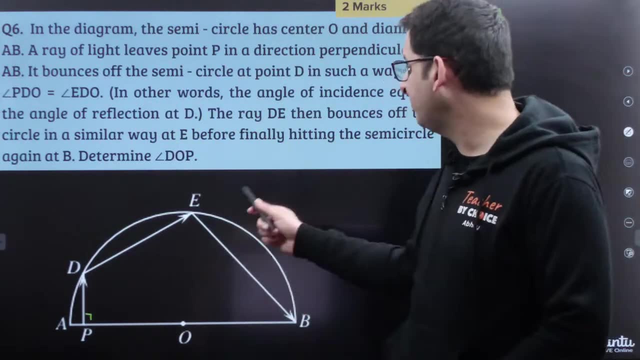 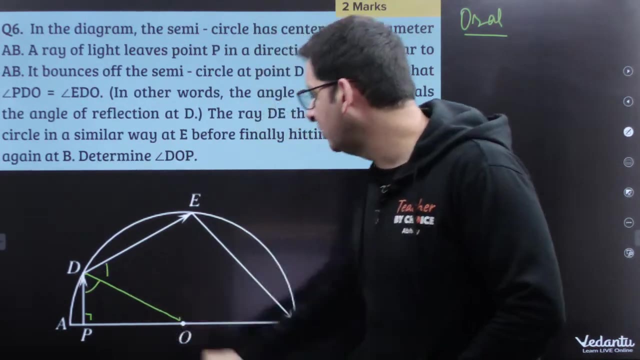 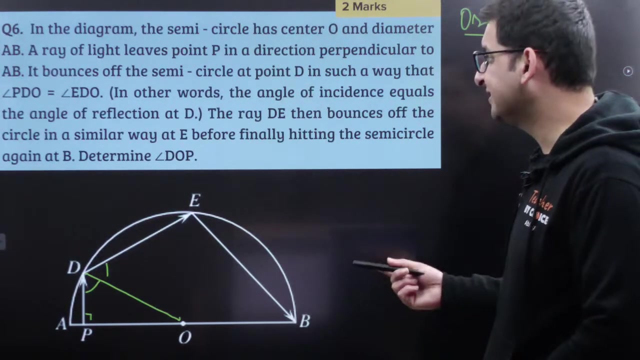 A ray of light leaves the point P in the direction perpendicular to it- perpendicular to AB- Bounces of the semicircle at point D in such a way that angle PDO is equal to angle EDO. The ray DE then bounces of the similar way before finally hitting. 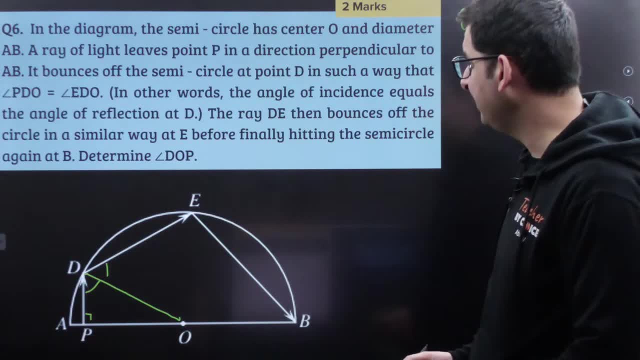 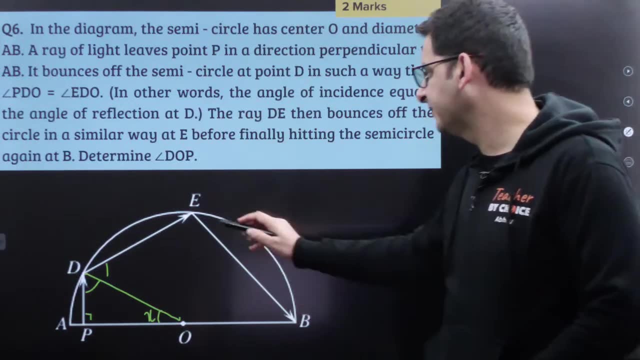 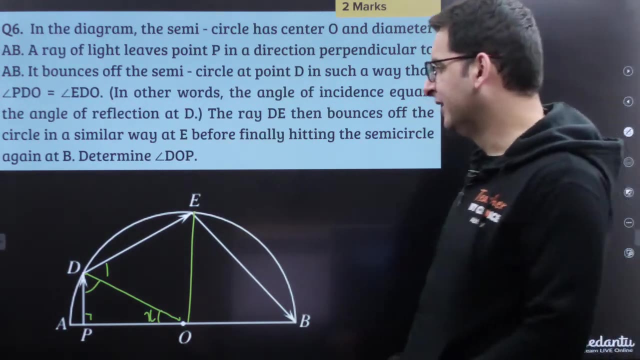 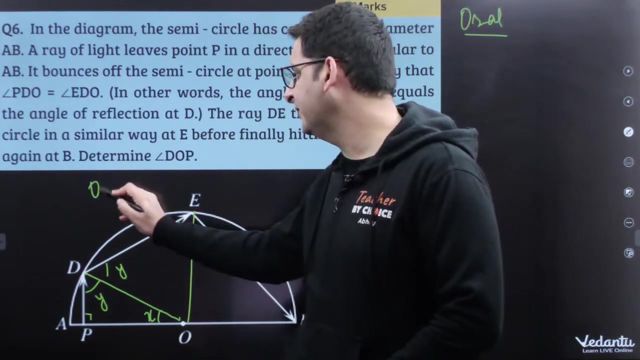 the semicircle at point B, determine the triangle, DOP, Determine the X. X is what we need to find Very simple. Let's say: this is Y, so this will also be Y. If this is Y, then this will also be Y, because OD is equal to OE. This is Y, then this is also Y. Angle of incidence. 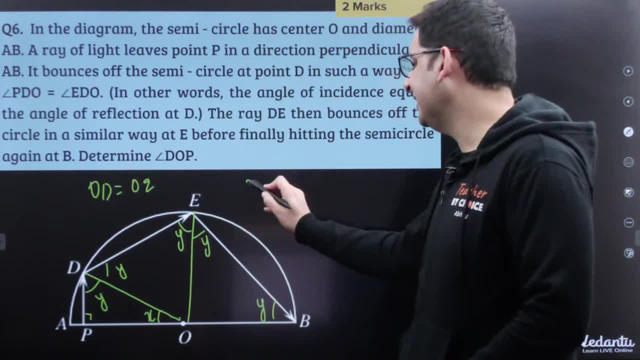 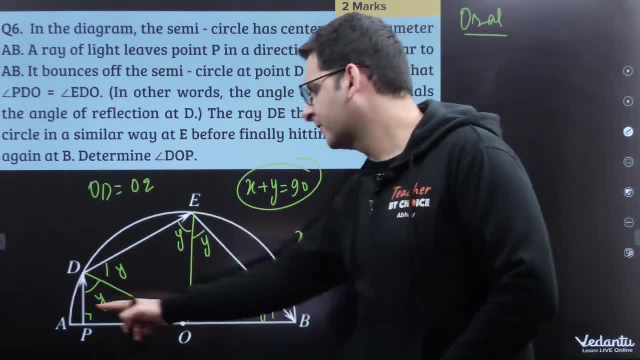 and angle of friction. This is Y and this is also y. And I know that x plus y is 90. So by doing angle chase you will get x directly Here. look at the quadrilateral. Look at the quadrilateral. 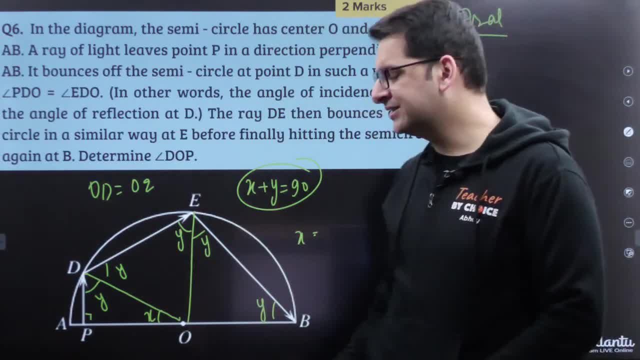 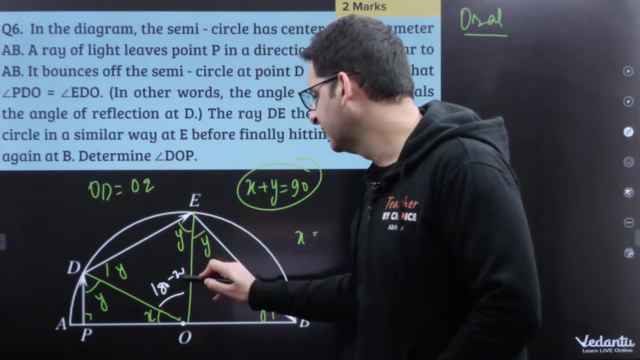 This plus this, plus this plus y is 360.. Or you can do angle chase here too. Here, This is 180 minus 2y. This is 180 minus 2y. Got it, Got it, Got it, Yes. 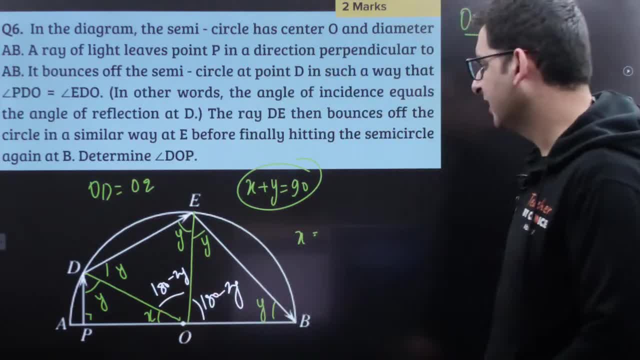 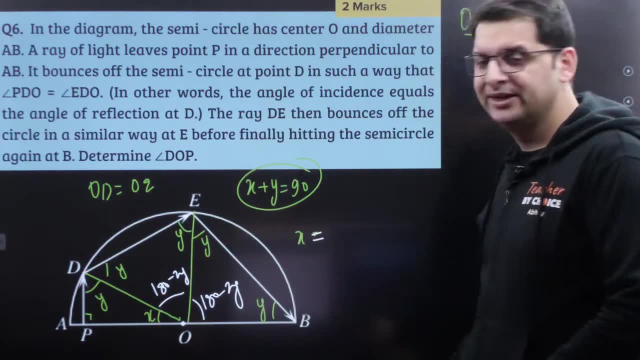 Got it. So this total angle is 180.. Or in this quadrilateral, the total angle is 360 degrees. Do anything You will get the value of x. as how much is x? Can you tell me, guys? Someone is saying 30.. 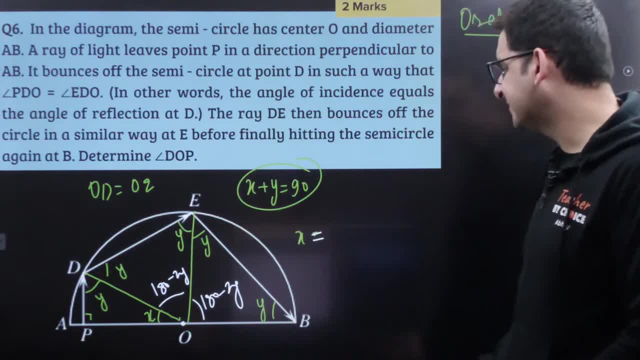 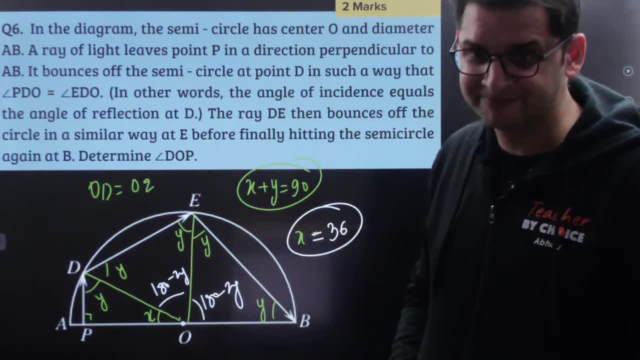 Someone is saying 36 now. So as you find x 36.. 36 will come, guys, This will be 36.. This will be 36.. Did you all get this? Did you all get this? Yes or no? 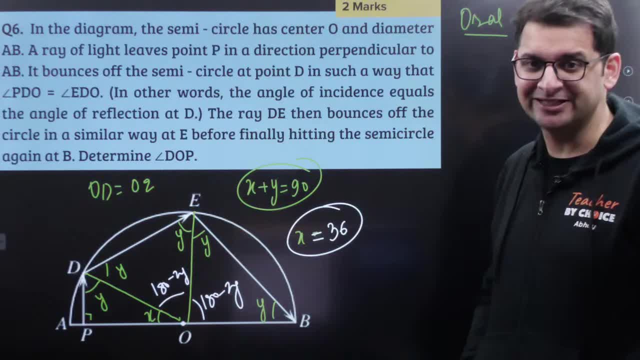 It will not be 30. It will be 36. 36. Yes, Navya Akshat. Yes, Tanmay. Amazing Shashwat, Super Got it. everyone. Did you all get this guys? 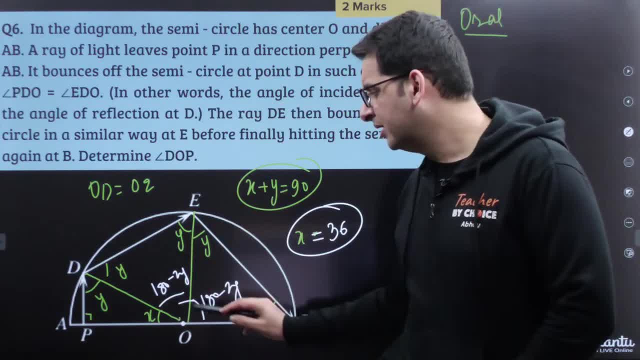 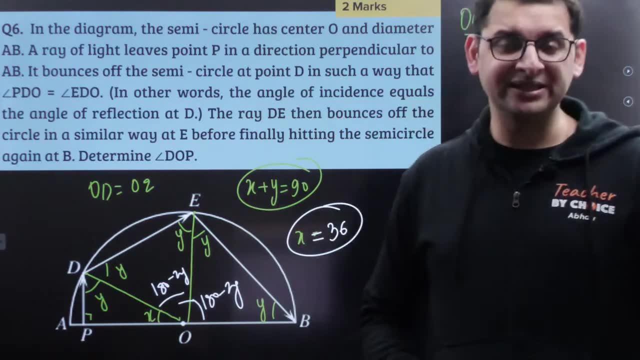 Did you all get this? Either do this total angle here with 180.. Or this quadrilateral P-D-E-B Quadrilateral, Do angle chase. Total angles are 360 degrees. Got it everyone? Did you all get this? 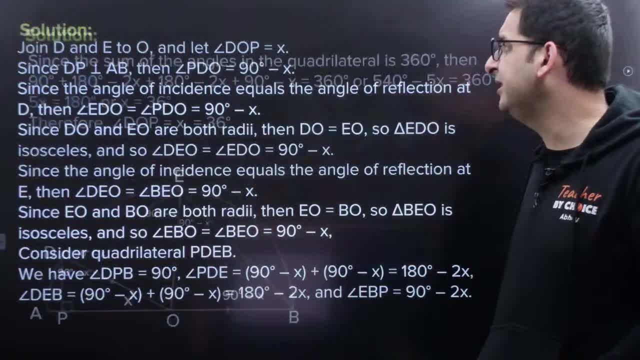 Yes or no? Fastly. So two markers done, Moving on to some three markers, Let's see if you are able to crack this. This is a good question, guys. This is a good question. This is a good question, guys. 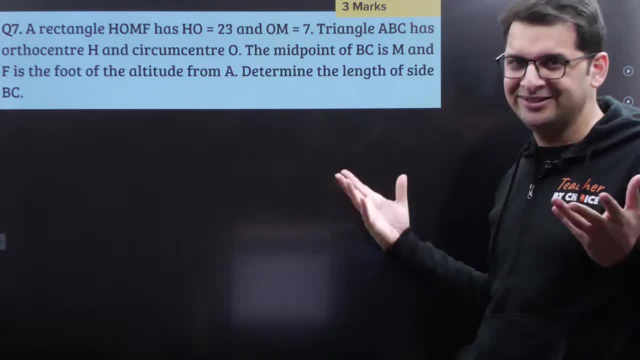 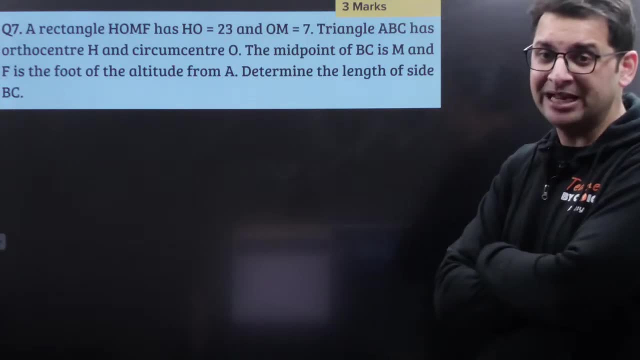 It seems like a simple property. If you know the property, then it is a question. If you don't know, then it will take some time. So, rectangle HOMF, It may take time to make a diagram, So I will give you some time, guys. 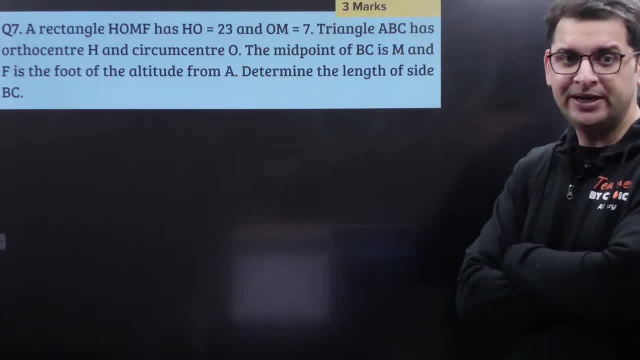 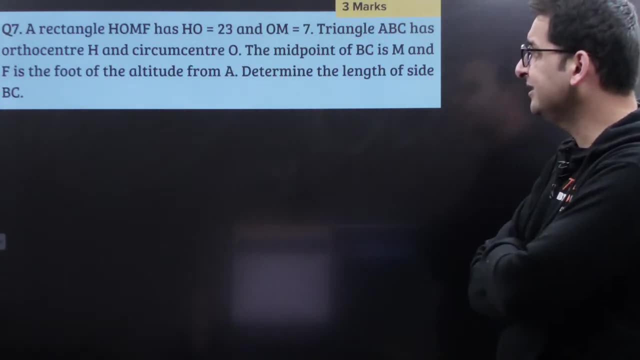 I will give you some time. I will give you some time to think over it. Rectangle HOMF has: HO is 23,, OM is 7.. The triangle ABC has also center H, circumcenter O. The midpoint BC is M. 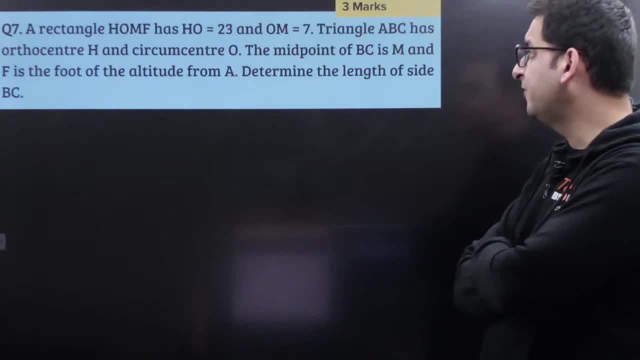 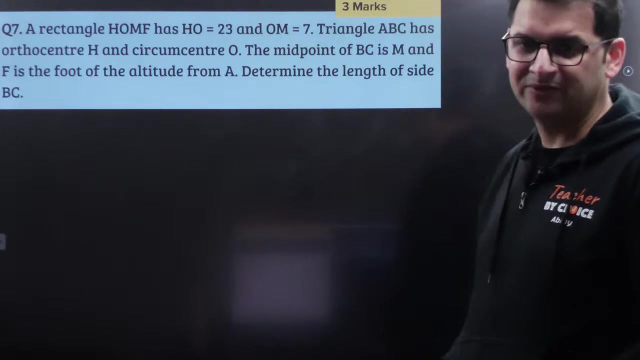 BC has midpoint M F is the foot of the altitude from A. So HOMF has H O M F. Determine the length of side BC. Tell me the length of BC. Tell me the length of BC. Yeah, I will give you some time for this one. 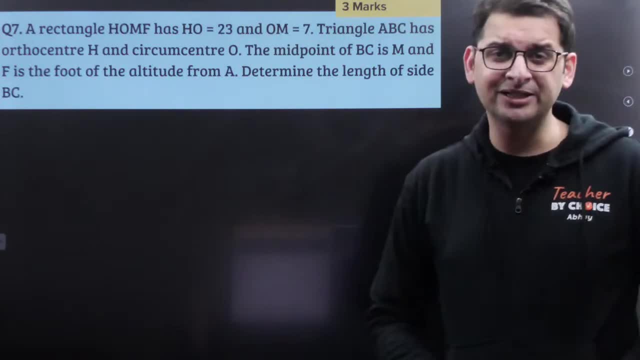 Coordinate for IOQM. But Pranav coordinate most likely is not going to come this time Because, since they are going to select very few students, so again they will be checking hardcore number theory, hardcore geometry, hardcore combi and so on. 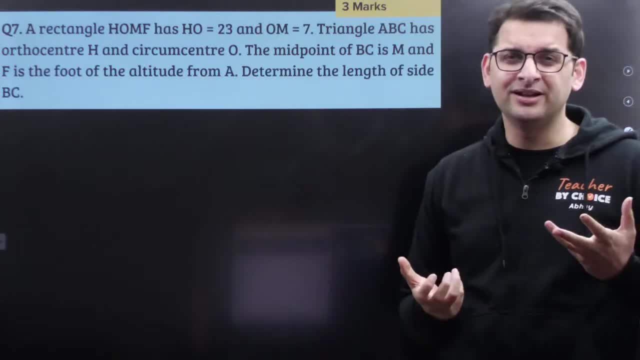 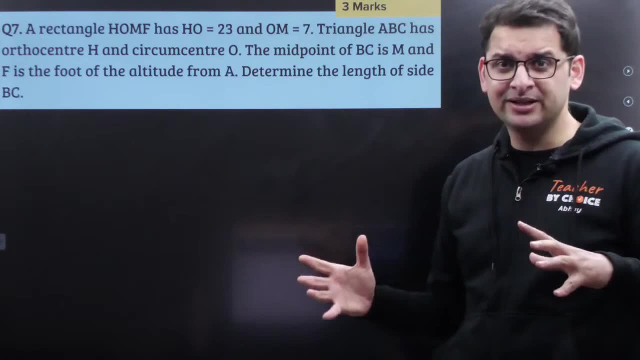 So I don't think there will be any question of combi And for combi. of course a little advantage is there for 11th class students because state lines on circles questions, Sometimes without geometry and coordinate geometry, can be done. 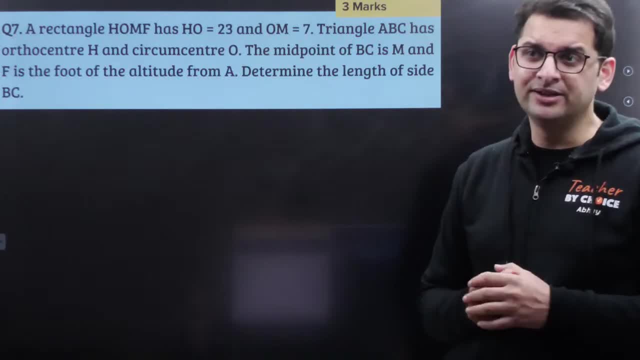 But I don't think it is going to matter much this time. So again, we are not doing coordinate geometry. Concentrate on geometry. Do it on number theory, Do it on algebra, Do it on combi, Do it on combi. 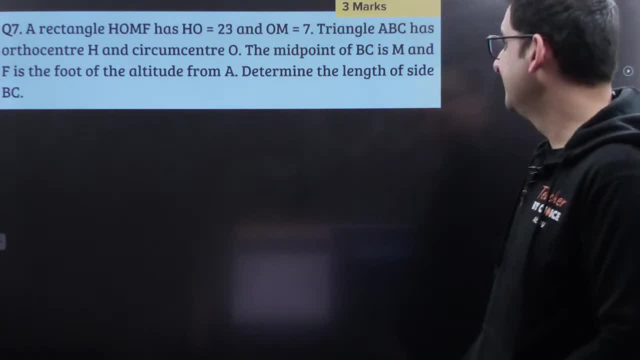 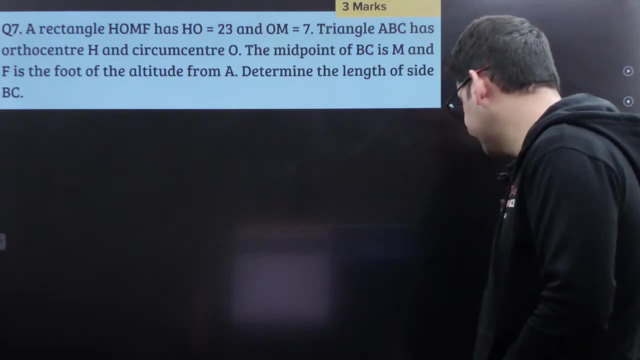 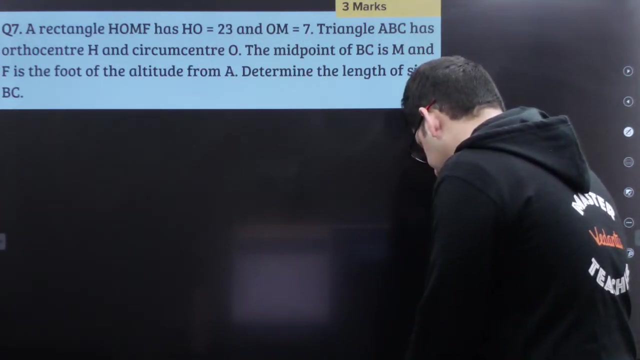 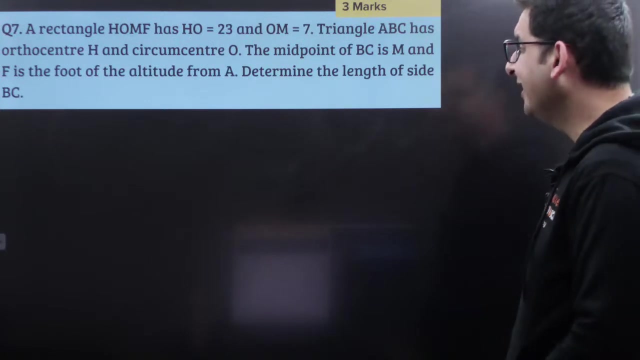 That is it. What do we do here? What do we do here? Diagram- to tumhe banana hai. Diagram maine banaka diya, toh question bahut asan ho jayega. Diagram: agar maine banana diya, toh question bahut asan ho jayega. 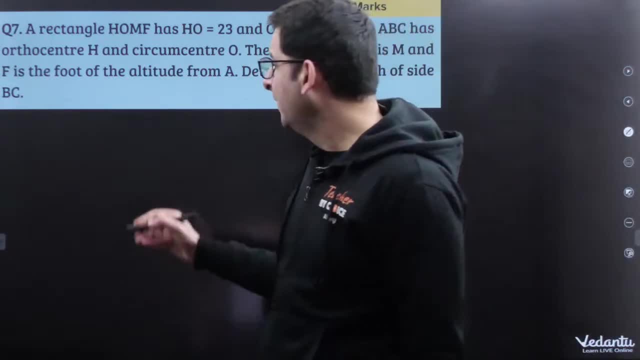 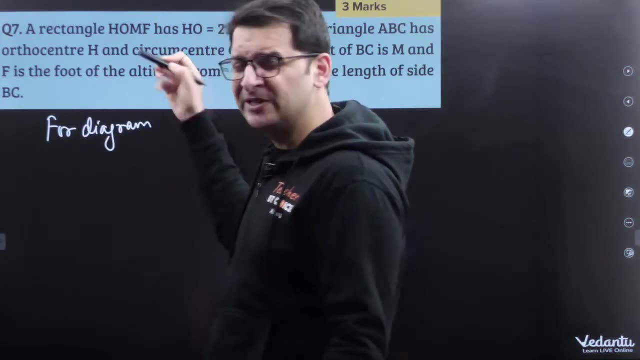 So how do we start? Should we Chalo? ek baat batao: Agar diagram banana hai For diagram, For diagram, Agar is tana ka scenario diya ho, soch ke batao, Should we start? 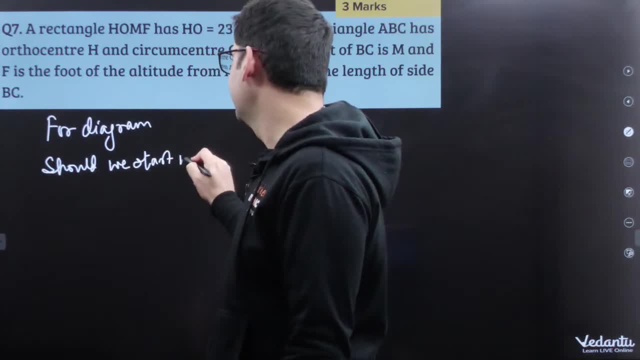 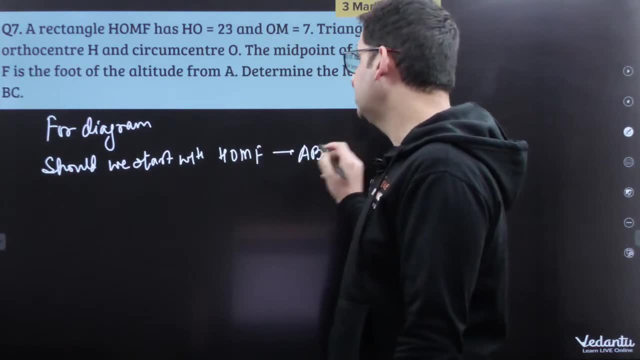 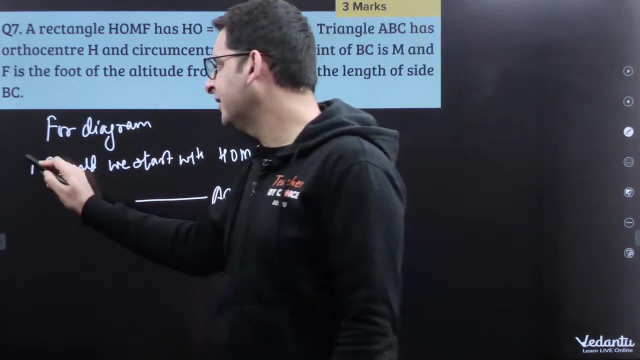 Should we start with HOMF and then construct ABC, Or should we start with ABC and then construct HOMF? Scenario 1, scenario 2.. Kya karna chahiye? Sochke batao, Sochke batao. 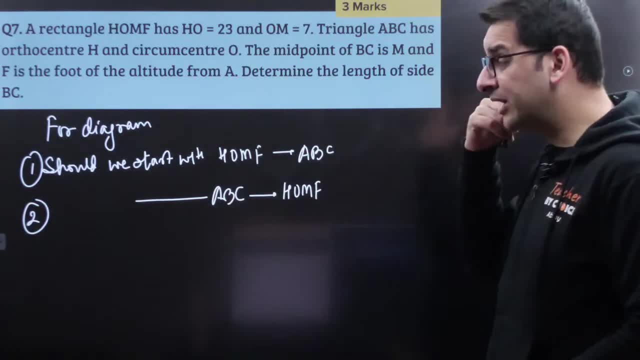 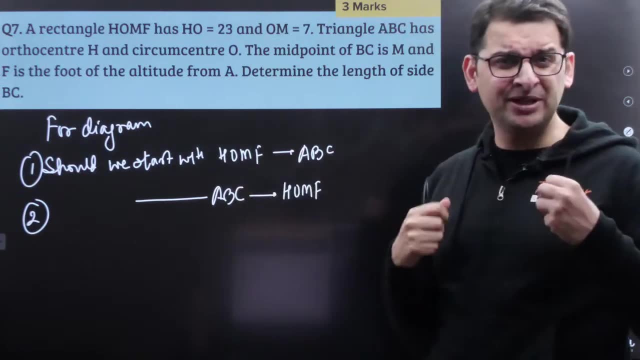 Kya hume iss tana ke question mein HOMF banana chahiye, rectangle banana chahiye aur phir ABC banana chahiye. Is it going to be easy? Ya, phir triangle ABC banao aur phir rectangle. 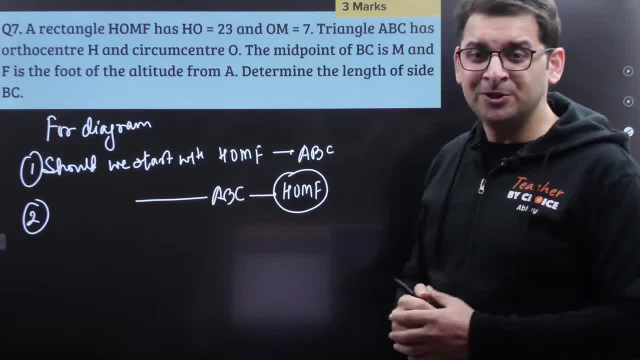 Yeh toh rectangle hi hai, na yaar. Yeh toh Toh jo cheez banani asan hai, Rectangle banana asan hai. Mujhe toh bas perpendicular lines jodh nahi hai. ABC bata nahi, kis tana ka rectangle hai. 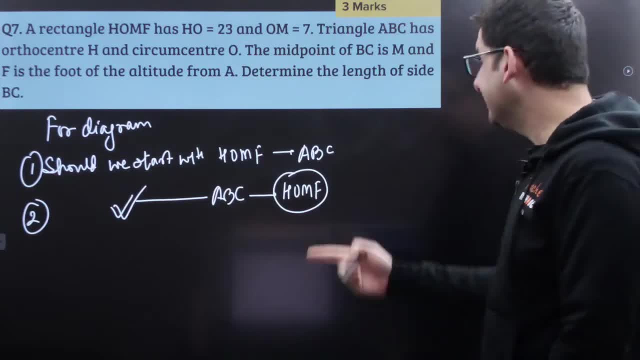 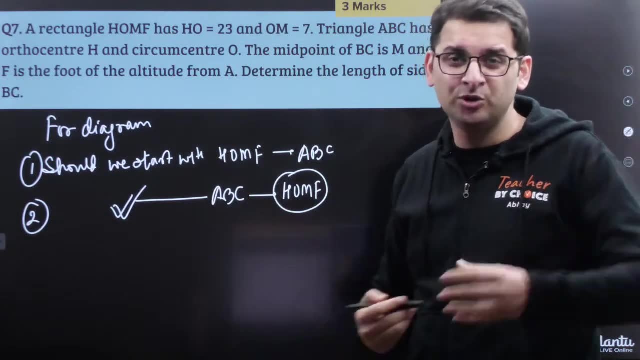 So again, This makes more sense. This makes more sense, This makes more sense. Dekho, Agar hum rectangle banadi hai, HOMF Aisa nahi bol raha hai ki question mein ABC nahi bana pao ki it is going to be difficult. 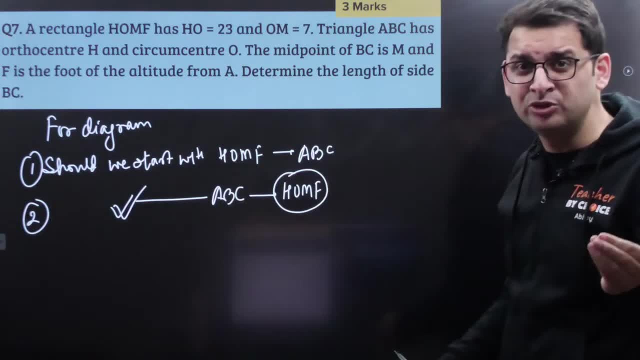 But ulta karna zyada aasaan hai, Because HOMF toh rectangle hai na, Mujhe toh sirf connect karna hai, Perpendicular lines connect karna hai. That is it. So again Triangle banao. 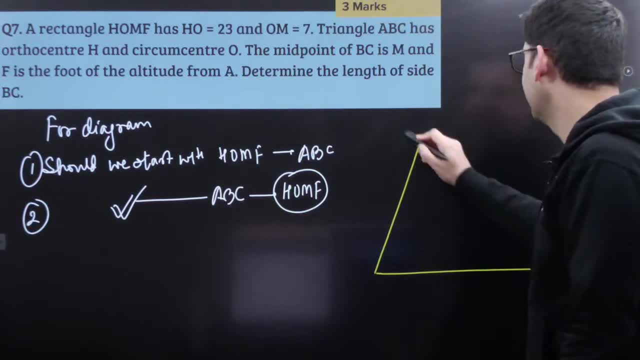 Let's say, triangle is ABC Bana liya. This is A, This is B, This is C, Ab. dekhte hai, yaha pe, kya, kya hai. Midpoint of BC is M. Toh, yeh, M. 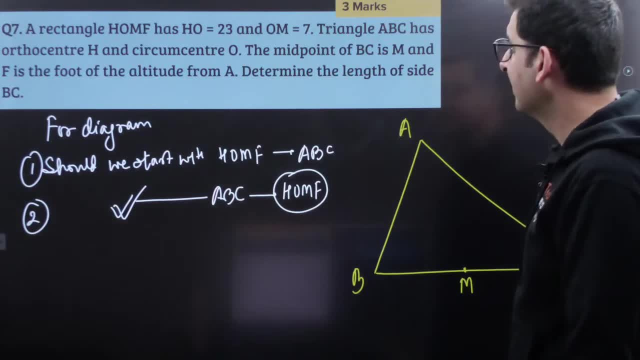 Done ho gaya ji HOMF rectangle hai. Achcha isko orthocenter H hai, Orthocenter iska H hai Toh orthocenter kuch aisa hota hai, Orthocenter iska kuch aisa hota hai. 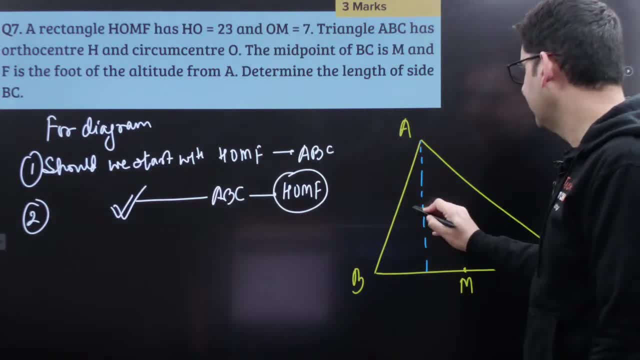 Toh yaha par kahin H hoga, Yaha par kahin uska H hoga. HOMF, Achcha, O kya hai? Circumcenter, Circumcenter. matla, pehle iska circle bhi banaate hai. 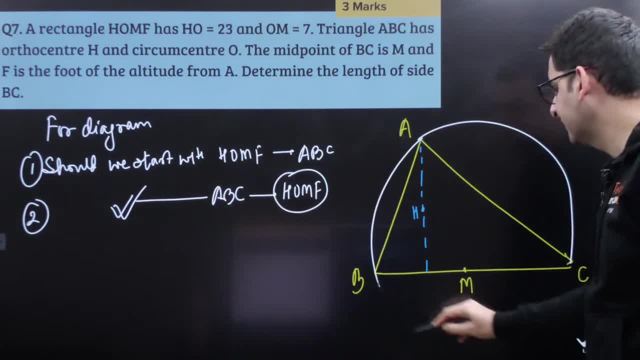 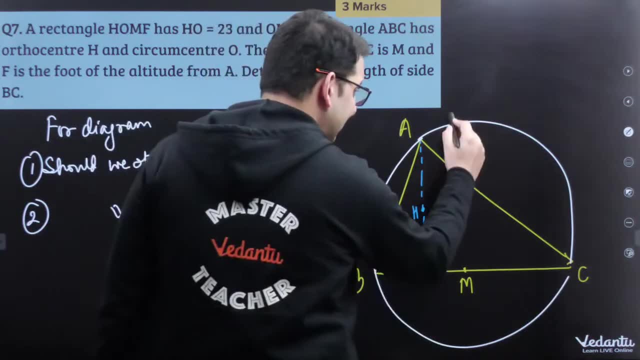 So this is going to be the circle And circum circle. dekho Dihansa, dekho Sarkal banta kese hai perpendicular bisector se. So again perpendicular bisector: yaha se, yaha se. Toh, guys, dekho HOMF rectangle hai. 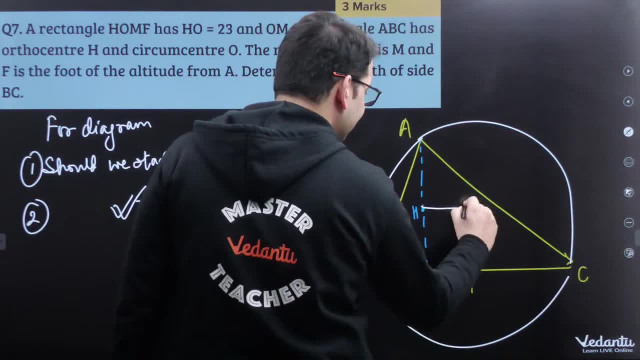 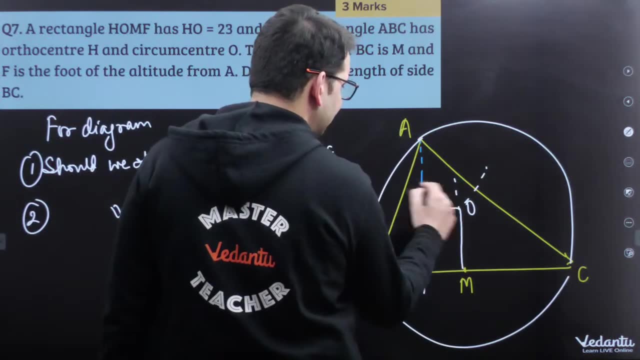 Toh kena say: O aisa kuch banega, F, kuch aisa banega, Kuch aisa, Kuch aisa Yeh perpendicular bisector. Yaha se perpendicular bisector kuch aisa raha hai. 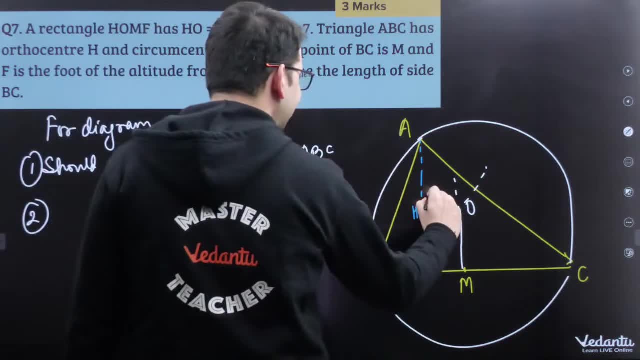 Mota mota kuch is tarike se rectangle banne wala hai. Achcha, HO ka value 23 hai And OM ka value 7 hai. Halake rectangle sahi sa nahi bana, Because this should be greater. 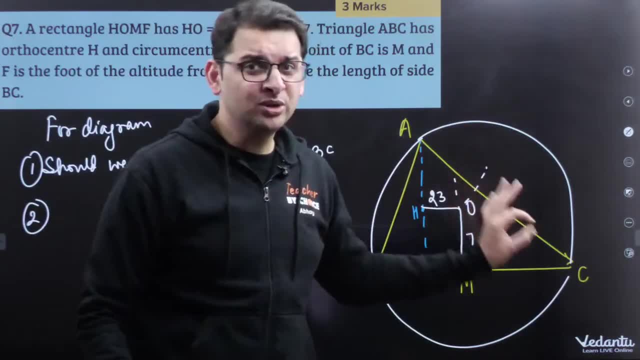 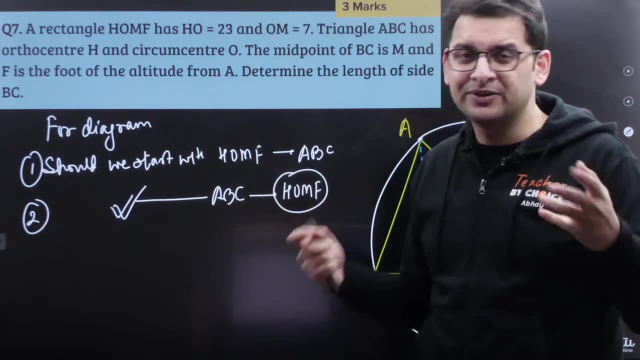 As per the figure. But koi baat nahi, Mujhe idea toh lag gaya. So again, it is always easy, guys, Jo simple figure hai na Rectangle, yaha pe simple figure, tha Rectangle, tha Triangle, pata nahi kaise hai. 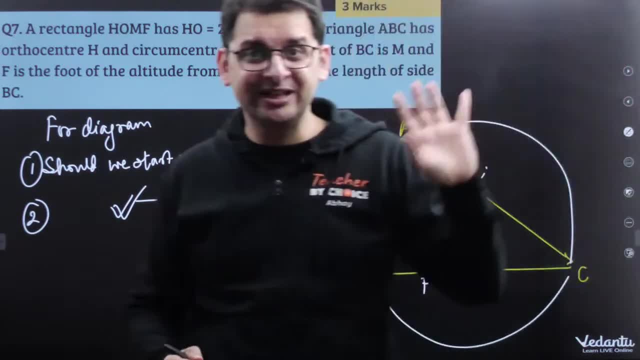 Toh jo simple figure hai, usko baad mein Is tarah ke question hai. Baad mein koshish kiya karo, Connect karne ki Woh aaraam se ho jaati hai, But agar rectangle safe mein. 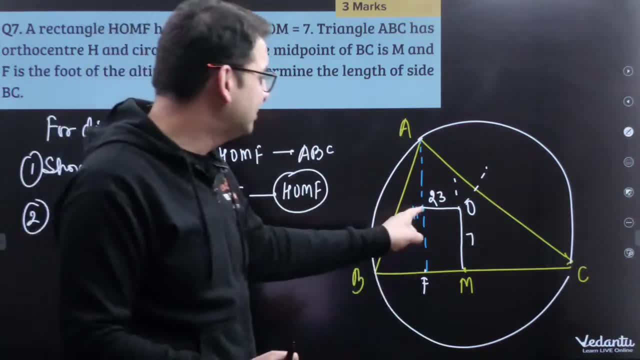 Main triangle banane ki koshish karna hai. It would have been very difficult Ki agar edge pata hai, Tumhe altitude draw karna. padega, Pura ka pura. It is going to be really difficult. Got it everyone. 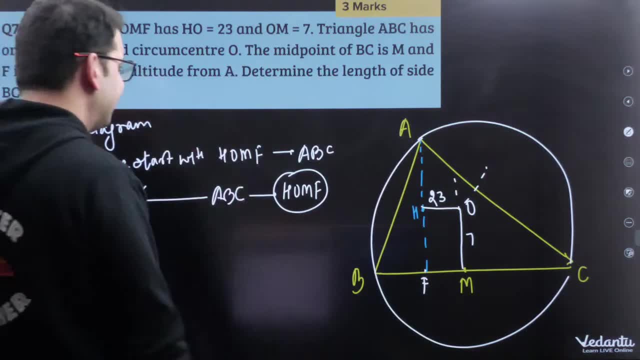 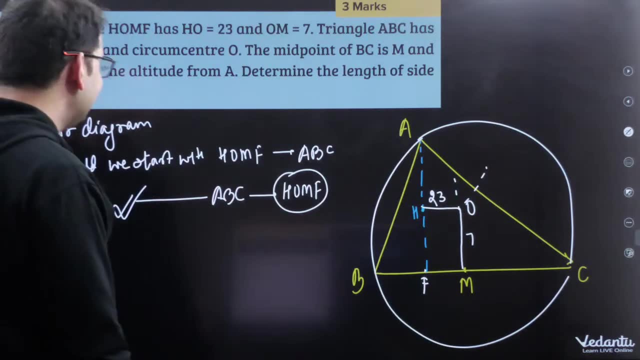 Yes, Super, Toh, yeh ho gaya. Yeh hamara figure hai Acha Yaha par. F is the foot of the altitude. draw mein Toh. this is the rectangle Which is already known. Find the length of the side BC. 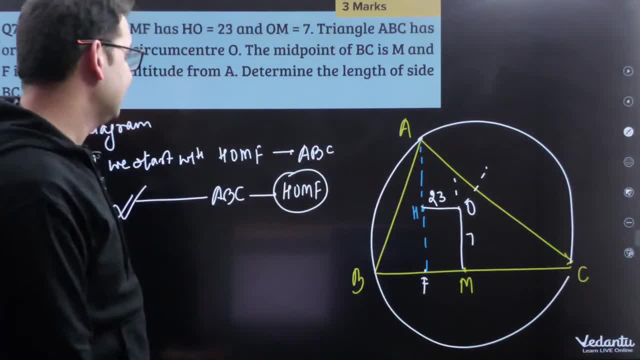 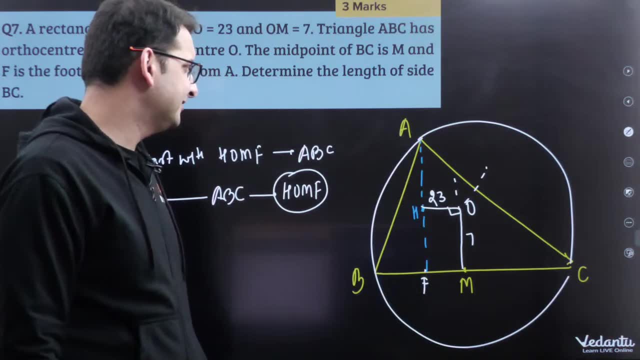 BC ka length find karna hai. These are the only two things which are given to us, And the fact that Yeh, Yeh hai Kya kiya jaye, Kya kiya jaye, guys. What do we do? 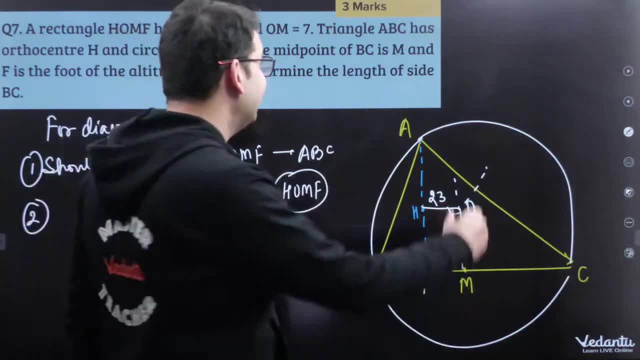 Ab yaha pe bahut sari cheeze hai, Jahan se main explore kar sakta ho. One is Ek cheez explore. HO is parallel to BC. One is: HO is parallel to BC. HO is parallel to BC. 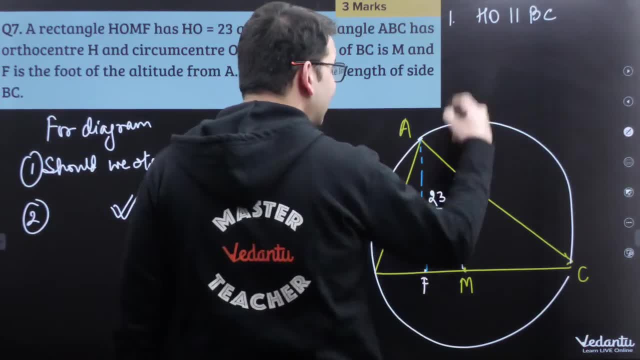 HO is parallel to BC Aur, agar tumhe yaad hai, Yeh jo OM ka value hota na. This is R cos A, R cos A Aur HF is 2R cos B, cos C. HF ka value 2R cos B cos C hota hai. 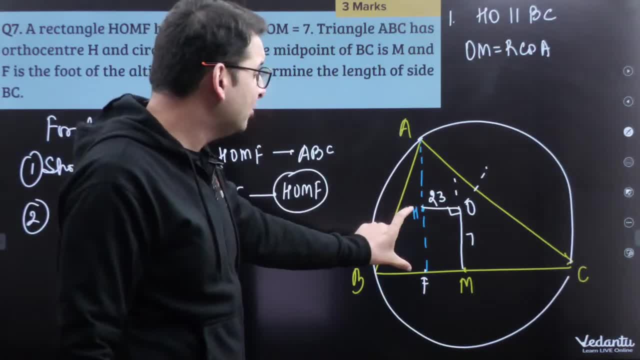 HF is 2R, Agar yeh pata hai, Nahi pata hai, Toh chhoda hai isko. Toh. agar yeh nahi pata hai, Toh yeh dono ko equate kar sakte ho tum. 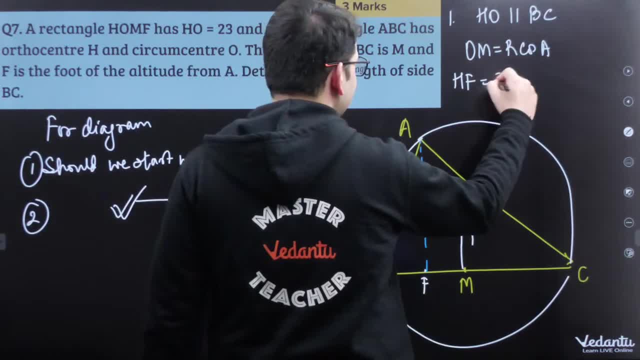 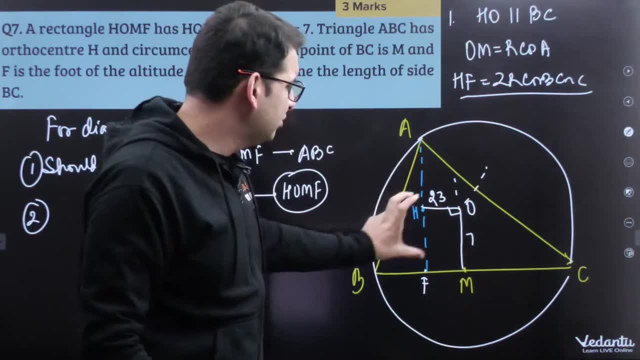 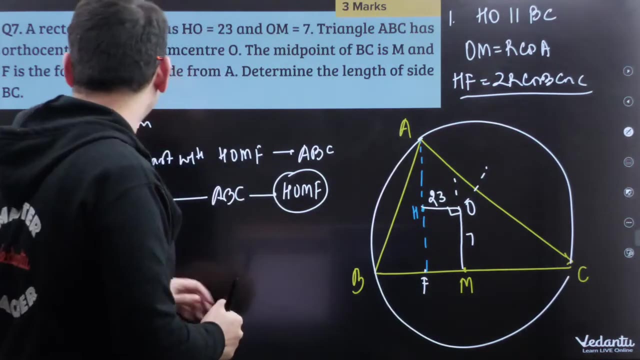 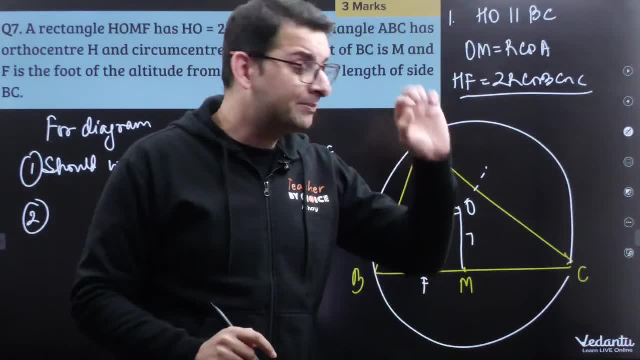 What else can we do? Ek aur property hodi, I don't know. Yeh wali property mainne bohot bar batahi hai YouTube sessions me batahi chuka hum Bohot saare questions ke andar. 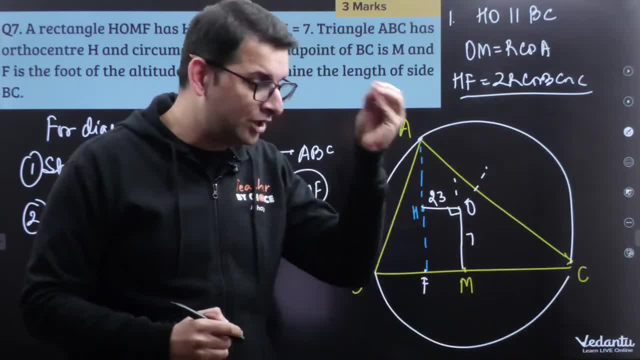 Yeh wali property hum regular Vedanta Olympiad School ke sessions me toh bata hi hai, Iocam camp ke andar humne bohot saare questions kar vayana hai. Yeh property batahi hai, Aur yeh bohot important property hai. 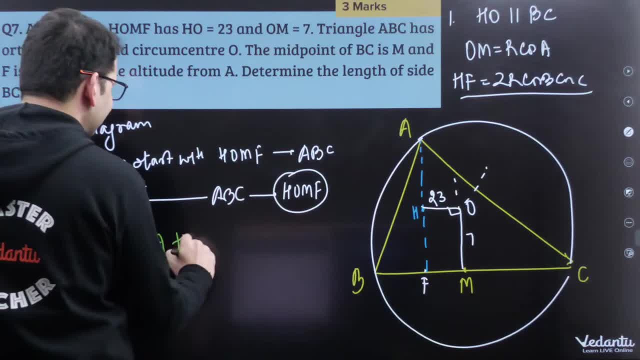 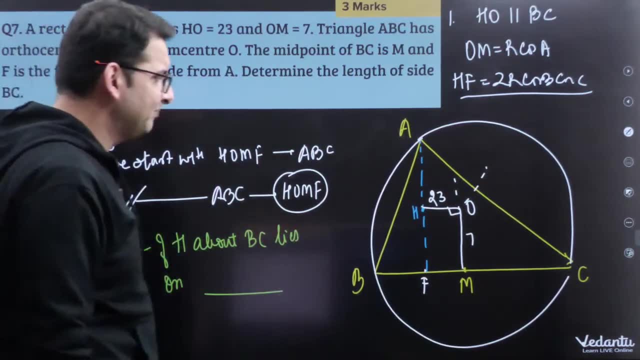 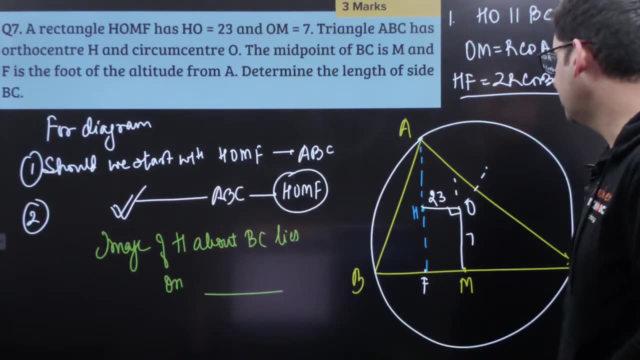 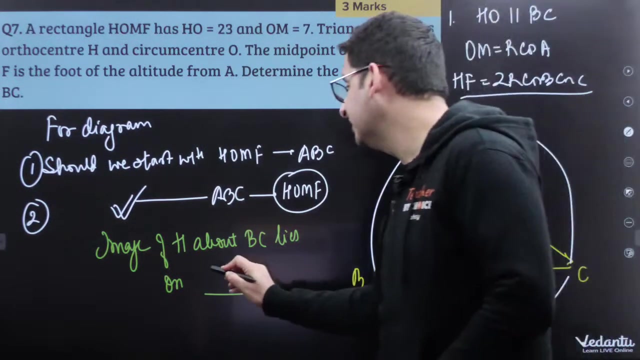 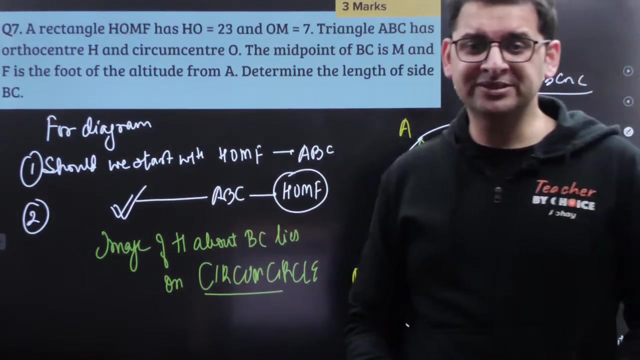 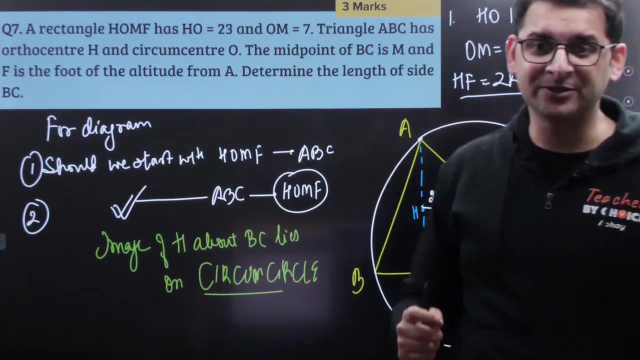 image of h about bc lies on dash. can you feel dash? ortho center ka image? ortho center ka image, guys, ortho center. ka image about bc always lies on, always lies on circum, exactly circum, circle, ortho center. ortho center. ka image about bc always lies on. 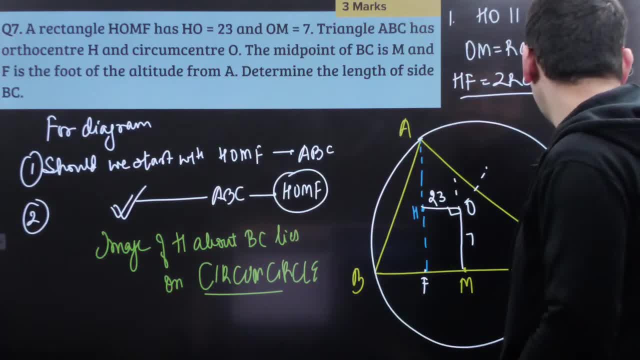 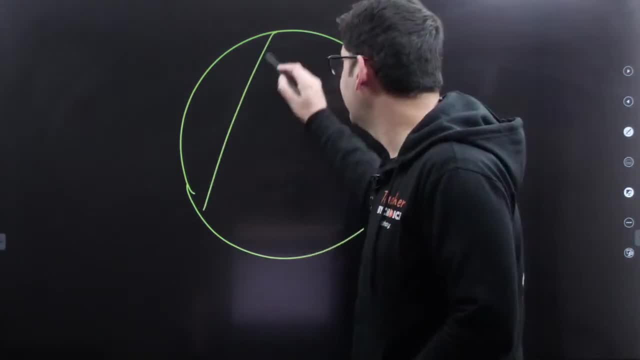 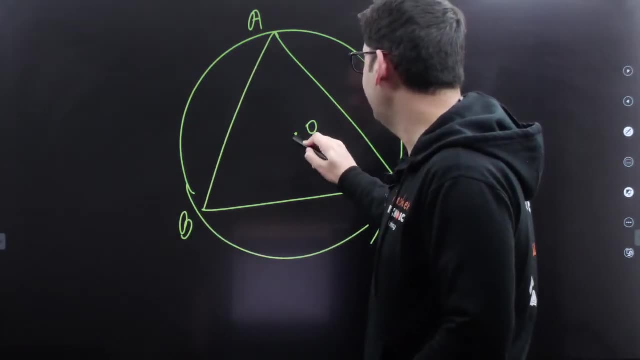 always lies on how om is r cos a dekho, fada fadche mata jata ho agar yeh circle hai, yeh triangle hai a, b, c, circle, circle, circle, yes o hai. let's say: yeh m hai, yeh mid point hai, mid point hai. perpendicular bisector. 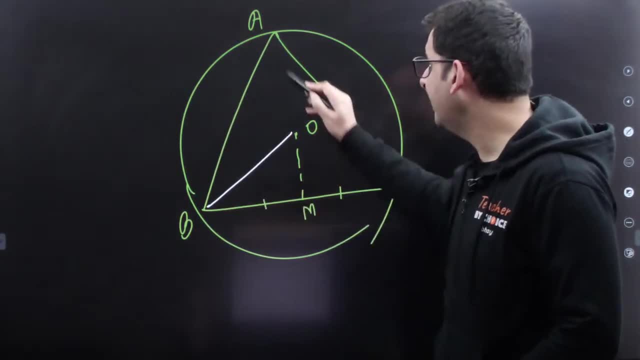 hota hai, kyunki to guys: yeh do cheeze, dhyana rakhakaro ek to yeh. agar angle a hai to yeh wala angle b a hoga, because yeh total angle 2a hoga to half angle a hoga. 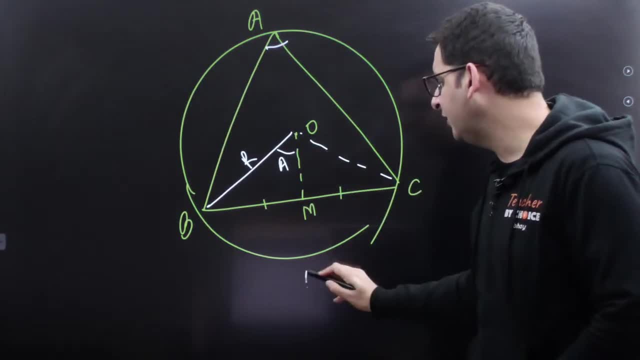 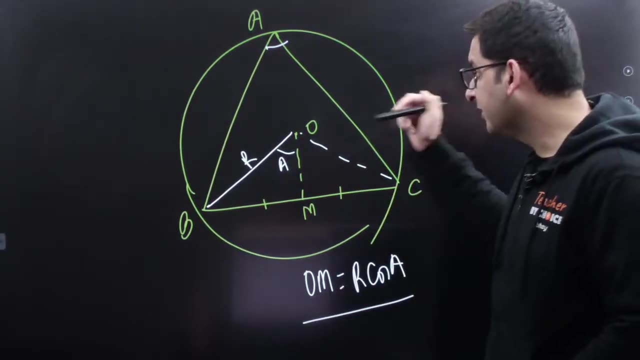 yeh r hai. so is triangle: me om ka value r cos a ho jayega, om ka value r cos a ho jayega. i hope this is clear tikey to yeh angle. a hai to yeh wala angle. a hai aadha angle. 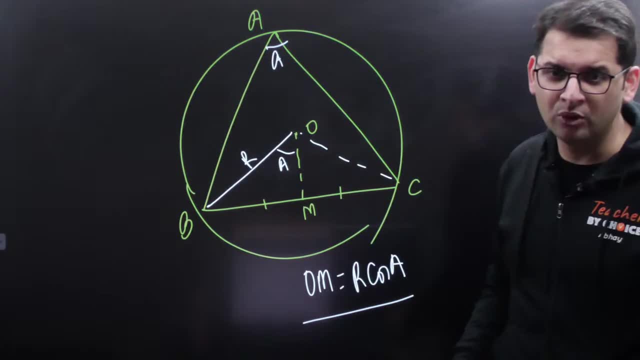 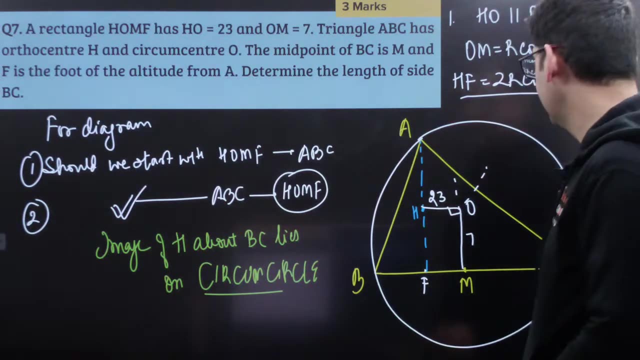 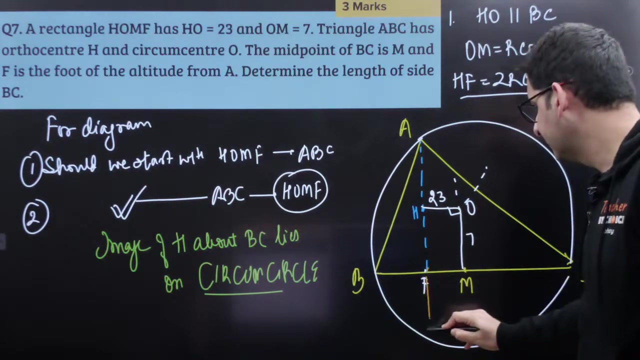 and yeh r cos a hai. to yeh chotey, chotey cheezein, isko dhyana rakhna hoga: tome, tikey, tikey, chalo, chalo. so h ka image about bc lies on, lies on. so let this be h dash isko. 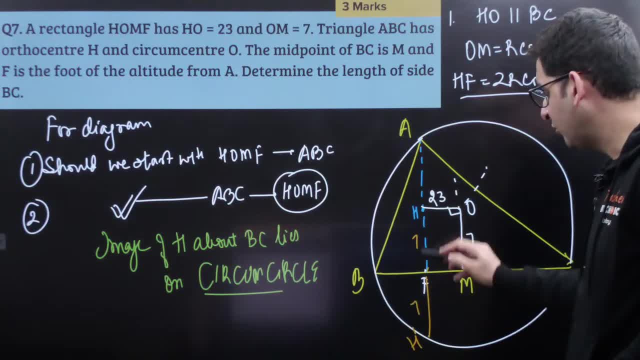 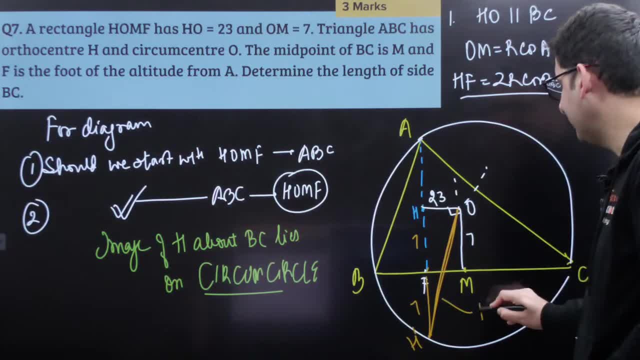 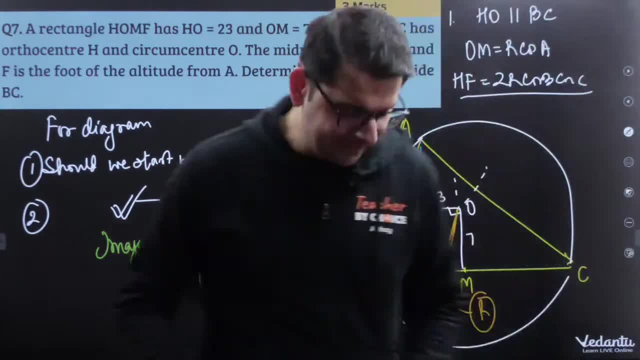 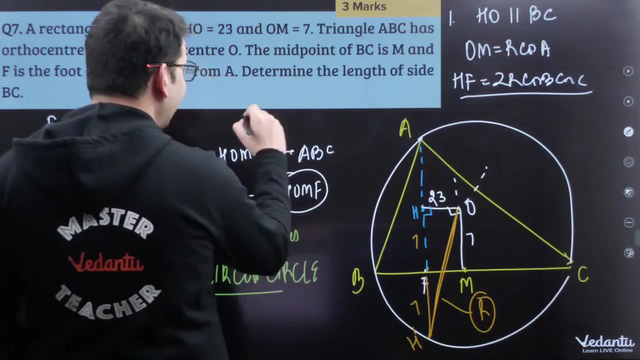 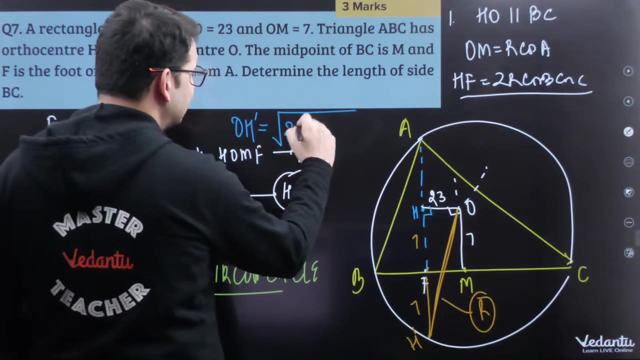 i can find out capital r fada fadche batao. can i find out capital r o h h dash mein? i can apply pythagoras toh o h dash is equal to root of, is equal to root of 23 square plus 14 square maante ho. 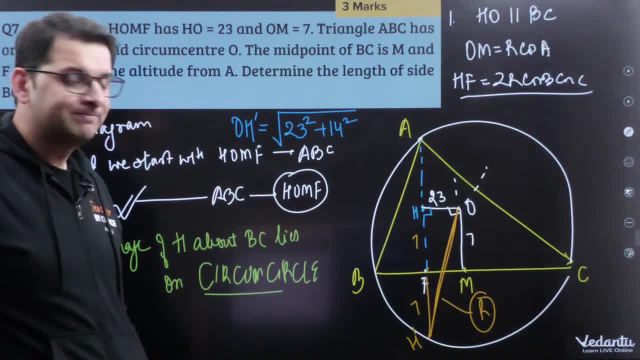 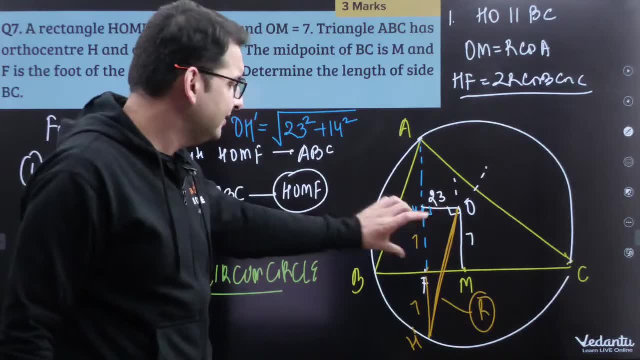 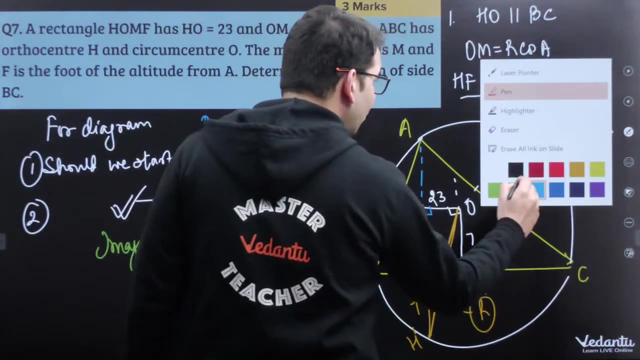 maante: ho, yes or no? Do you all get this? OH' is capital R. capital R is this: 23 square plus 14 square, 7 plus 7 is 14 square. Okay, can I say OH' and OB are exactly same. 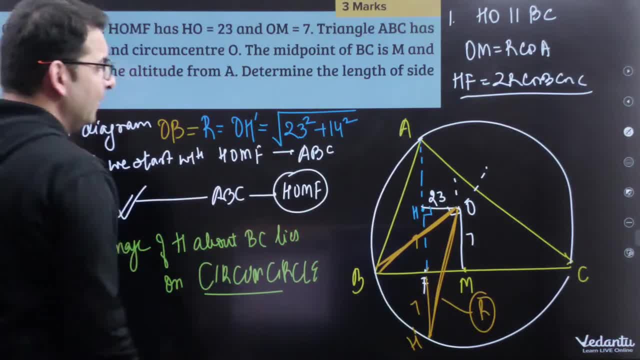 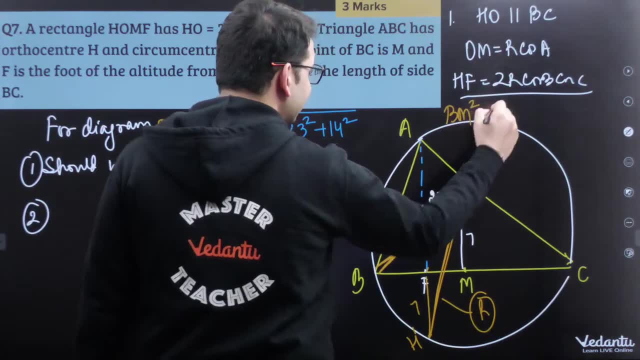 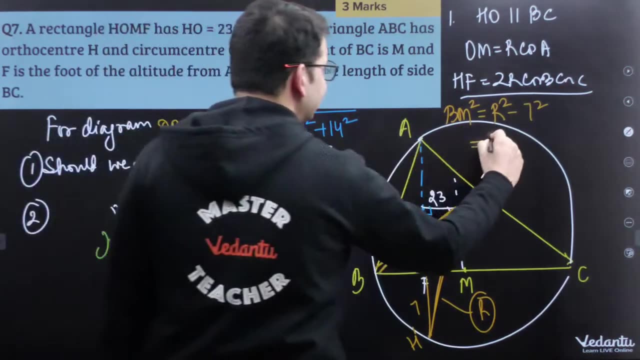 This is OB as well, And if I put a stone in OBM then I will get the value of BM. So BM's square is going to be capital R square minus 7 square. Capital R square is this: 23 square plus 14 square minus 7 square. 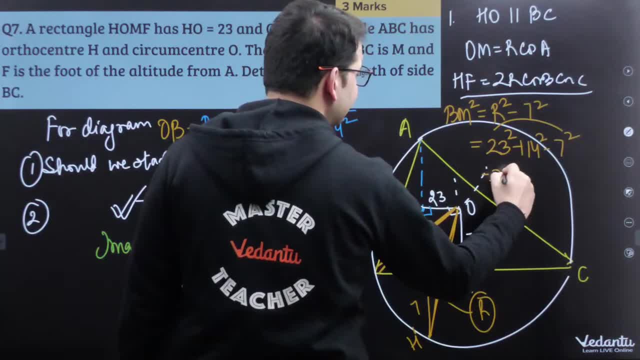 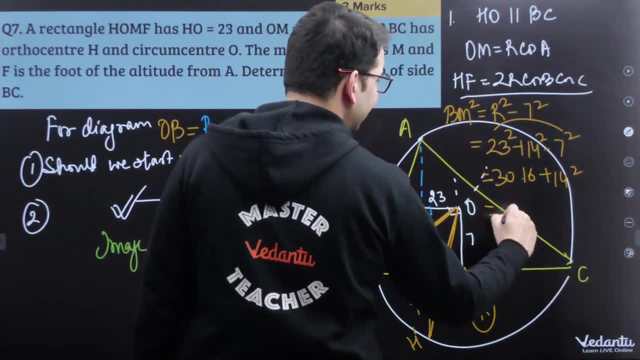 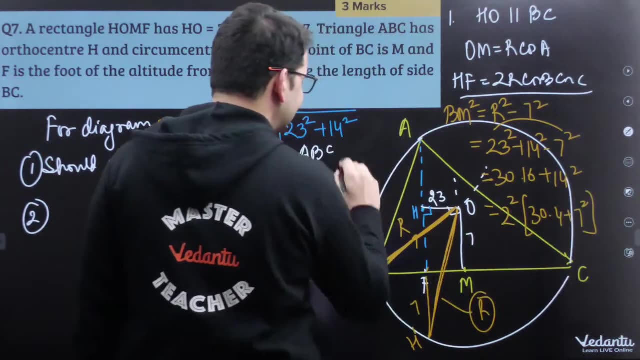 23 plus 7, A square minus B square is 30,. into 23 minus 7 is 16 plus 14 square. If I take out 2 square here, then 30 into 4 plus 7 square 120 plus 49, 169.. 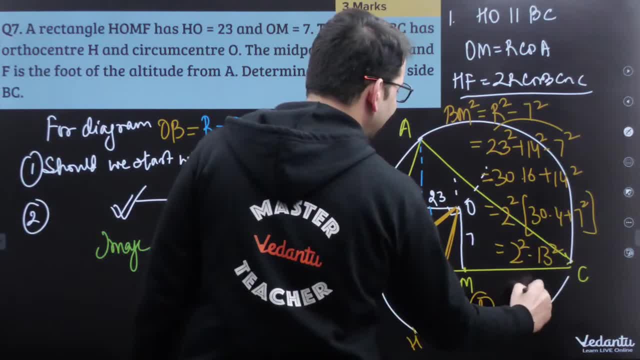 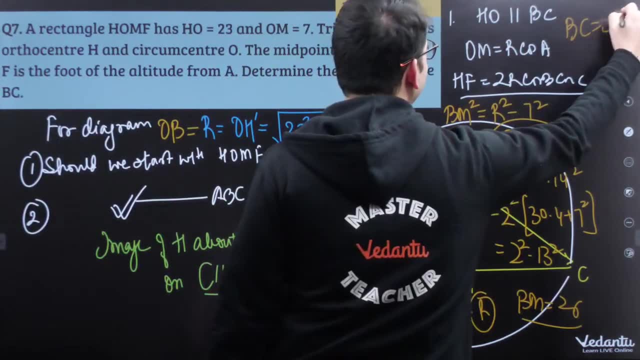 So 2 square into 13 square, So BM's value is 26.. BM's value is 26,, so BC's value is 52.. BC is 52.. So 52 is the right answer. I hope this is clear. 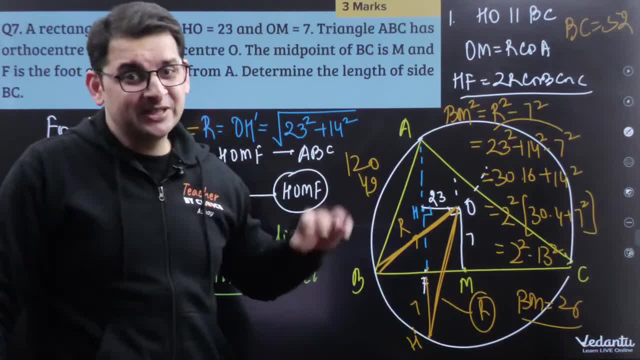 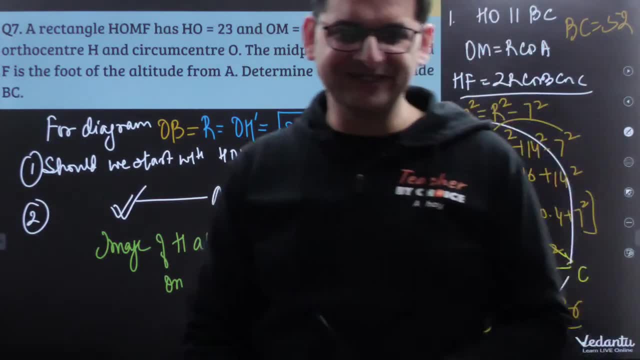 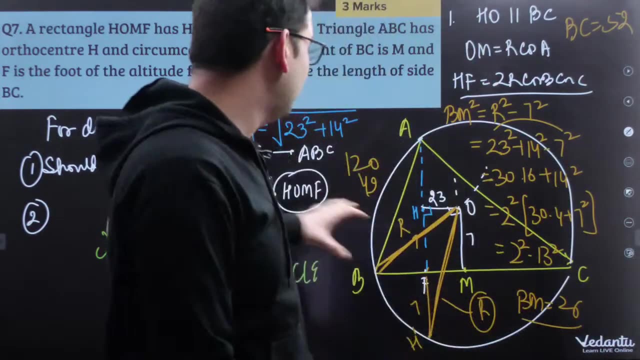 I hope this is clear. Got it everyone. This was an amazing question. It was a very good question. It was a very good question. Amazing, amazing, amazing, Akshit, super, Super. Did you all get this? Apart from this, there are a lot of other solutions also. 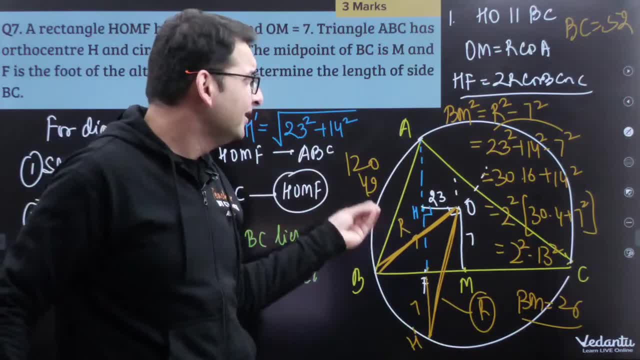 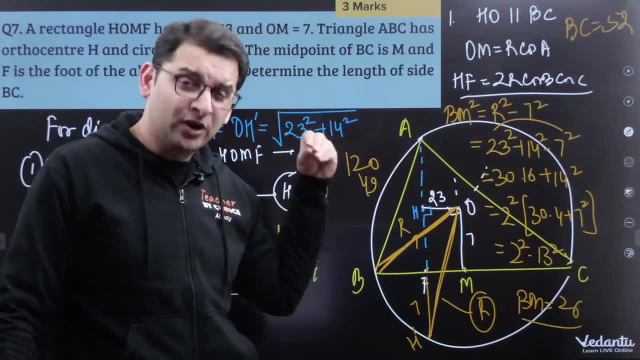 Apart from this, there are a lot of other solutions. If you do this carefully and go inside, you will be able to find a lot of other solutions also. Your task is, apart from this solution, if there is any other solution, if it is good. 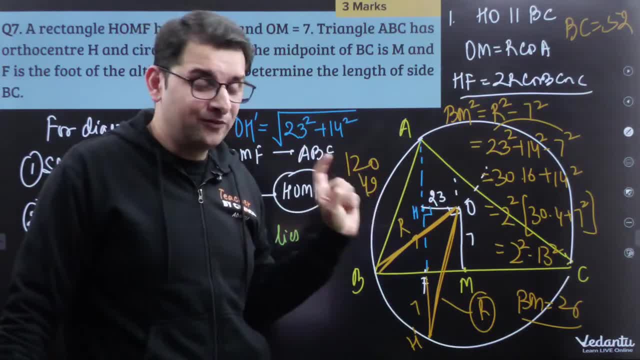 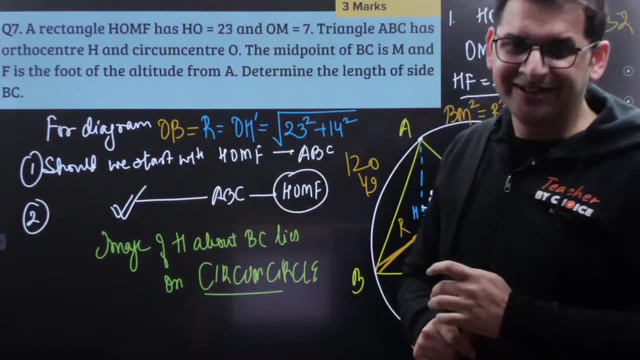 if you find it, just ping me over telegram, and I would want to see that. But this was a very lovely, very elegant kind of solution. Yes, Got it, Got it, Got it. So this was a three-marker, guys. 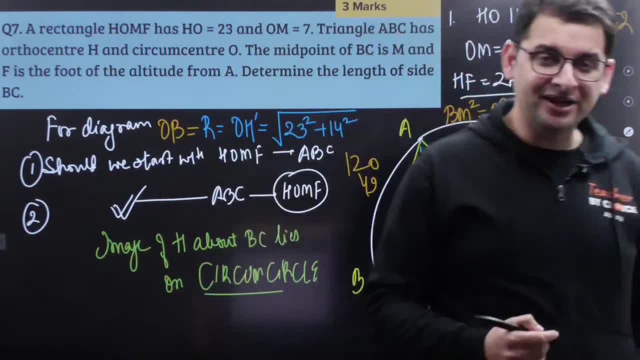 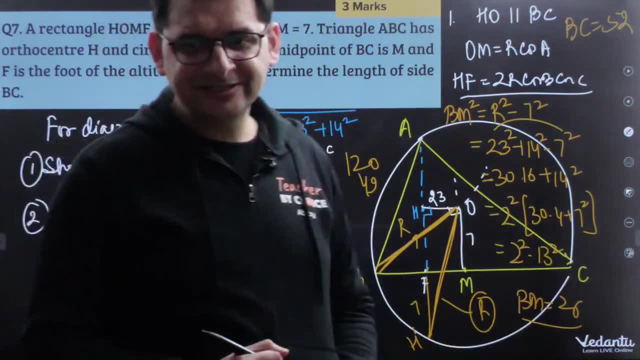 This was a three-marker. The five-number question is not that easy. You have to put a lot of thought into it, But this was a three-marker. Got it, Got it, Got it. Yes, Yes, Yes, Abhishek. 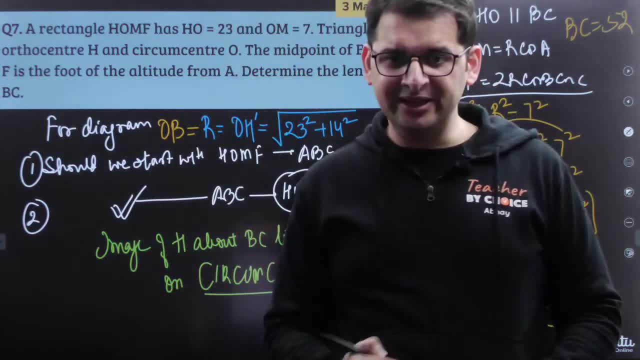 Abhishek, There are a lot of other solutions too. There are a lot of other solutions, But this was a very amazing, very simple solution. There is no need to do anything here. Got it Super, Super, Yes, Yes. 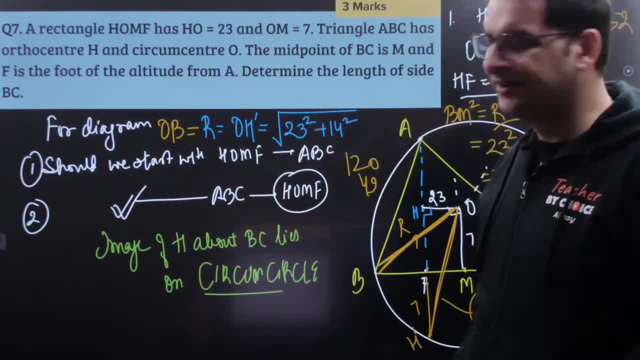 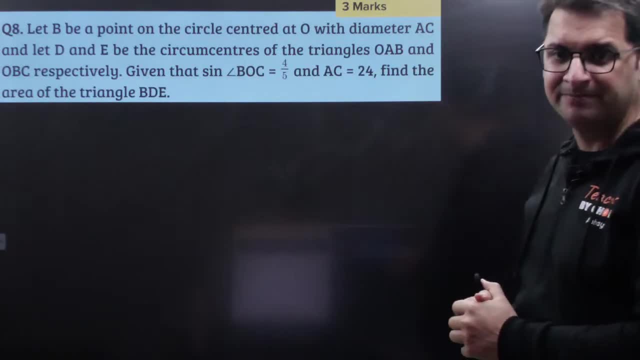 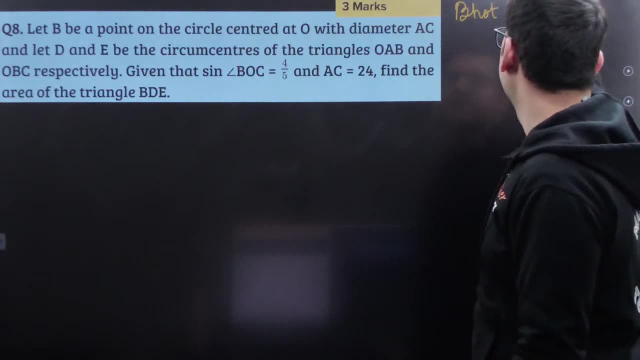 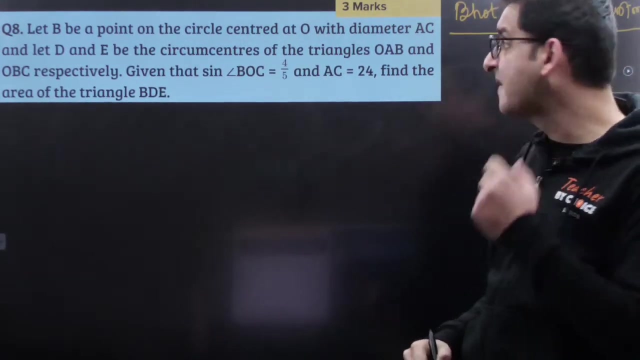 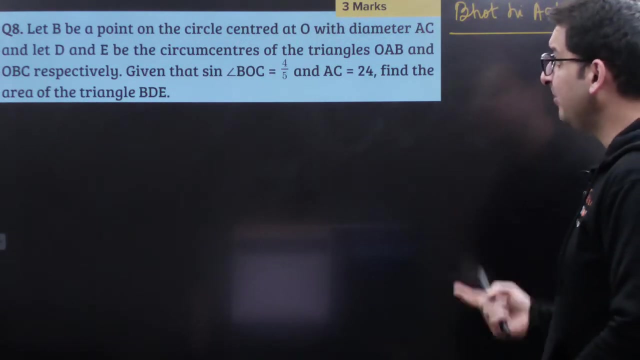 Yes, Yes, Yes, Yes, Super Super. Moving on to the next question, which is this: This is again a very, very amazing question, guys. Very good question, Very good question, Very good question. So let B be a point on the circle centered at O with diameter AC, and let D and E be the. 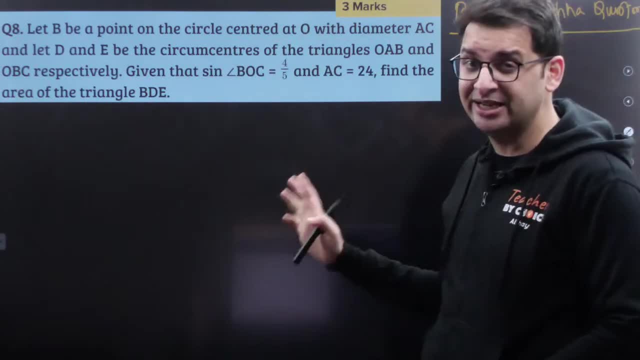 circumcenters of triangle, OAB and OB. Yes, Yes, Yes. So for this you will have to make the diagram, guys. There is no other option. So it was a very easy one. Yes, Yes, Yes. 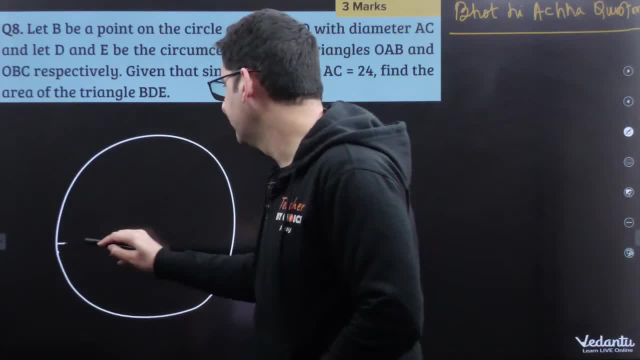 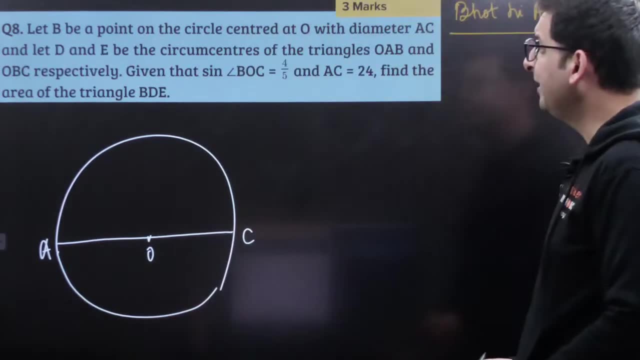 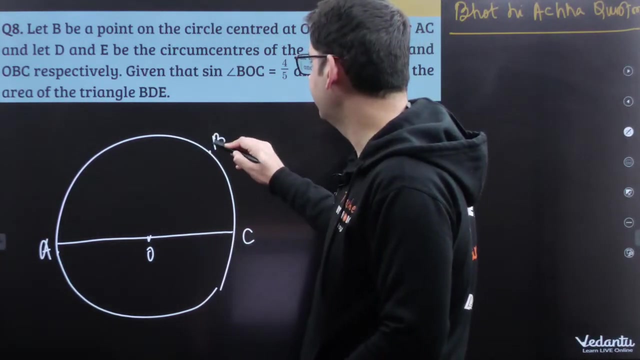 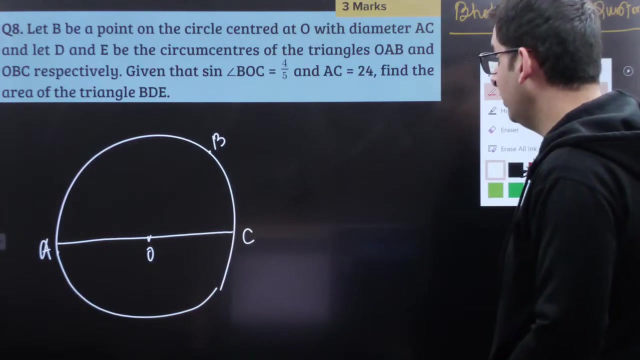 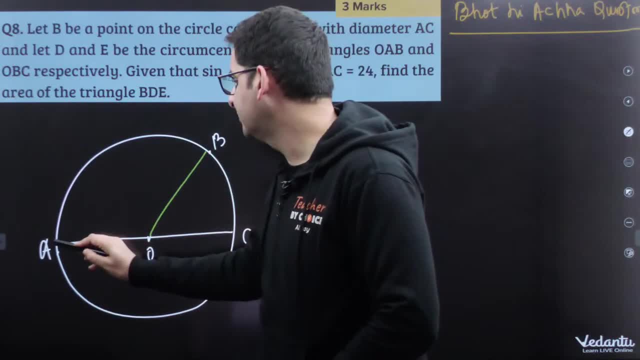 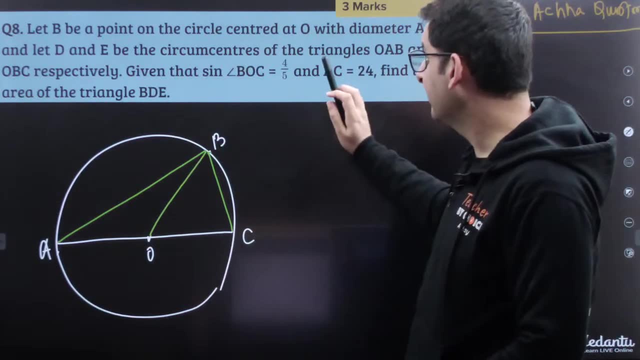 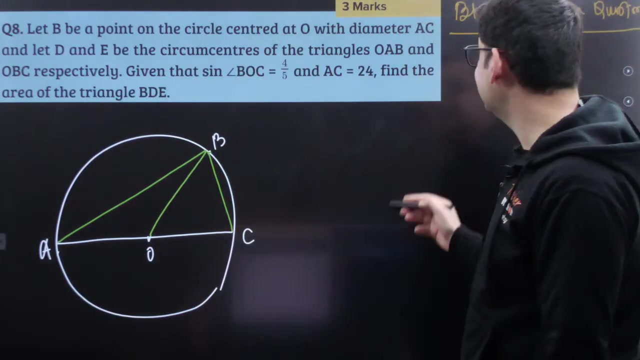 So let's join this and this And let's join this as well. Now, what is he saying? D is the circumcenter of OAB. Do you understand circumcenter? Do you understand circumcenter? So D is the circumcenter of triangle OAB. 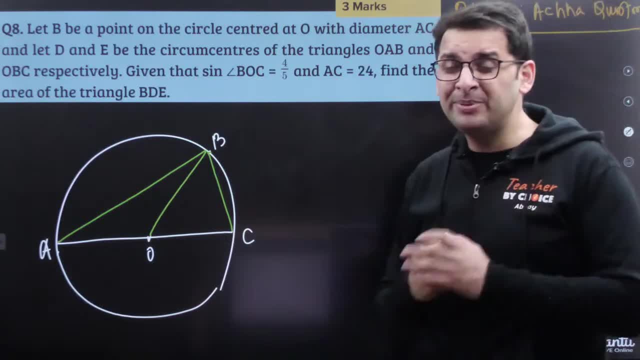 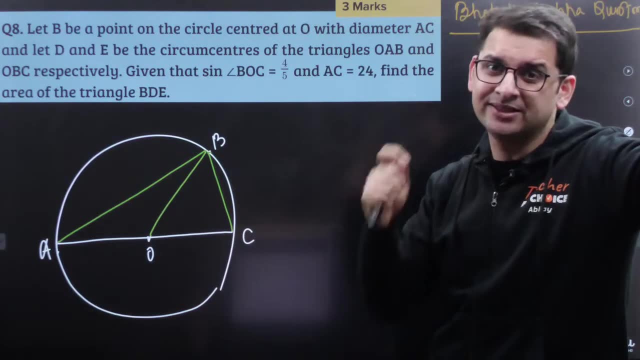 And E is the circumcenter of triangle OBC. So here, when it comes to questions like that, you gave the circumcenter of two triangles, you gave the incenter of two triangles. So here we always follow the basics That what is circumcenter from there? 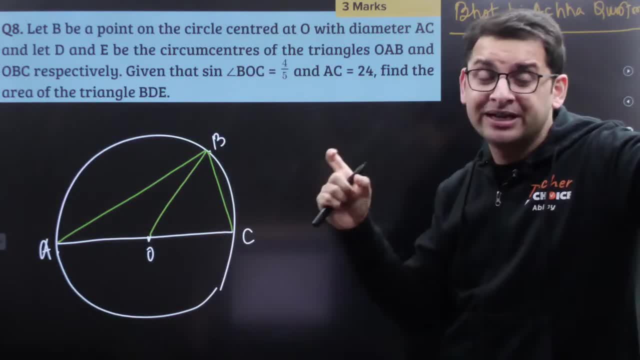 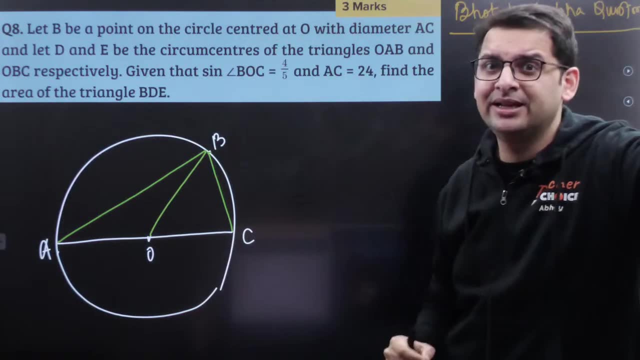 So circumcenter is the point of concurrency. of whose point of concurrency is it made of? We should be very clear in our minds, Should be very clear That how is circumcenter made, How is incenter made, How is orthocenter made? 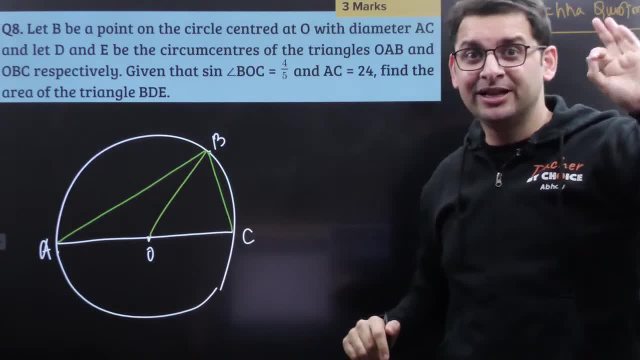 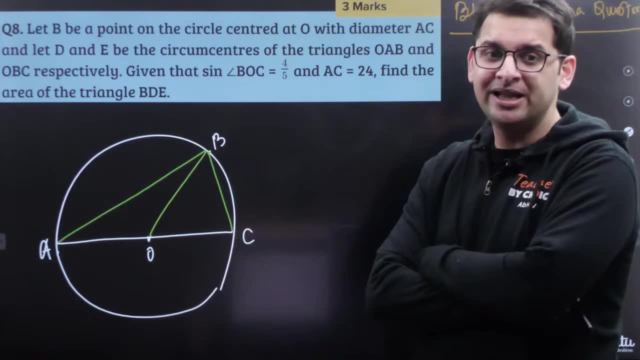 Formulas come later. First the basics: How is it made? How is it made? How is it made? Where does it come from? So someone told me: how is circumcenter made? How will circumcenter be made? Quickly tell me the question. 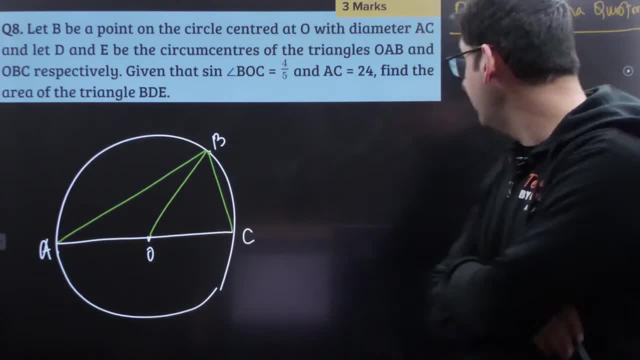 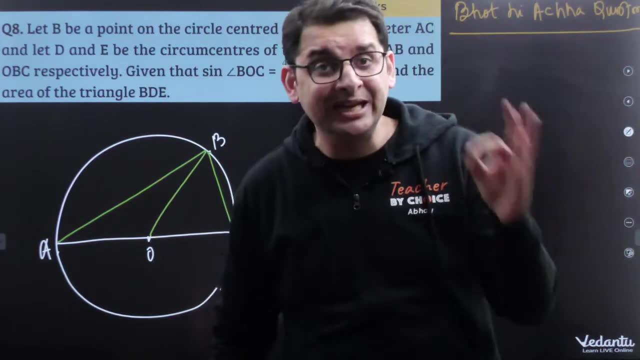 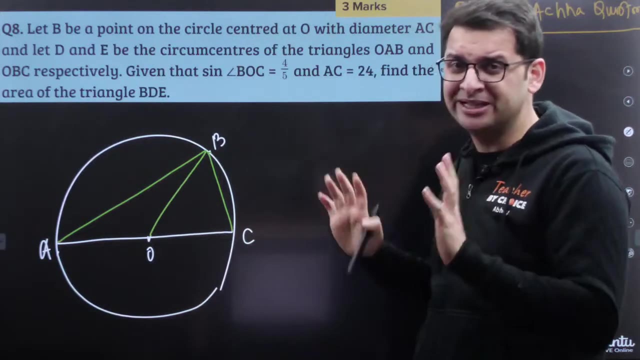 How does circumcenter get formed? Circumcenter is the point of concurrency of Circumcenter is the point of concurrency of, Quickly, on the exactly perpendicular bisectors. So here, perpendicular bisectors, exactly what will be made? I don't know. 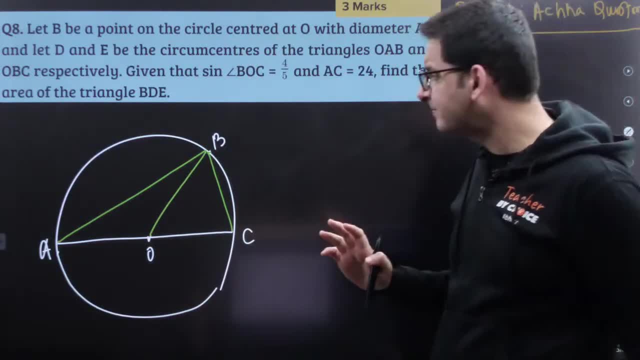 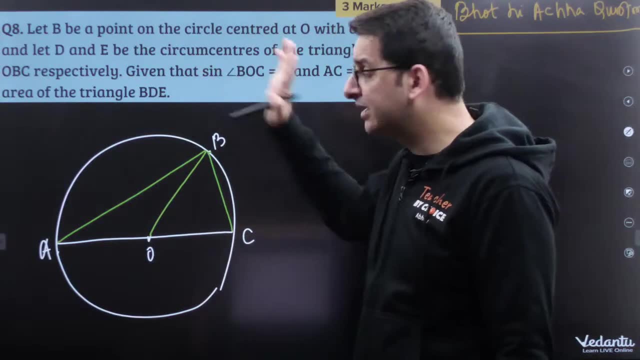 But we try to make thick perpendicular bisectors. Now there is one more thing here: The circumcenter of OAB is D and the circumcenter of OBC is E, So O is perpendicular to OB and O is perpendicular to OA. 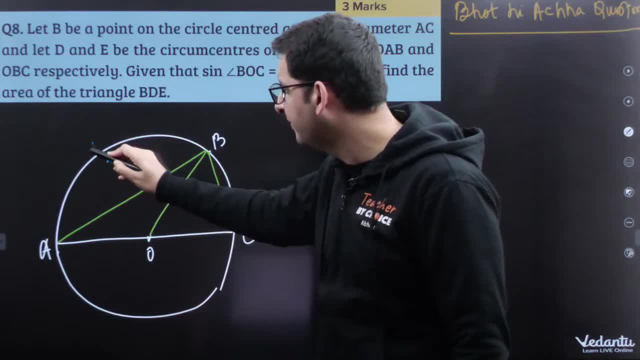 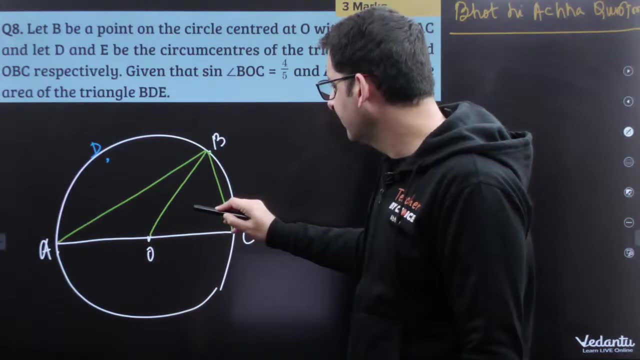 So perpendicular from here and perpendicular from here, So D will be somewhere here. Let's assume D will be somewhere from here, And the perpendicular of OB will be somewhere here, So E will be somewhere here. From here to here, E will be somewhere here. 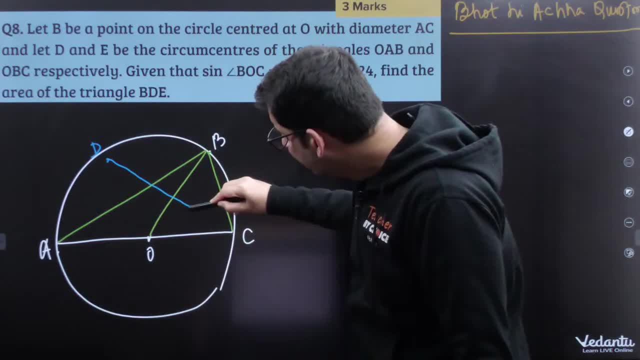 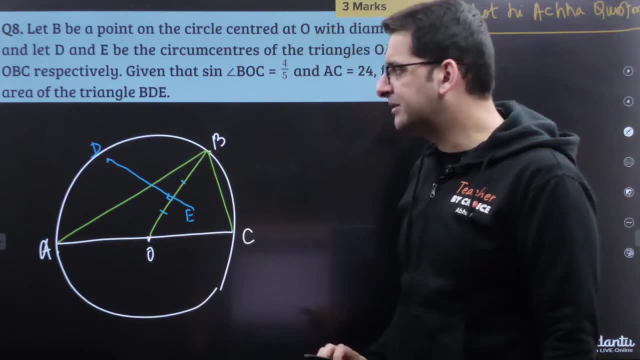 And I know that when I join these two here, this line is actually perpendicular to this line, Perpendicular bisector. Let's say: this is E, This line is perpendicular bisector. So D is the circumcenter, E is the circumcenter of this. 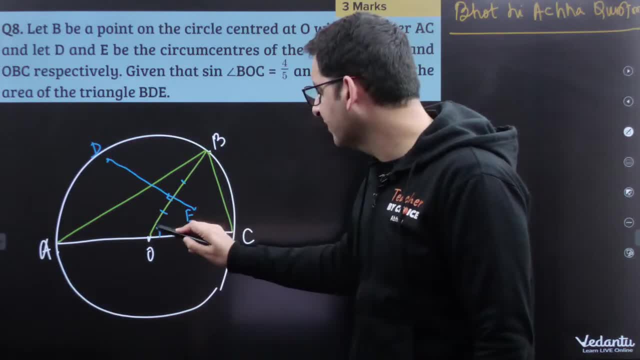 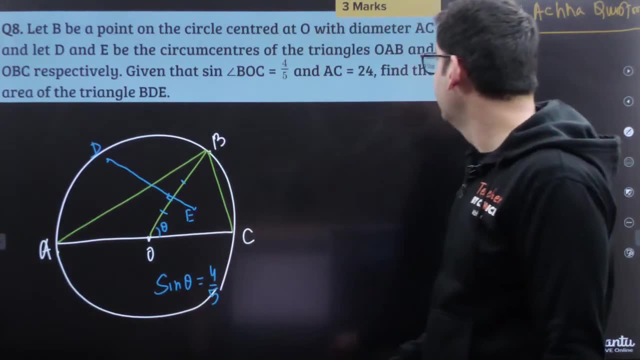 Okay, what we have to find out? BOC: this theta is given. So I know that sin theta, Sin theta is 4 by 5.. This is also given And AC is 24.. So this is 12 and this is also 12.. 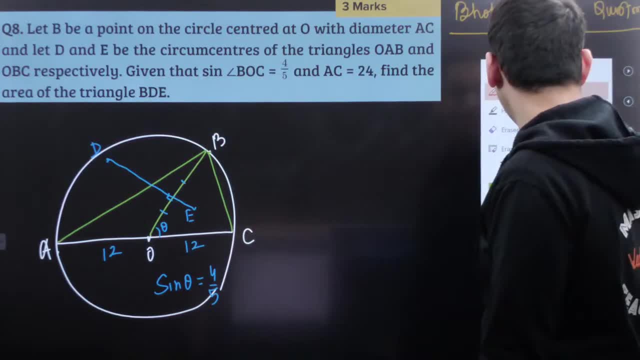 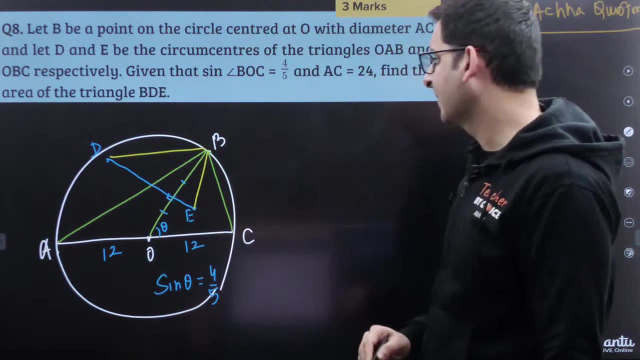 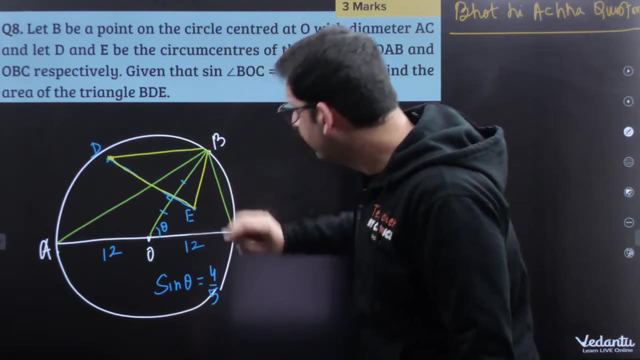 AC value 24 is given. What is the area of triangle BDE, BDE. Let's join BDE first. So this is BDE, This is BDE. We have to find out its area. We have to find out its area. 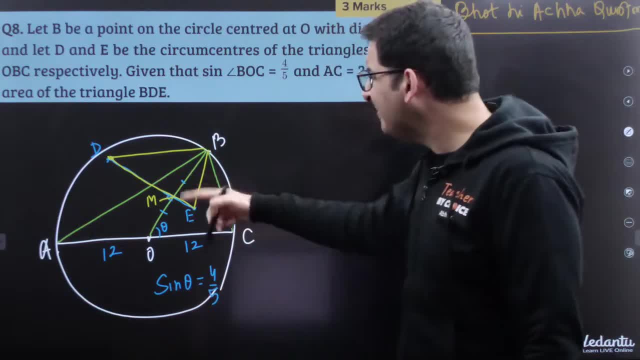 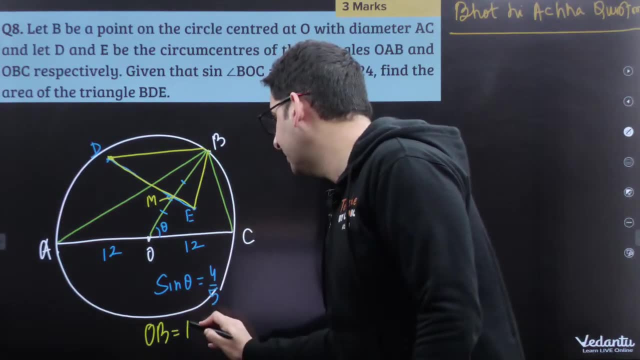 Let's say this point is M. Let's call this point M. M is the midpoint of OB, M is the midpoint of OB And OC is same. So the value of OB is 12.. So OM and MB will be 6.. 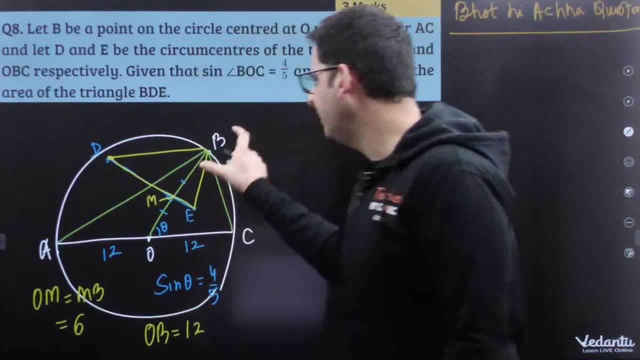 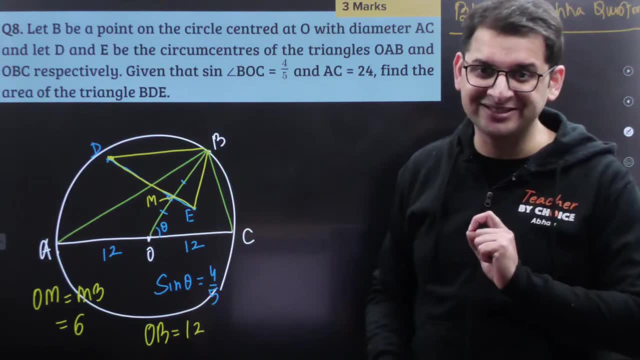 OM and MB will be 6.. OM and MB are 6.. OC is 12. So OM and MB are 6.. So OM and MB are 6.. I hope this is clear. I hope this is clear. Sin theta is 4 by 5, so cos theta is 3 by 5.. 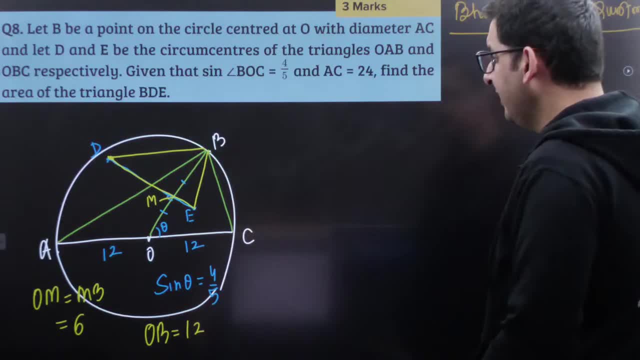 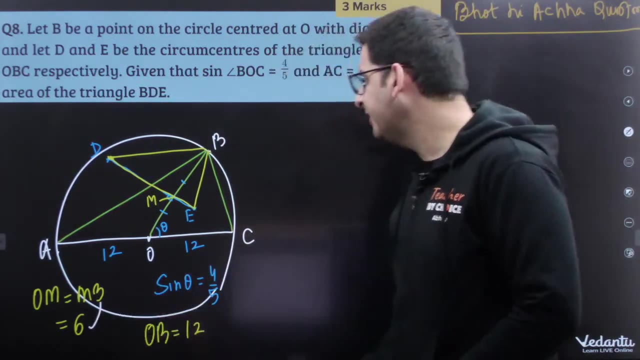 I want to find the area of MDE. I want to find the area of MDE- Sorry, BDE, For the area of BDE guys, For the area of BDE guys. Imagine, for the area of BDE. value has come, height has come, bm is height, bm is height, so half into bm, if I somehow 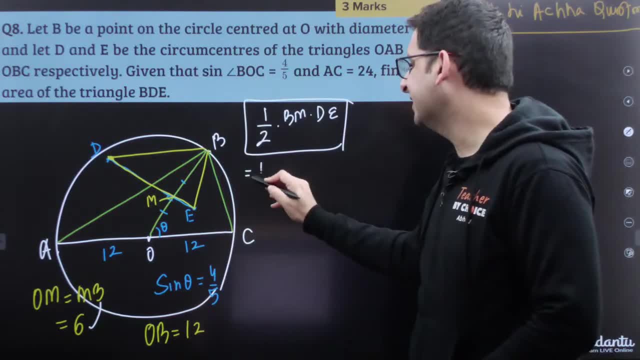 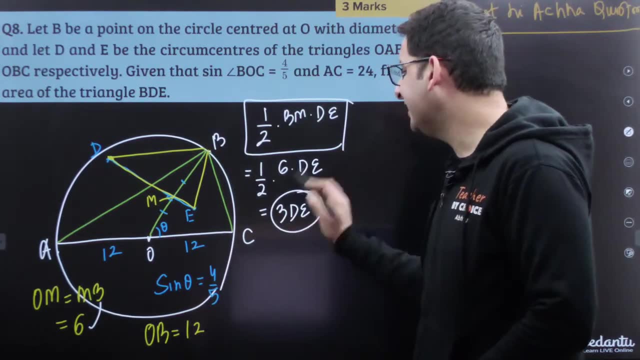 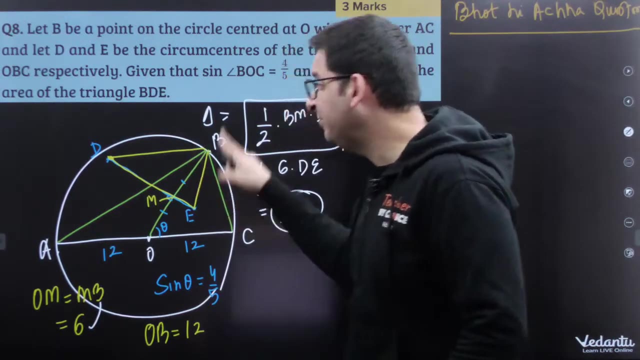 take out de. can I say I am done so this is half into 6 into de, so basically 3 times de. so whatever the value of de is, that is the area of triangle bde. so think like this: what to do, what to take out, to take out the area of bde now, how to take out the area. 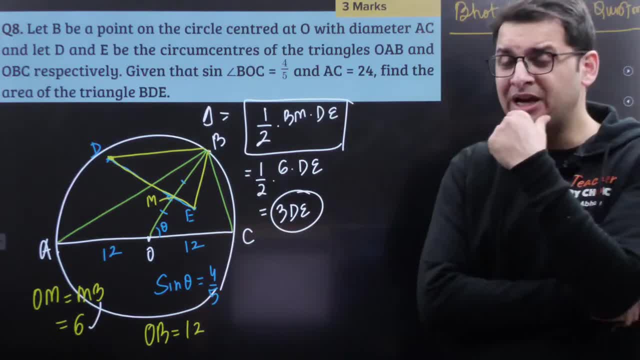 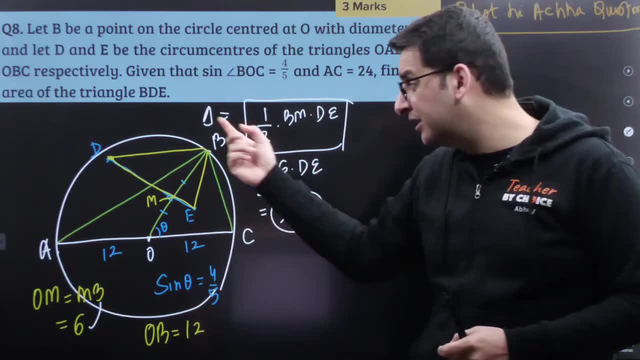 of bde. one is half base height. this is half base height, second half into product of two sides, into the sign of an opposite angle, internal angle. there are many other ways. if I know the value of all three sides, then I can apply the hero formula. so here is the. 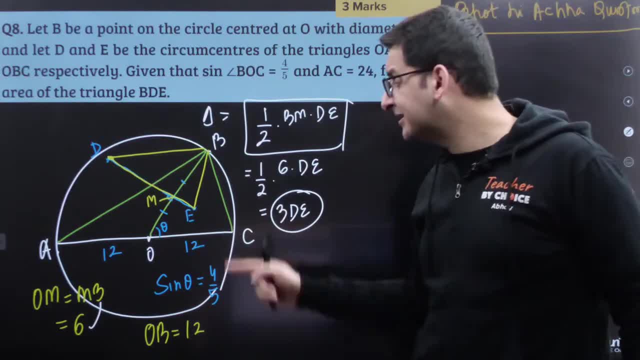 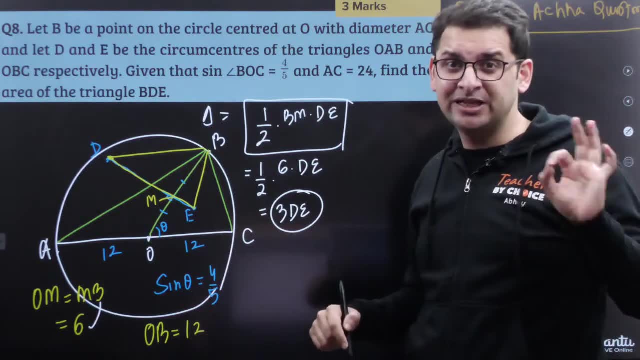 best approach. half base height will shine. can all three sides be taken out? If all three sides are taken out, then maybe it will be very difficult. if all three sides is going to be really difficult for me, because abhi ek bhi side nahi pata. 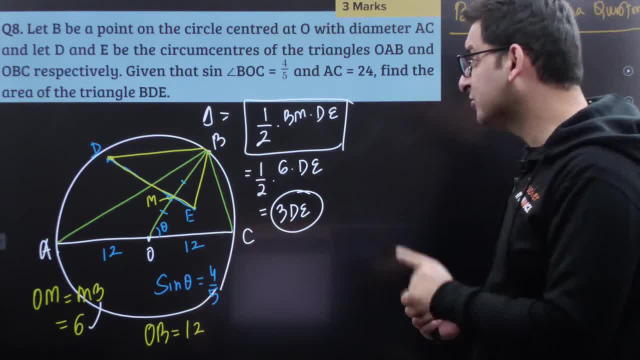 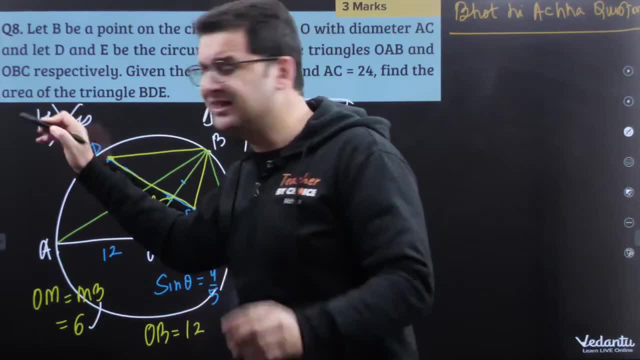 ek bhi side nahi pata. so tino side nikalna is going to be really difficult for me, so I am not going there. Hero's formula: maine kharij kar diya. Hero's formula kharij kar diya Nahi. 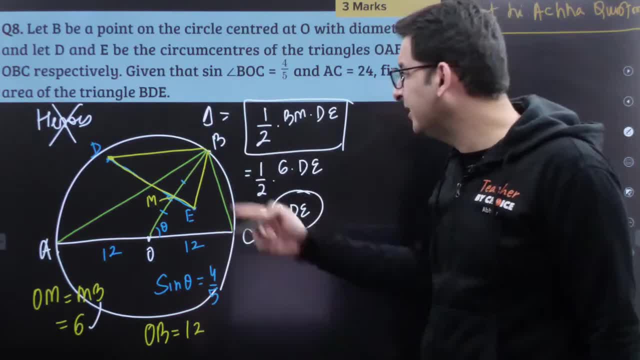 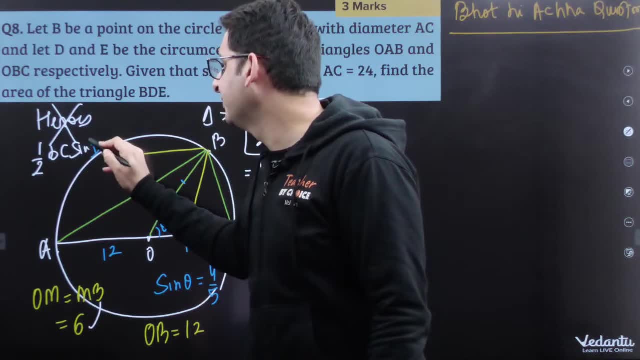 Half BC sine A. Kya mujhe iska sine pata hai, Pata nahi. Do sides bhi nahi pata Chhor diya. Half BC sine A Chhor diya, But half base height mujhe dikhaya, zira. 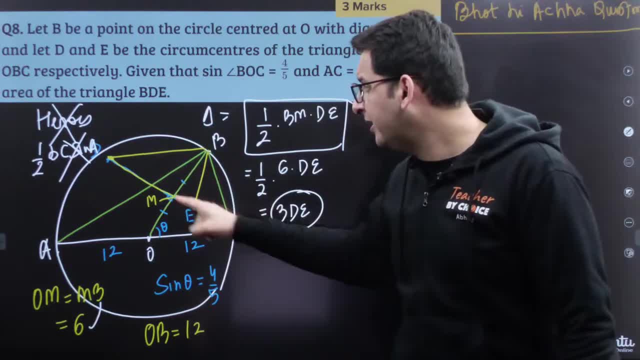 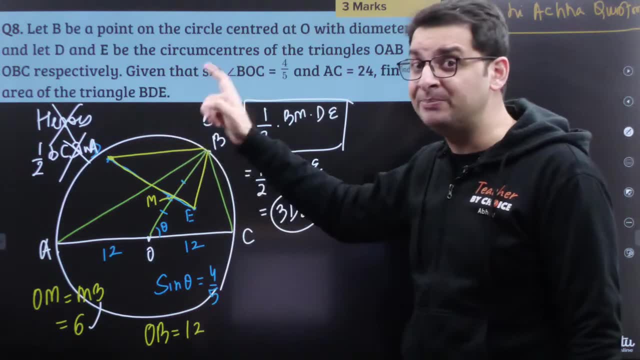 because maine jaise dekha, basic se gaye Ye jo hai. DM is nothing but perpendicular bisector of OB, because D kya hai? D is circumcenter. Kaise banta hai Perpendicular bisector ke point of concurrency? 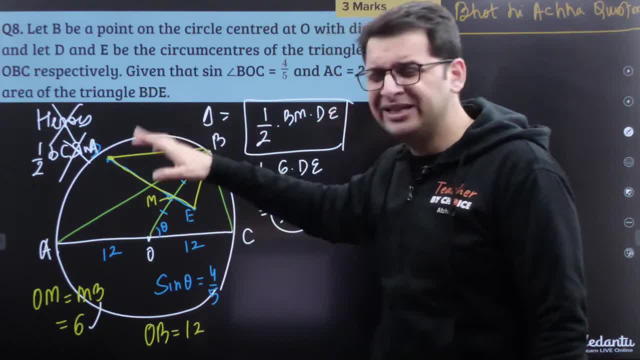 Iska banane ka zaroorat nahi hai. Iska banane ka zaroorat nahi hai, because chahiye nahi Ho sakta. chahiye hoga to baad mein dekhenge. but DM is the perpendicular bisector, Matlab M midpoint. 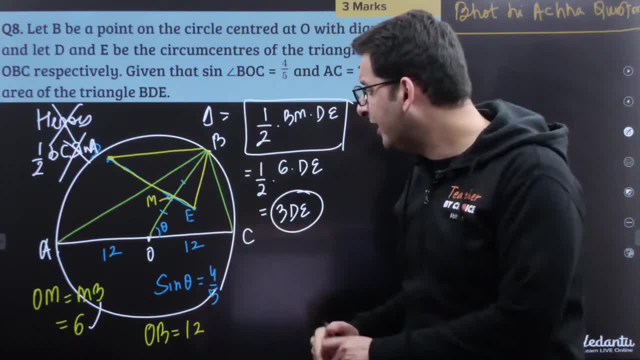 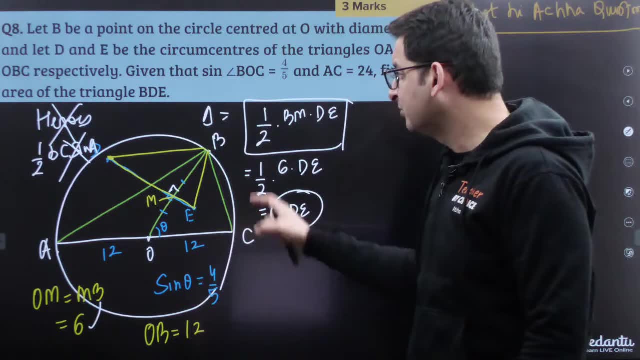 M agar midpoint hai aur perpendicular hai to ye height ho gai BM. BM ka value 6 hai, because total OB ka value 12 hai, To ye 6 hoga. Ye 6 hoga because M is ka midpoint hai. So mujhe OM aur BM. 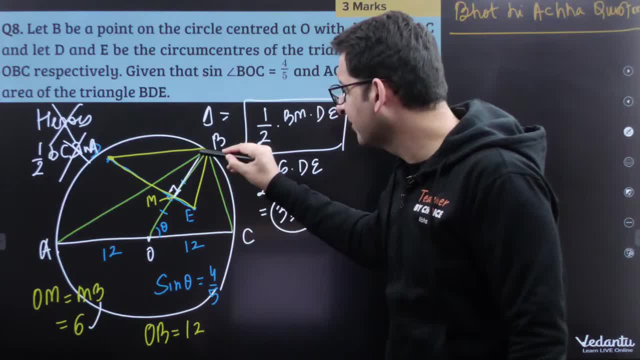 a gaya 6, 6.. So ye, agar 6 hai, This height is 6.. So yaar to mujhe sirf ye nikalna DE. So agar DE nikal gaya, I am done. So how do we? 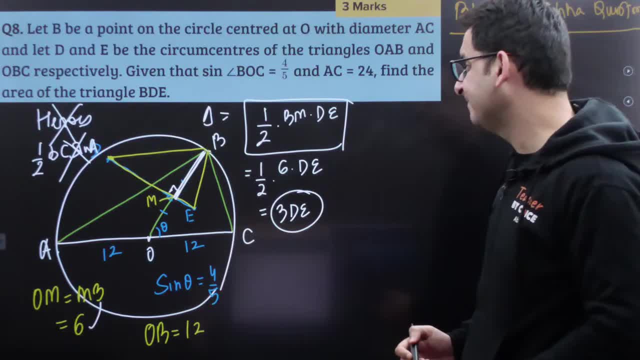 find DE. That is the question, guys. How do we find DE DE? kaise find kare? Ab mujhe sochke? batao Ab kaun bacha dekhte hai. yahape Kaun bacha mujhe batayega. 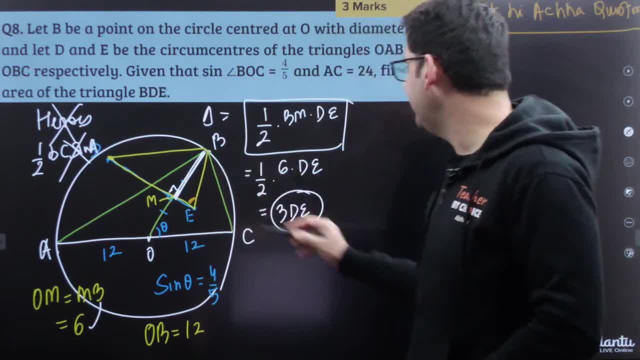 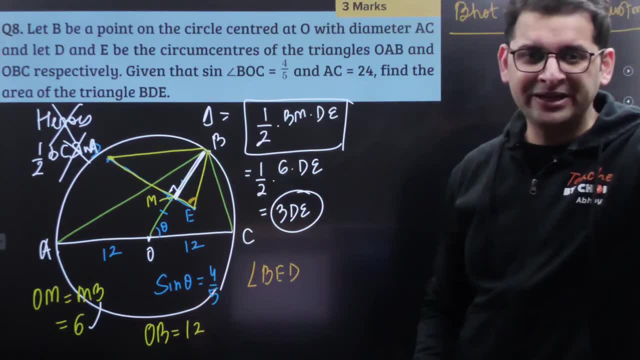 What is going to be this angle guys, Angle BED. Koi mujhe bata sakta hai? what is going to be angle BED on the chat box? What is going to be angle Abhi hamne thodi dara pehle discuss kya tha. 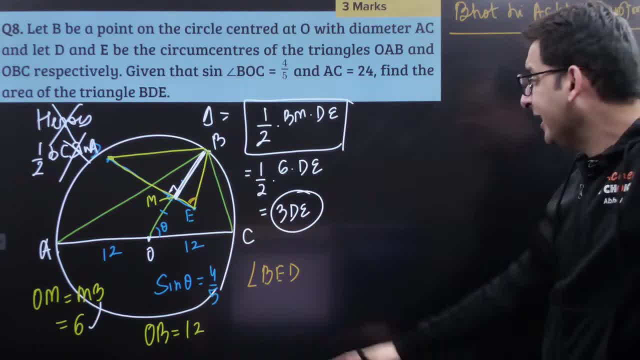 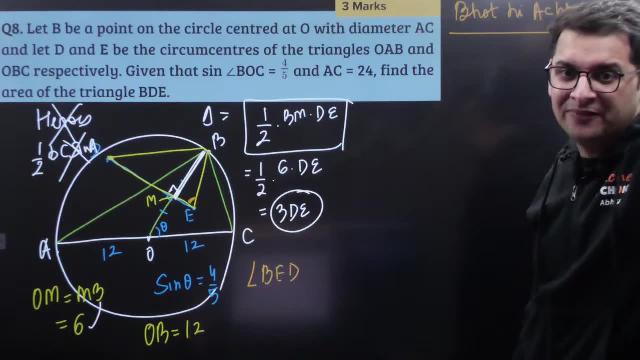 isko Abhi hamne thodi dara pehle discuss kya tha. Agar ME iska angle perpendicular bisector hai, What is going to be angle BDE? Aarav is saying BED is going to be angle C. 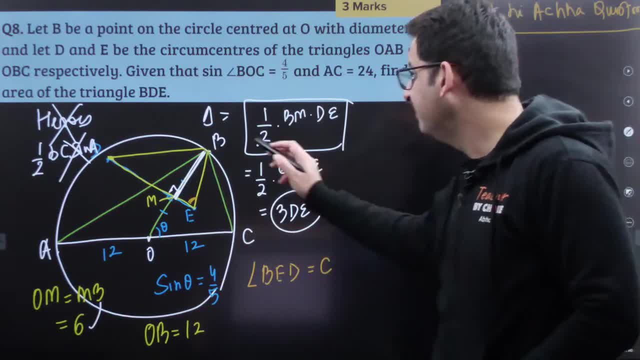 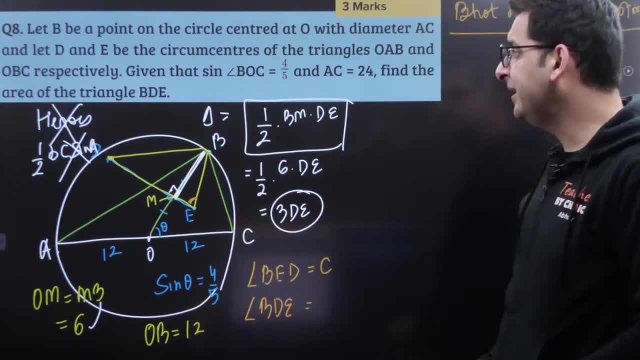 BED is going to be angle C And what is going to be BDE? Angle BDE kya hoga. Koi bata sakta mujhe Angle BDE kya hoga? Anyone BDE? What is going to be BDE? 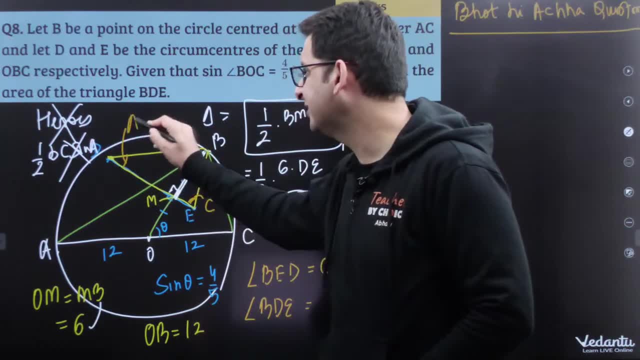 Ye buche tum bol rahe hain, C hoga This, Can I say, this is similar tarike se A hoga. This is going to be A. Ye kaisa hai, Ye aise hai, Abhi hamne. 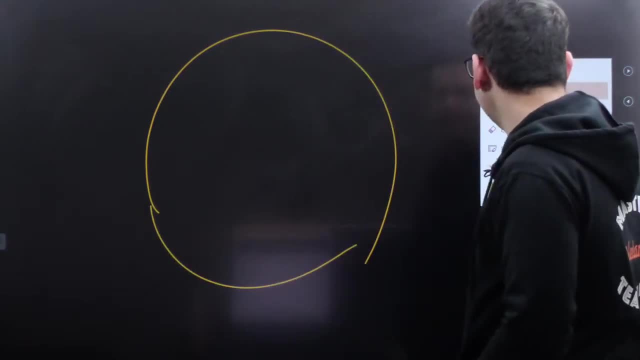 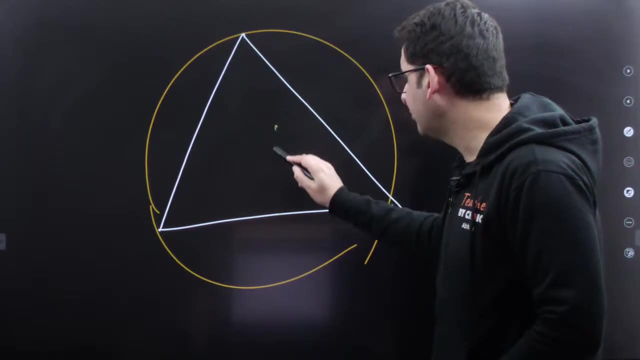 discuss kiya ki agar ye circle hai, Agar ye circle hai, Ye triangle hai, Yaha par iska perpendicular bisector draw karte hain, Yaha se perpendicular bisector draw karte hain O point pe meet kar raha hai. Agar ye A. 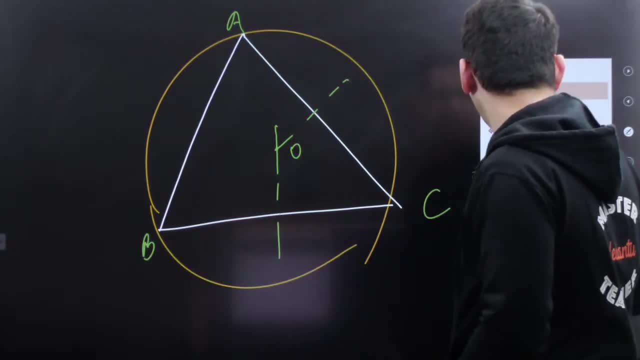 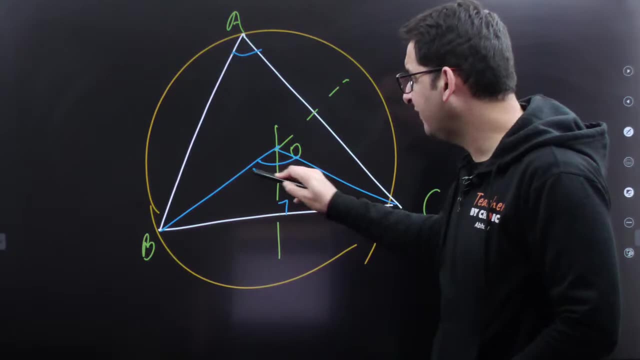 hai, Ye B hai, Ye C hai To agar main inko join karta hun OB ko aur OC Ye. agar angle A hai to central angle 2A hoga, Since ye perpendicular bisector to ye wala angle A hoga To ye wala angle. 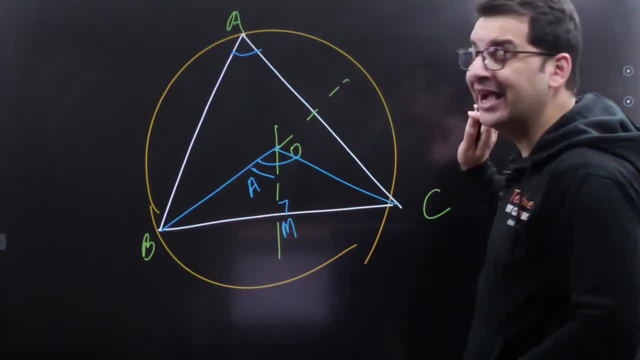 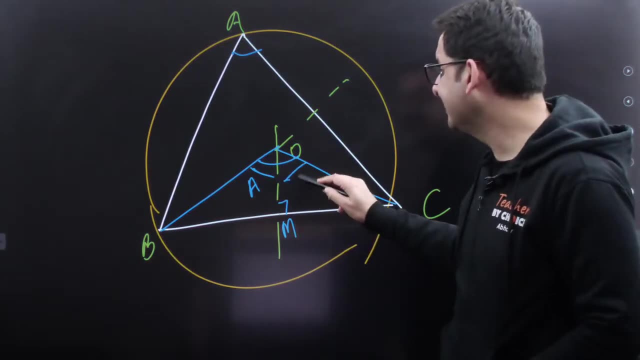 BOM is BAC. As simple as that. Isko zahinak na BOM is BAC. Isko hamesha dhyan rakhna. This angle is A. This angle is also A. This angle A. 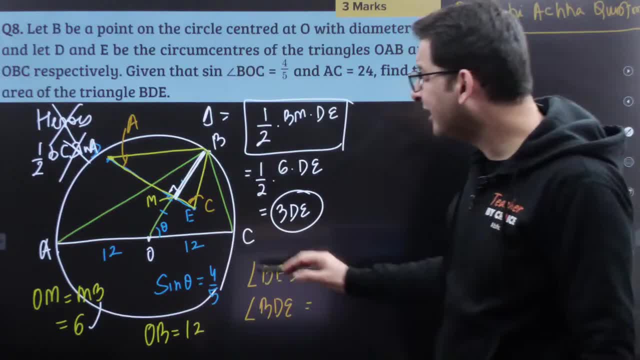 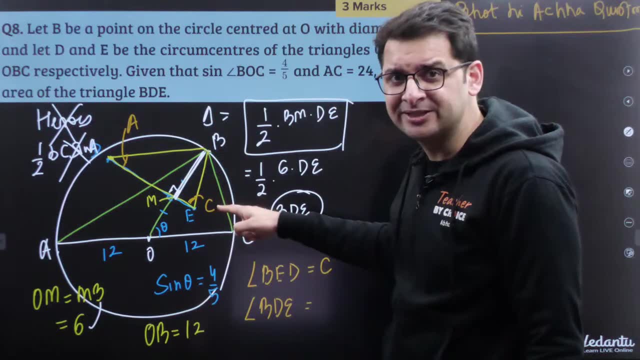 Got it? Got it, Got it. Yes, Super To yaha par exactly same cheez To agar ye perpendicular bisector to OBC, pe nazar dharma lo OBC Triangle, OBC Perpendicular bisector, To kena say: 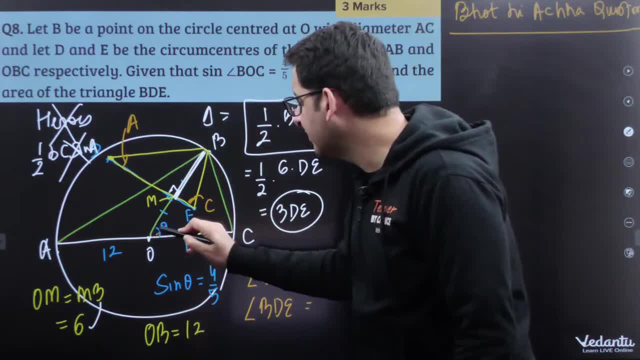 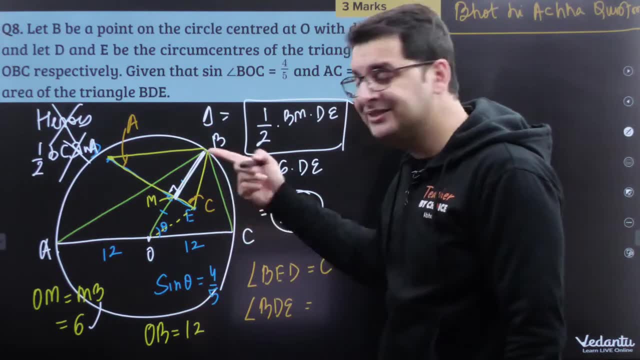 agar mai, agar mai yaha se bhi isko join kar dita ho, Isko join kar dita ho. Ye total angle Ye C hai to ye angle 2C hoga To aadha angle C hoga To ye C hai To ye bhi C hai. 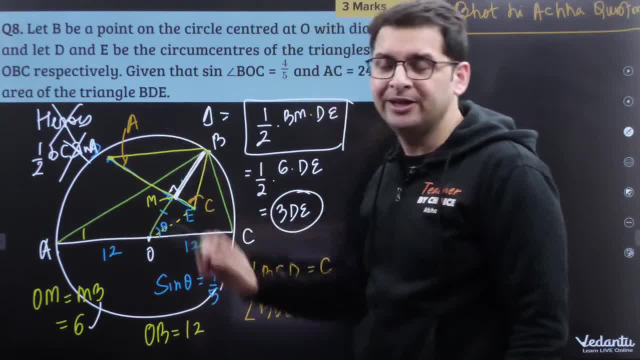 Similarly, ye agar A hai, Ye bhi A hoga, Ye bhi A hoga, Ye bahar nikal gaya, But again concept to same hi raega. So can I say, guys, Since this is A, This is A. 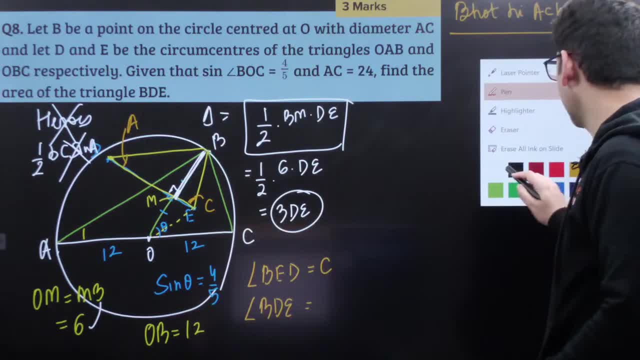 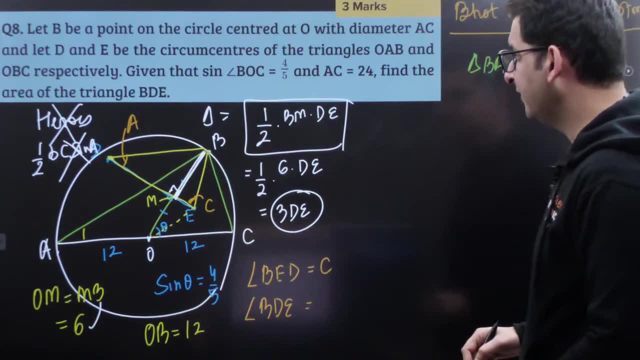 This is C. This is C To kya mai yaha par bol sakta ho, Kya mai yaha par bol sakta ho ki triangle BAC is similar to sorry. Triangle BAC is similar to triangle BDE BAC. 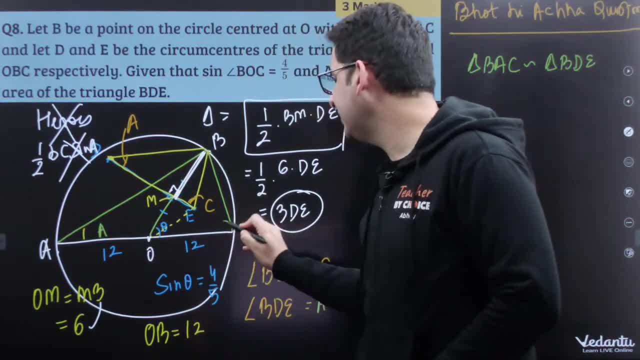 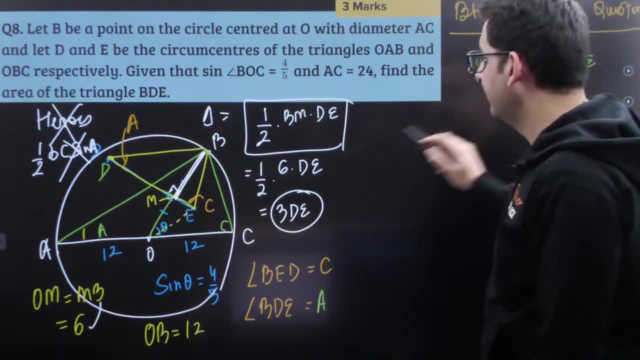 BAC BAC, Because ye A hai to ye A hai, Ye C hai to ye C hai To yaar BAC mein or BD, BDC mein, Sorry, BDE, BDE mein, BDE mein aur BAC mein, do angle same ho gaya. 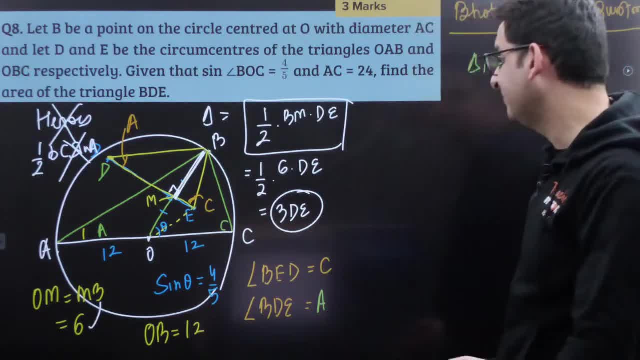 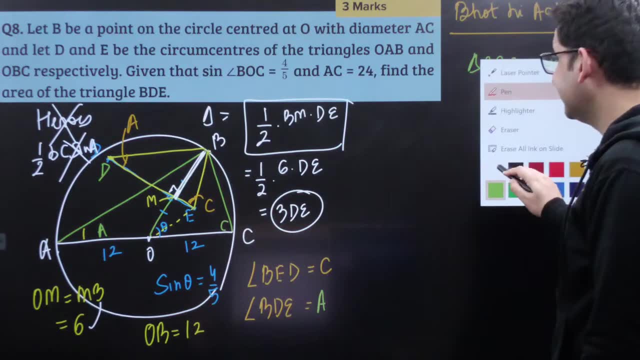 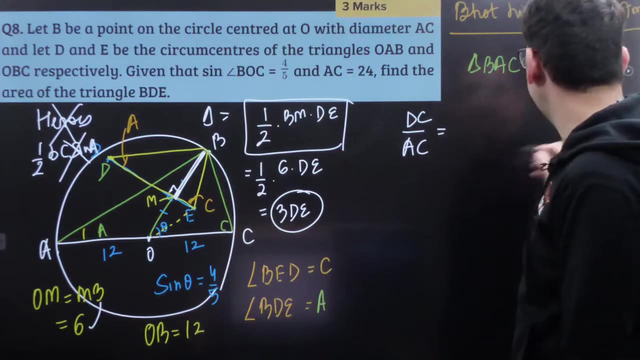 To kena say: these two triangles are similar to each other. So agar ye do triangle similar hai, guys, Agar ye do triangle similar hai, So kena say, kena say DC upon AC is equal to DC. Sorry, not DC DE, DE upon. 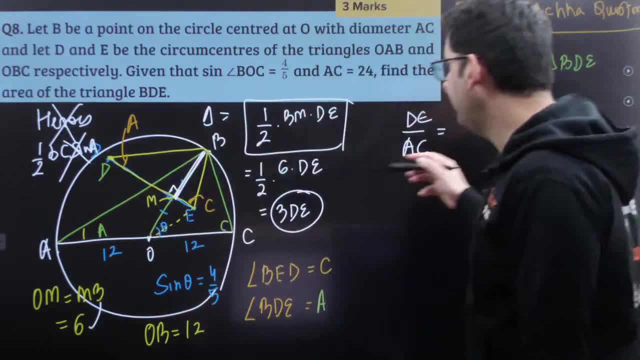 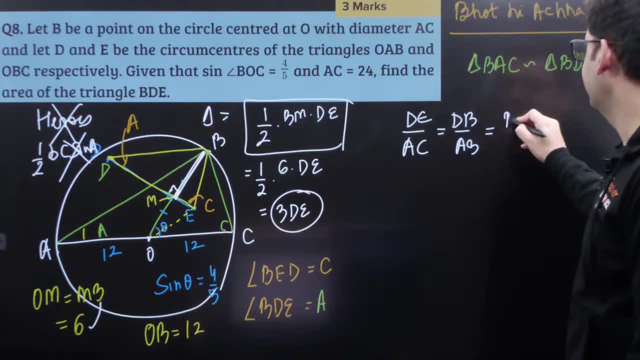 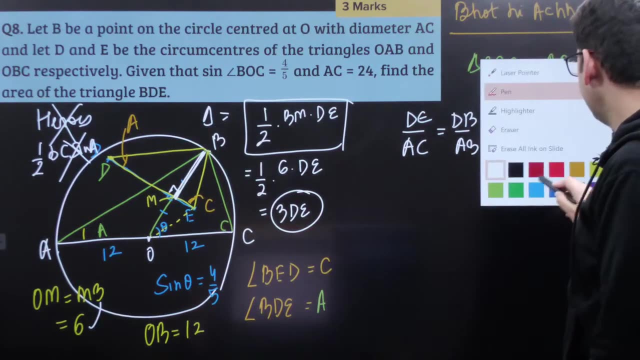 AC is equal to DB upon AB. DB upon AB is equal to BE upon BC. Ye cheez ho ka Acha. mujhe DE nikalna hai. I need to find DE Acha mere paas AC bhi hai. I have. 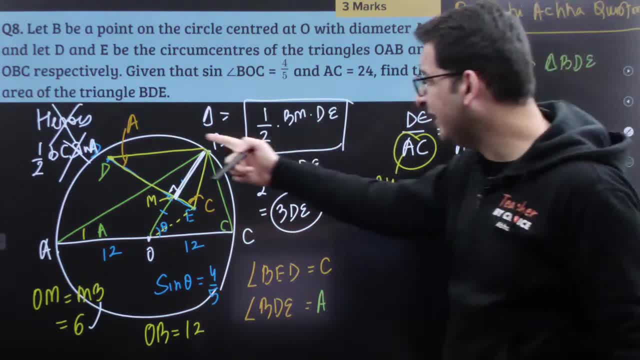 AC, which is 24.. But yaha par mujhe dikh raha hai: ya, DB bhi nahi hai Aur AB bhi nahi hai. DB aur AB mein se kuch bhi nahi hai. Similarly, BC, BE bhi nahi hai aur BC bhi nahi hai. In dono mein se kuch bhi nahi hai. 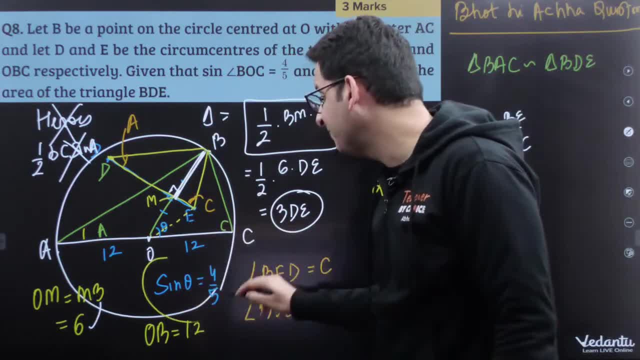 But mein paas abhi ye ye cheez hai, ki sine theta is 4 by 5.. Iska istimal abhi tak maine nahi kiya: Sine theta 4 by 5.. Sine theta 4 by 5.. Ab guys, yaha par dekho. 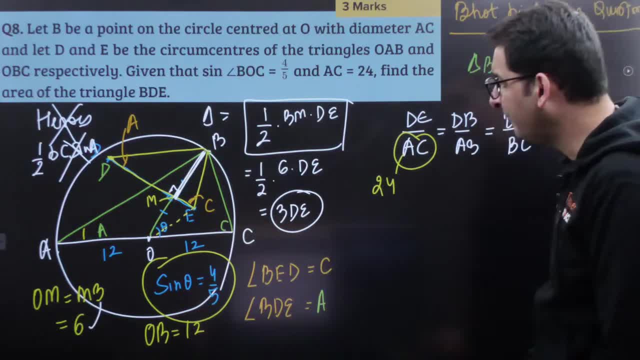 ek bahut interesting ki Sine theta 4 by 5 ka sabse bharpoor fayda kese hoga, Agar main yaha se perpendicular drop karta ho. Let's say, this is N Drop a perpendicular from B. 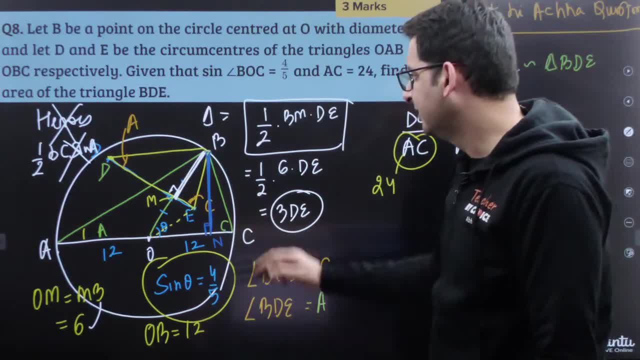 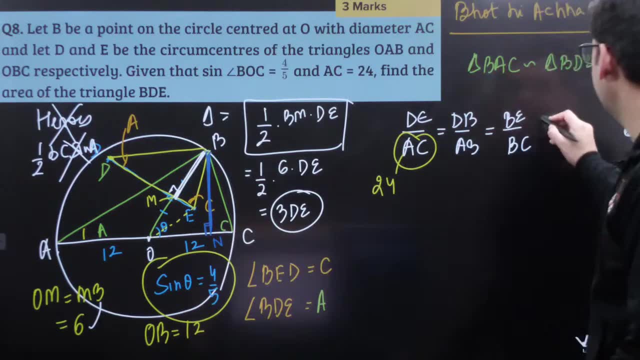 to AC. This is N, This is N, This is M. So can I say, agar ye triangles similar hai to inke, perpendicular, ka ratio bhi similar hoga. So this will be equal to BM upon BN. also, Can I say that: 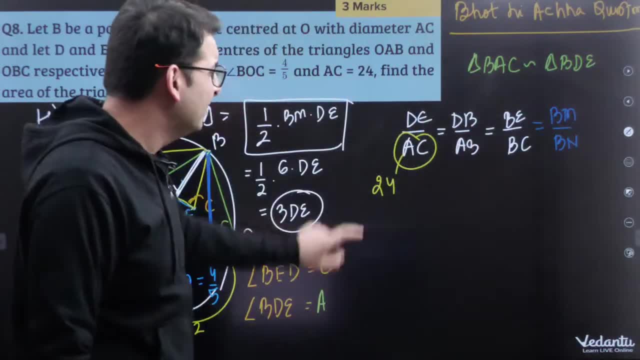 Agar ye 2 triangles similar hai to sides ka ratio to barabar hoga. Mujhe ye nikalna hai. Problem is, mujhe ye find karna. Ye hai Yaha to ye dono pata lag jai, Yaha, ye dono pata lag jai. 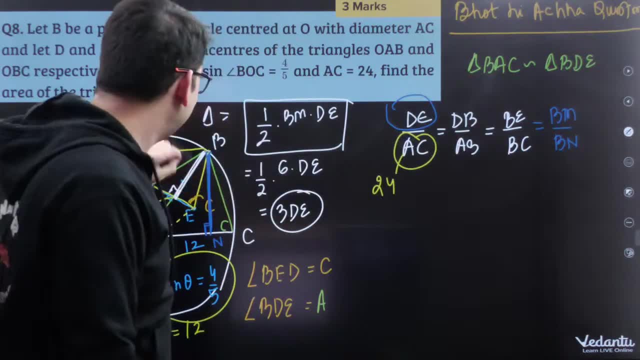 Ye dono pata nahi lag raha hai. Na ye, na ye To maine. kya lagaya ki BM ka value to already hai. maine pass Maine B se N bhi drop kar diya. Perpendicular on to BAC, So similar triangles. 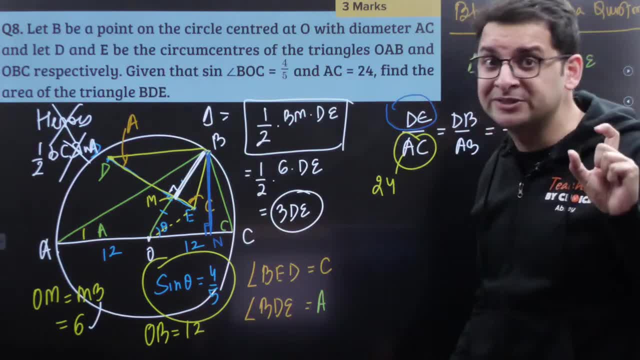 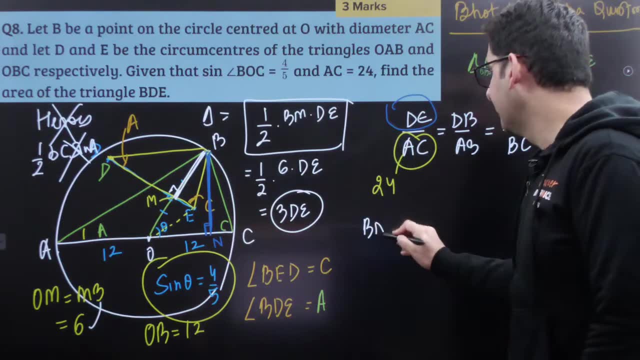 agar hai to length of the perpendicular, Ratio of the perpendicular is also going to be same. So can I say: BN ka value, Agar hum dekhe What is going to be BN, What is going to be BN, So ye OB. 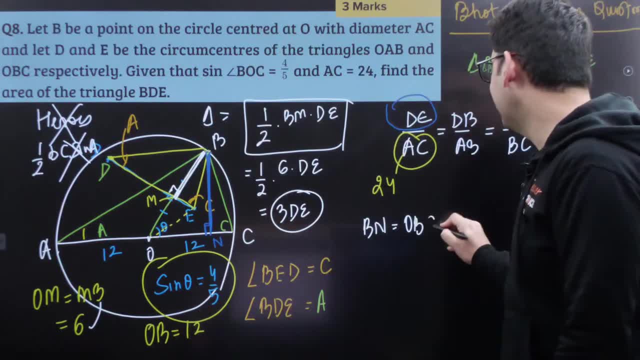 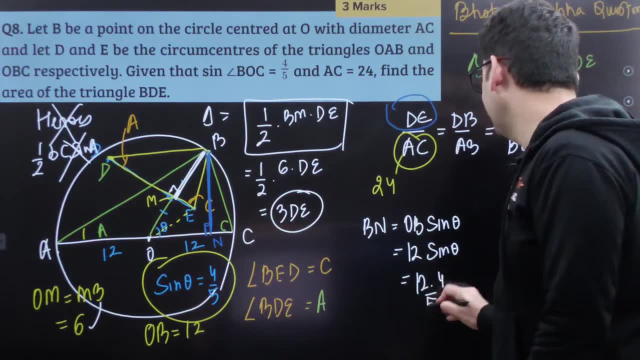 OB ka sine theta, OB ka sine theta, OB ka sine theta. matlab 12 sine theta. Matlab ki 12 into 4 by 5.. Matlab ki 48 by 5.. Ho gaya question. Ho gaya question. So DE upon 24. 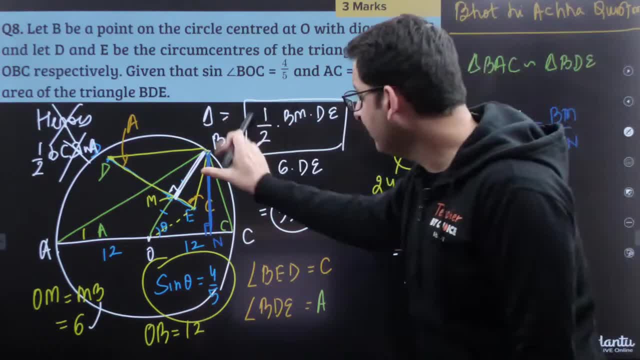 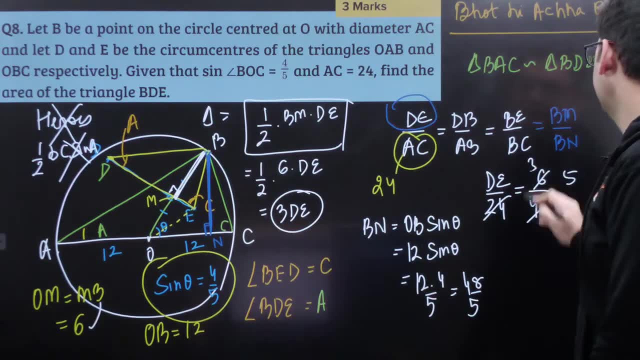 is equal to BM. What is BM? BM? BM is 6 upon 48 upon 5.. Ye ho gaya 2.. Ye ho gaya 3.. So DE ka value agaya 15.. DE ka value 15 hai. So 3DE is going to be 45.. 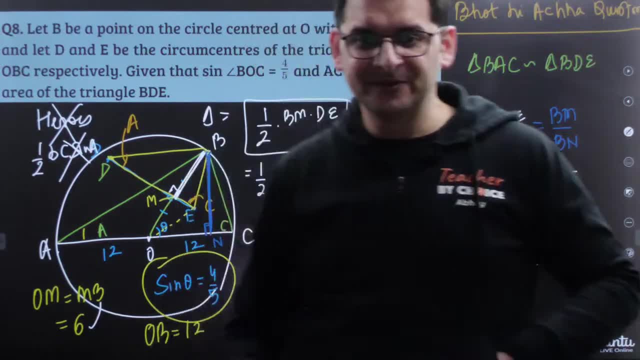 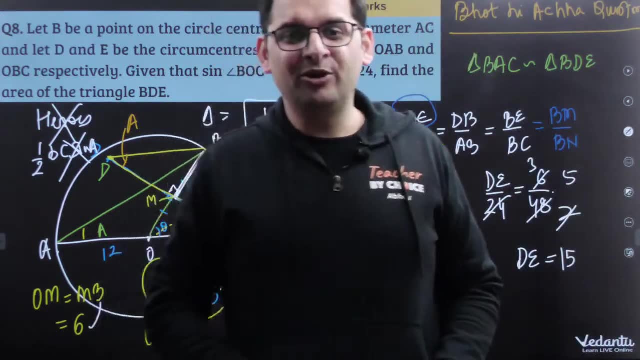 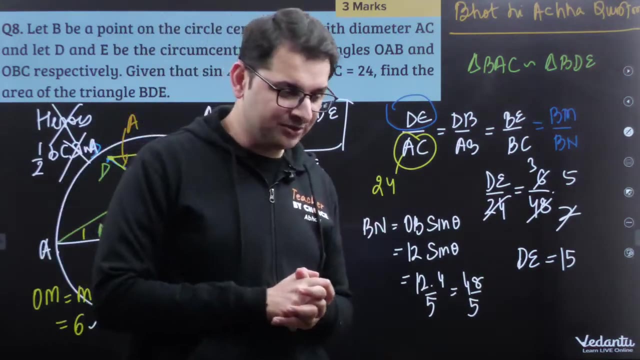 So 45 is going to be the right answer. 45 is going to be the right answer. Is this clear? Is this clear? Oh na, bhai, If you are a part of IOCUM camp, elite camp, agar ke tum part ho to 19 or. 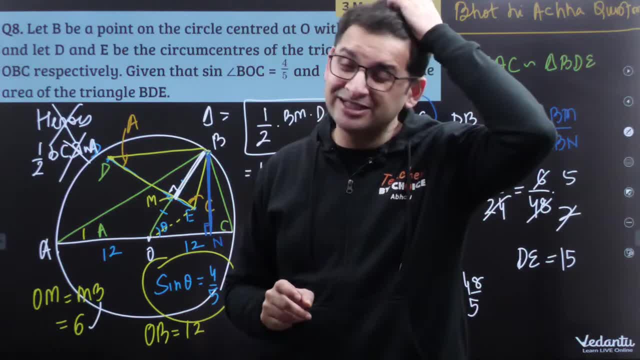 20 ko tum check karna, 18 or 19 or 19 or 20 ko humne 2 lectures, 4 lectures liye the Tika hai. 3 marker geometry, 5 marker geometry. 3 marker number theory, 5 marker number theory. Wo amazing. 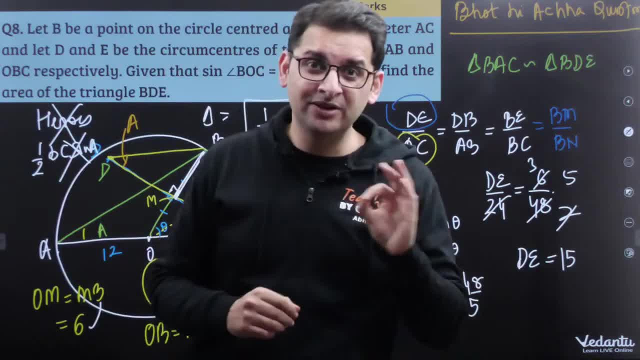 question: the 3 marker b, 5 marker b. To usme jo 5 marker wale question tha hai, jo humne geometry me aur number theory me kara tha, wo actually me 5 marker hota hai. Ab wo alag baat hai. 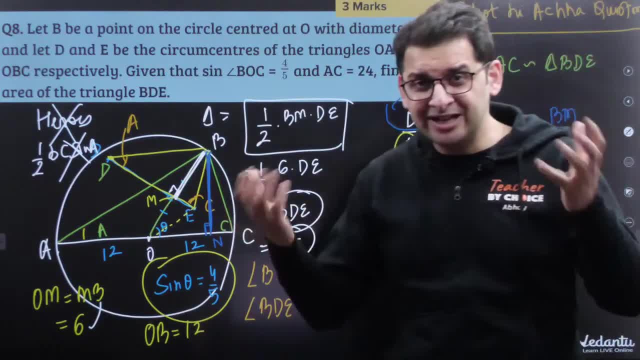 ki kabhi kabhi IOCUM ki andar bhi 5 number wale questions itse jata hai, Jo simple hota hai, Ya 3 number ke questions aise aata hai, jo muskil hota hai 5 number me. 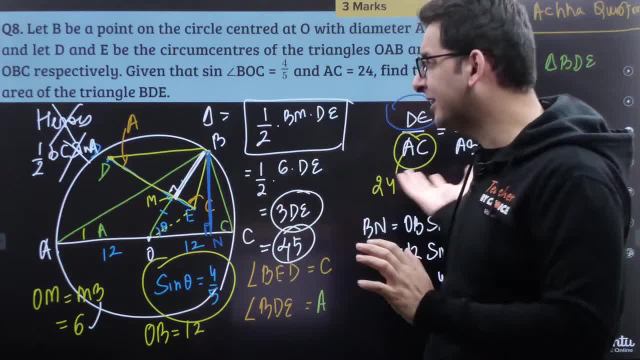 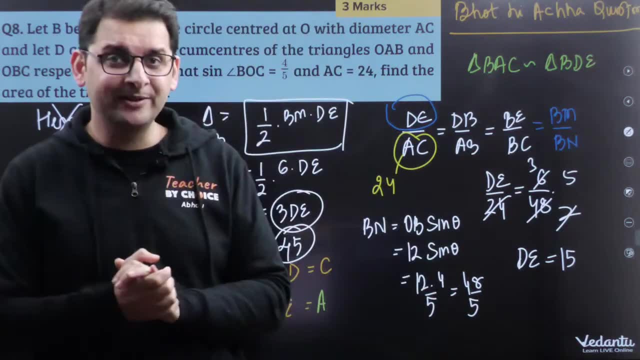 hota hai. So it happens all the time. But actually me ye zyada muskil question hi hai: 5 markers ke anda bhaut zyada cheezan sochni padti hai, Bhaut alag thought lagta hai, Isme zyada thought nahi hai. 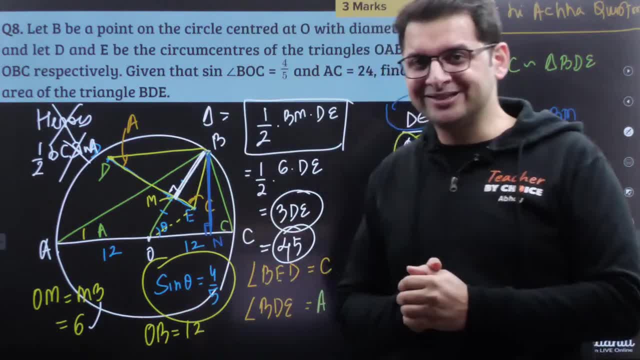 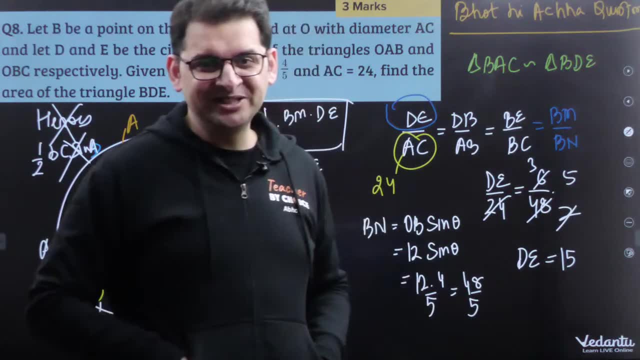 Bhaut simple hai, isme Basic concept hai. Did you all get this? Did you all enjoy this? Samajh me hai Maza ya Maza zyada important hai. Did you all enjoy this? Did you all enjoy this? 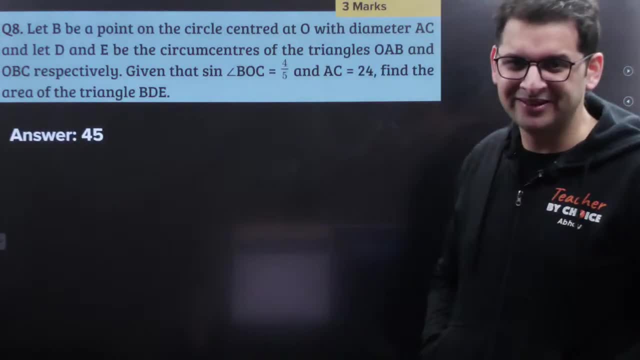 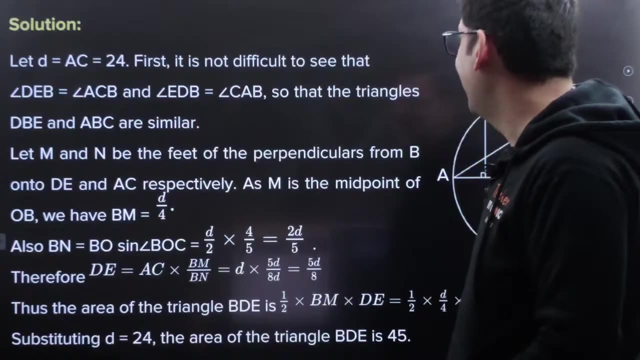 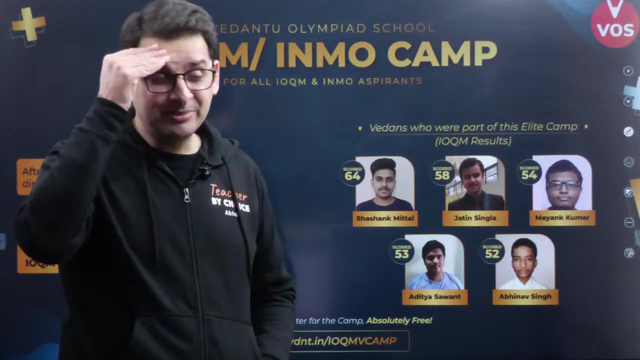 Yes, Superb, Superb, Superb, Exactly, Akshit, Exactly. I hope this is clear, guys. So that is it, guys. Aaj bhaut is chota session, Bhaut is cute session. Jase ki maine starting me bola tha Bhaut sare. 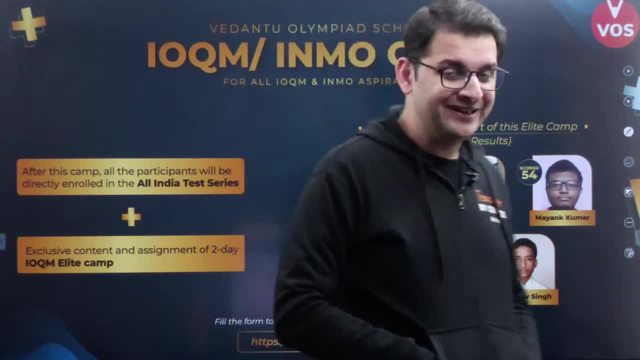 bachche unse gila shikwa kar rahe. the Yaha pe telegram pe ki sir aap INMO ke liye zyada karwaate ja rahe ho, IOCUM ke liye kuch bhi nahi karwa rahe. So I 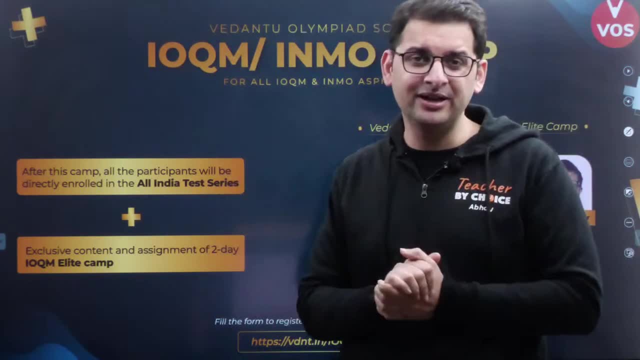 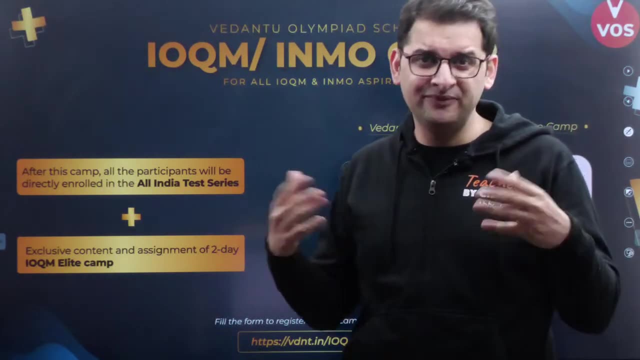 thought iss hafte hum 2 markers, 3 marker 5, marker ke questions ke upar topic wise pe focus karenge To aaj ka session was on geometry. Kal ka session maybe will be on number theory Ek session, algebra pe Ek session hum. 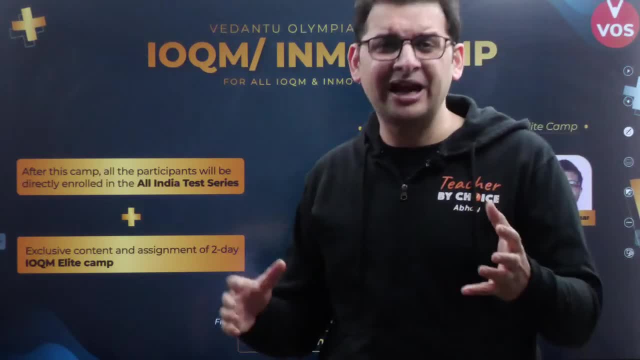 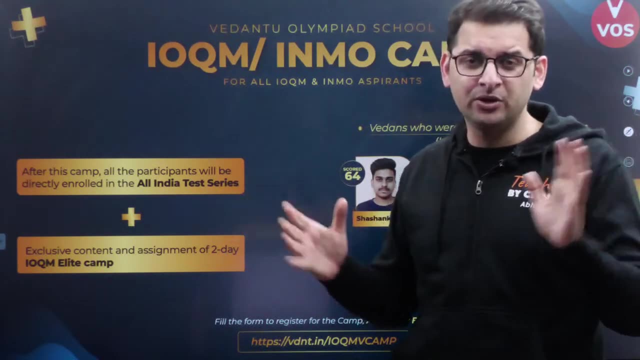 combi pe lenge Jisme hum 2, marker 3, number Aaj majorly 2 number ke questions, the But kal 3, number 5, number wale questions hongi Tike To basically IOCUM. So this week we are going to concentrate. 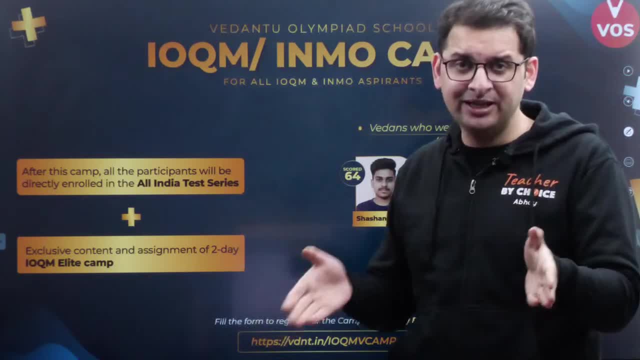 on IOCUM, INMO walo ke liye camp hai. Aaj mera lecture hai. INMO ka hi lecture hai 6.30 baje Jisme, functional equations and numbers discuss karna hai, And secondly INMO question of the day. 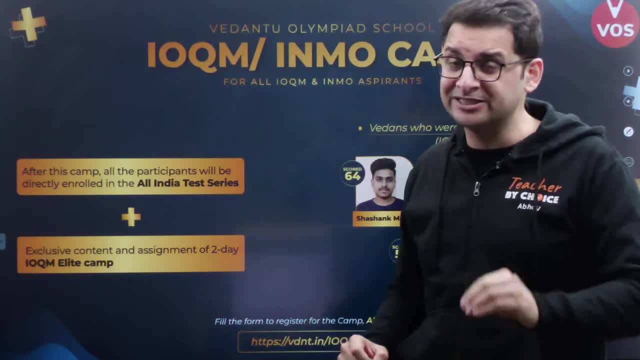 aar roz Ek question tum logon ke liye, INMO walo ke liye already aa raha hai, Jiske andar tumhe dekhna hai, Baht amazing ideas hota hai, Wo sochne hai Samajhne. 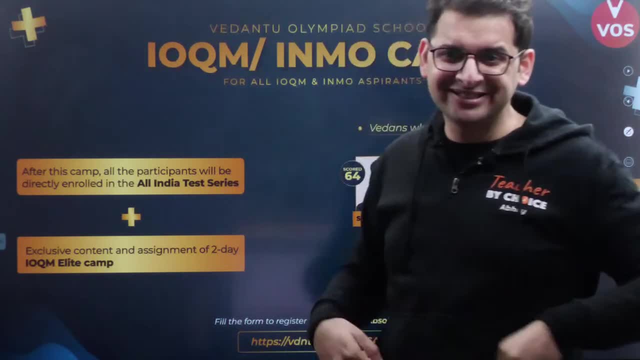 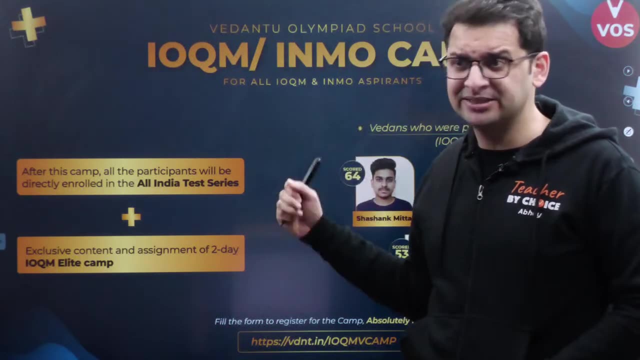 hai, Aapne dimaag mein dalne hai And feel lene hai: Yes, Superb, Yes, yes, yes, bache, every, every day, we are going to discuss one topic, Aaj geometry, kiya discuss Kal number theory karenge. 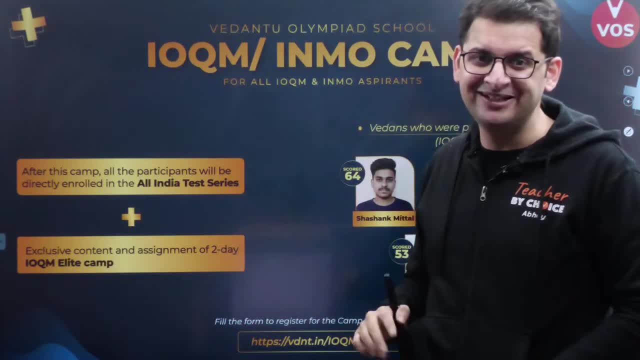 Phir algebra karenge, Phir combi karenge. Toh main chodunga nahi, bhai. Simple thi baat hai. I will not leave you Telegram ID, guys. ye note, karlo, You can always get into. 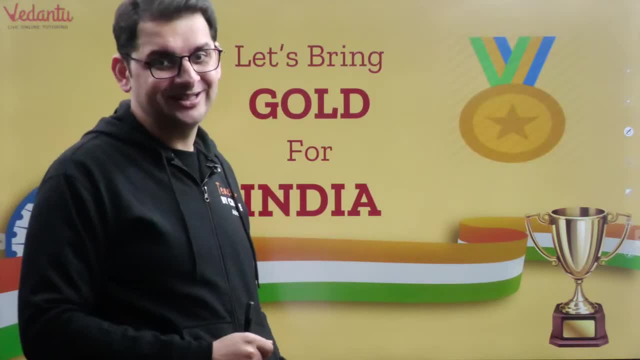 touch with me over telegram, And this is the aim. Isko dhyan rakhna, guys, Iss saal nahi Agle saal pakka se karenge, But iss saal koshish, karenge, Puri, Puri koshish. 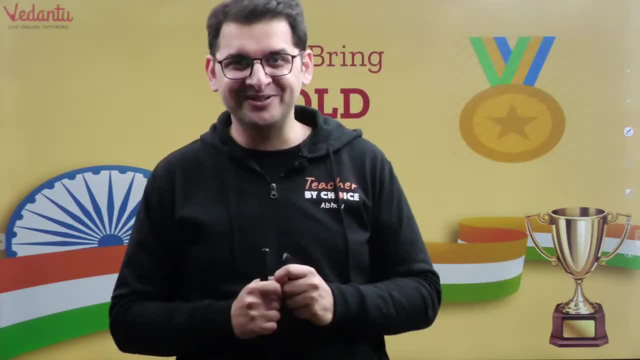 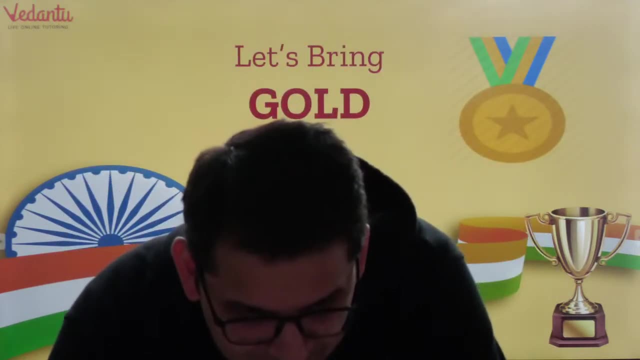 karenge, Shiddat se koshish karenge, Koshish karne walo ki kabhi haar nahi hoti. All right guys, Take care. God bless you. I'll see you in the session. Bye everyone.